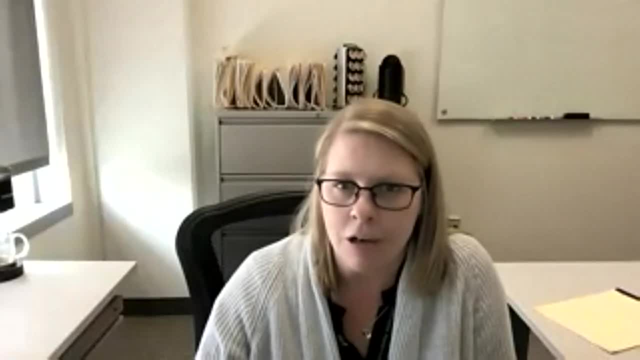 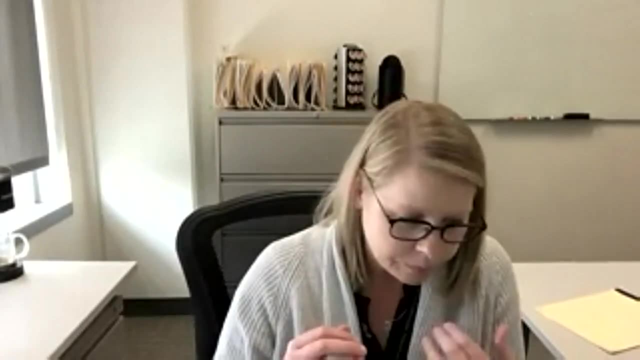 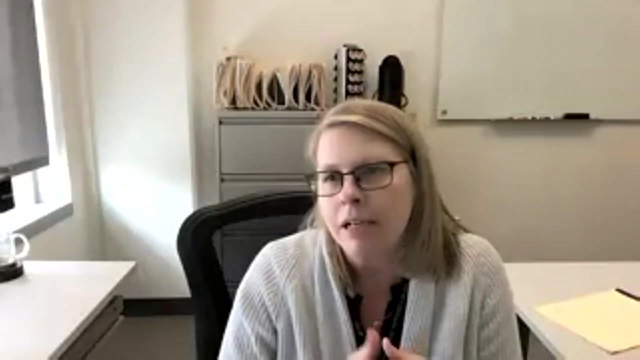 be accessed through our website, which is called OPAR. Maybe I can get Rob or Shannuk to write our website in the chat for me. A few housekeeping things before I hand it over to Rob to do introductions. First of all, you're automatically muted when you come. 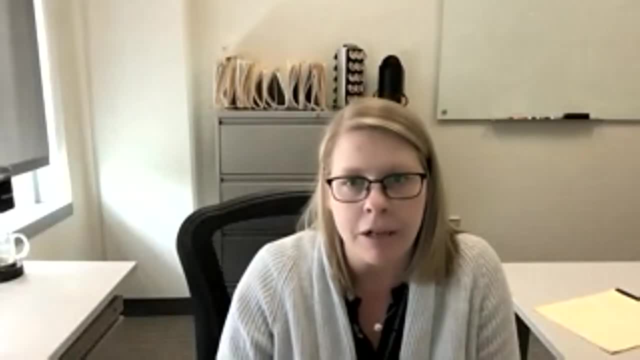 in. We appreciate it just because of the number of people on the call. If you stay during the webinar, you'll be able to hear from us. So if you have any questions, you're muted during the presentation and write your questions in the chat. Shannuk's. 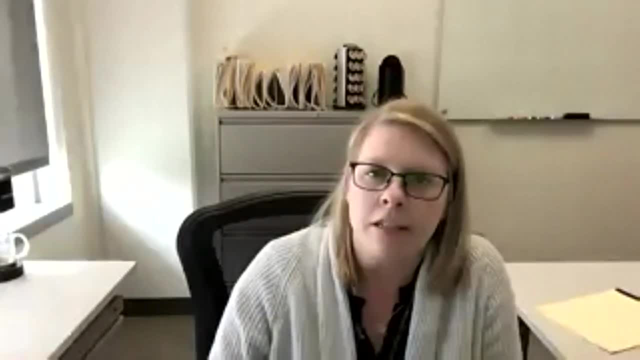 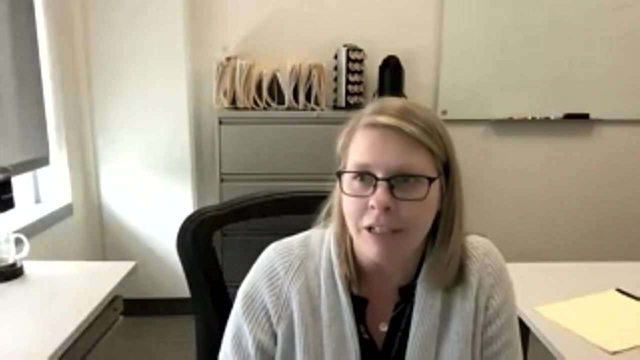 going to be watching and monitoring that chat for us, And so when he sees questions that warrant clarification right at the moment, he'll go ahead and speak up. If there are more discussion-related questions, we have designed this webinar to be, in general, an 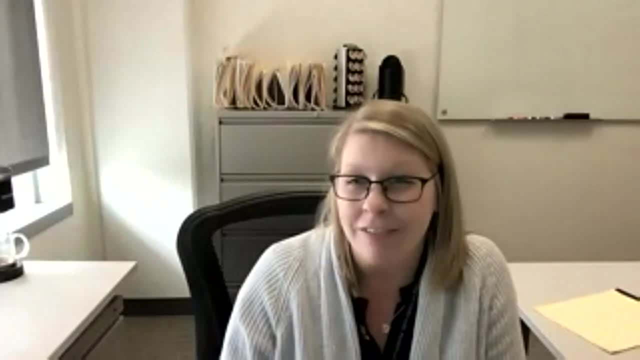 hour of presentations, then followed by 30 minutes of discussion for those that can stay online. It usually takes us about an hour to get to the end of the webinar, So if you have questions, please feel free to reach out to Rob. We'd love to hear from you. 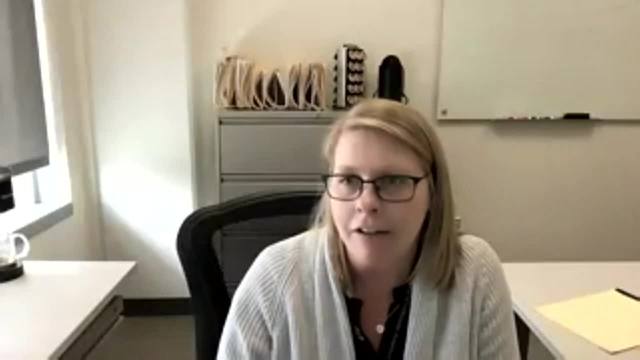 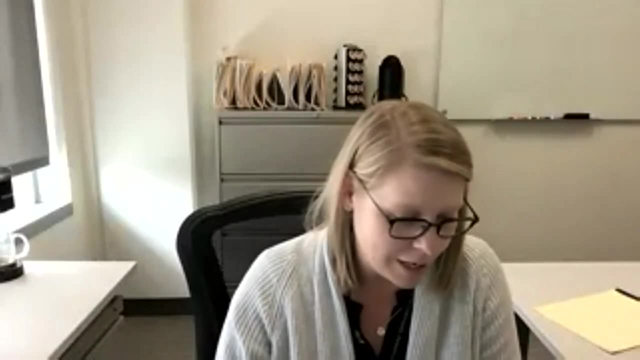 So we've got about a little less than a week to get the video up on the website and all the appropriate links there after it is. So if you have to leave early or if you want to share it with a colleague, we will put this recording up on YouTube as well, I think. 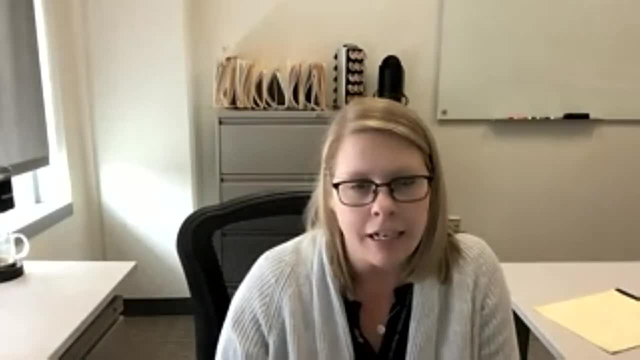 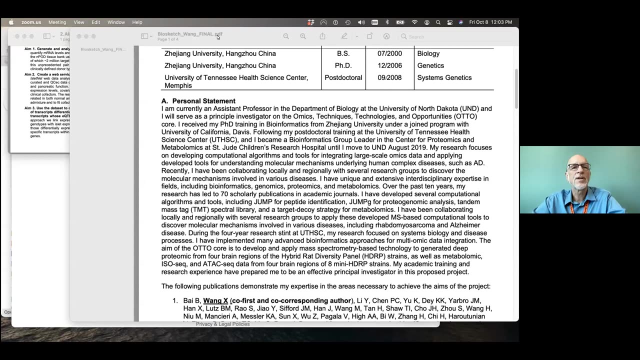 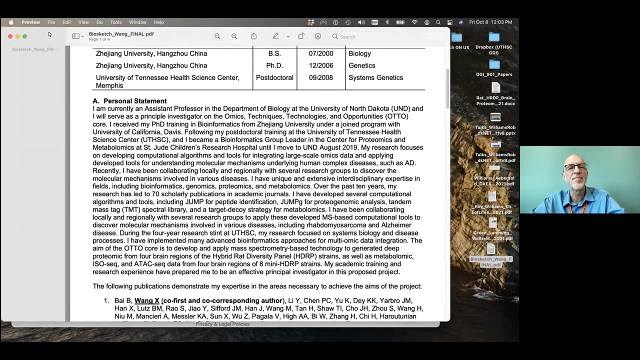 that takes care of the housekeeping things. I'll go ahead and hand it over to Rob to introduce Shuxing. Yeah, it's a great pleasure to have Shuxing join us to give a presentation. He's been at our OPAR webinars. 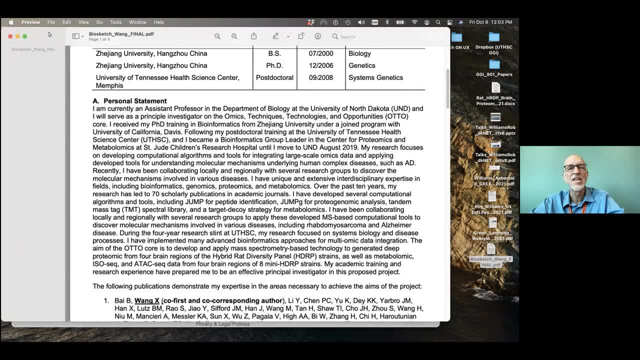 And great Xu Sheng. thanks for agreeing to do this. Xu Sheng was also a recipient of a pilot grant from the OPAR P30, and it went so well that he's taken on a larger role in our pending renewal. But I just thought of an efficient way. 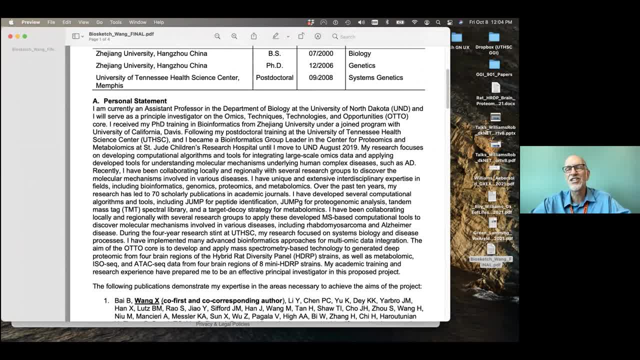 to do an introduction and not make too many boo-boos is actually to show you his personal, his biosketch. And he started out in Zhejiang, on the east coast of China, just a little bit south of, well, probably a couple hours south of Shanghai. 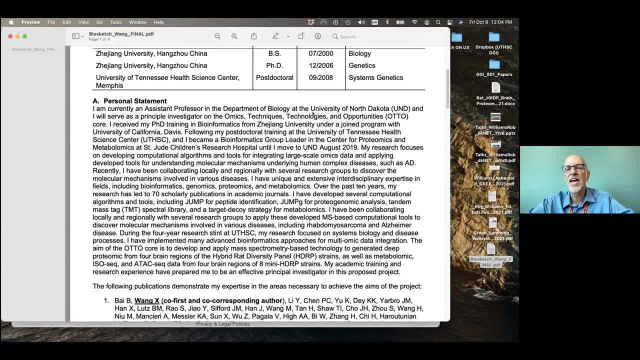 It was sort of a unique university that had a joint PhD with the University of California Davis, where I got my PhD, And so he has always had. since I've met him, he's always had excellent English, which is wonderful. He's a really strong bioinformaticist. 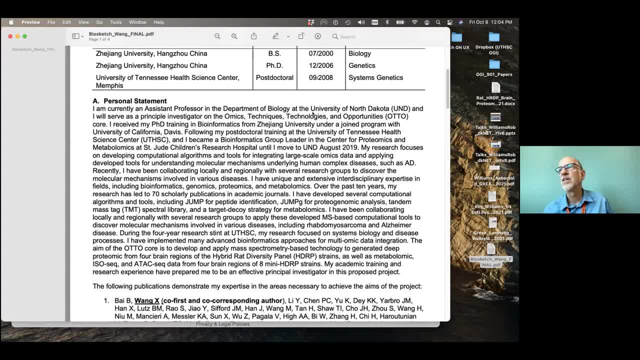 Zhejiang is famous for its bioinformatics and genetics- statistical genetics programs, So he came. when he came to UT in 2008,, he really was more than a postdoc, He was actually responsible almost single-handedly- Poor Zhejiang. 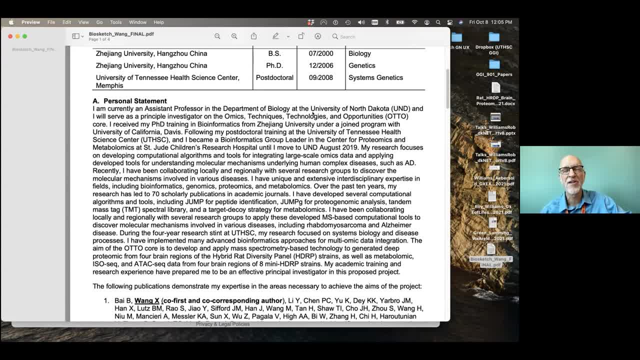 For all of the genomics and bioinformatics we did on campus. So he was sort of a one-man band for many of us And he stayed at UT, came out with a really high impact set of papers with Dr Lulu and myself and others, Megan. 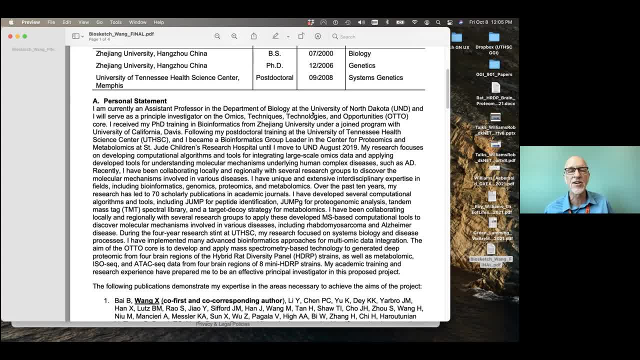 I don't know how many others really very productive stay here and then moved down the street to St Jude where he worked for the first time very intensely in proteomics with Junming Peng, who is a famous proteomics expert at 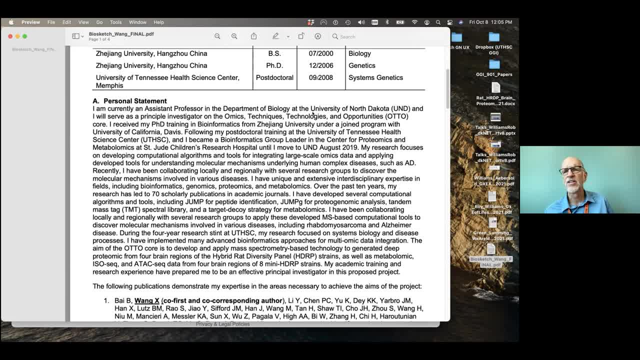 who was at Emory and now at St Jude, And I think Junming. even if I'm correct, Zhejiang did a lot of work with Geigy at Harvard at some point. So Zhejiang really pushed the envelope on proteomic workflows and software development. 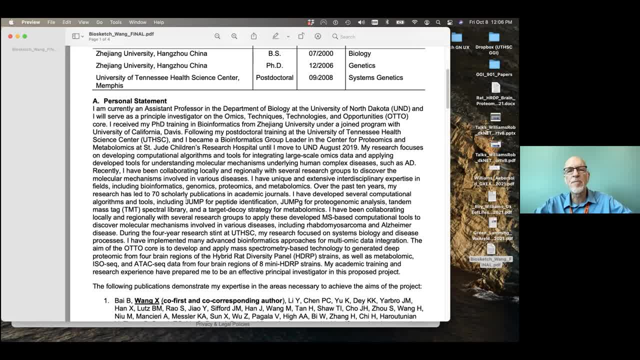 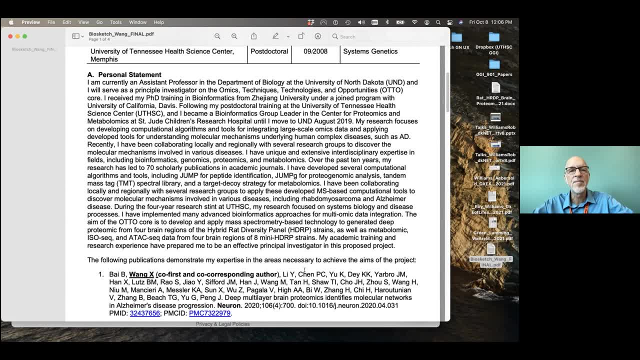 And he this whole jump series that you see here: jump for peptide identification pump, jump G for proteomics. that's all work that he's done. So in addition to doing the analysis, he also builds the tool sets that are critical for proteomics. 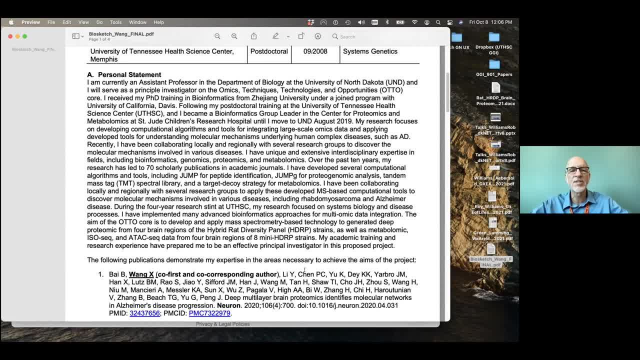 So I really we couldn't have had a better expert to give us this talk. The nice, the great thing from my point of view is he's he's worked with the hybrid rat diversity, the hybrid hybrid data set, And he's been on this panel and we will. 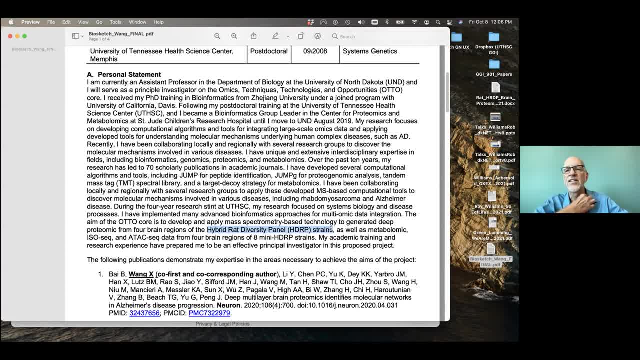 he'll be telling you a little bit about that data set towards the end of his presentation. Then I'll be giving you a short tour of the data that Zhejiang and team generated and then I'll hand it back to Zhejiang. 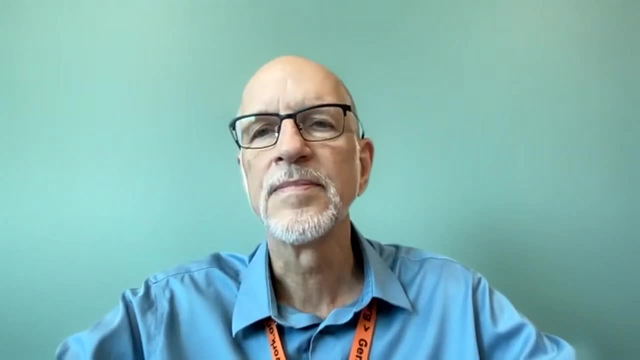 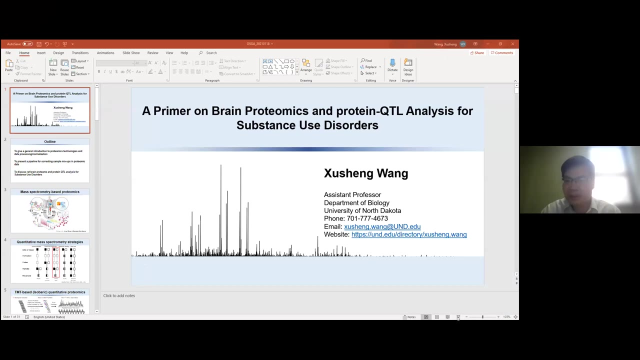 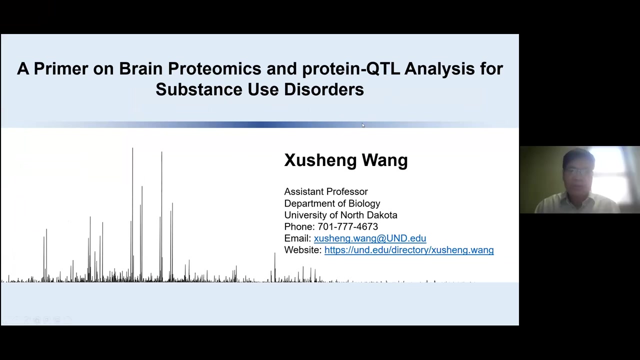 So thanks very much, Zhejiang, for joining us. Thank you very much, Low, for your nice introduction. Yes, but it's not yet in presenter mode. Okay, There you go. Perfect. Yeah, So today, I think Rob and I are going to present proteomics and protein QTR analysis. 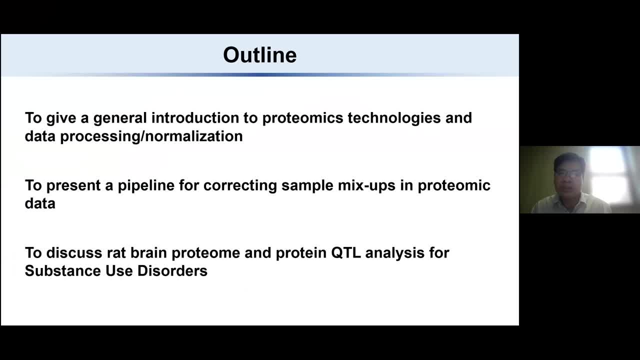 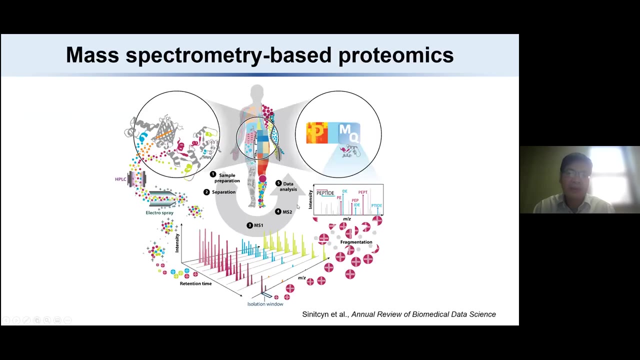 We will first give you a general introduction to proteomics technology and data analysis, And then we will present a new pipeline that we developed for collecting sample mix-up in proteome data. And finally we will discuss red brain proteome and protein QTR. 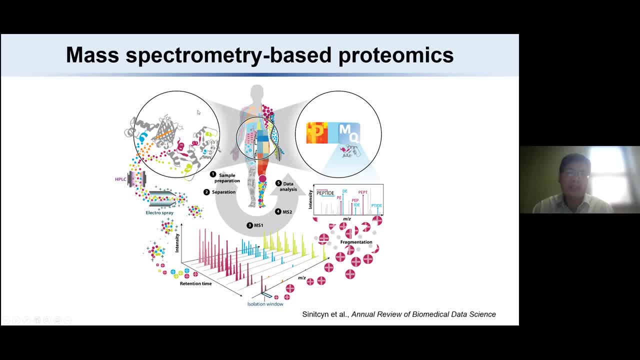 So, first of all, what actually is mass spec-based proteomics And for a typical mass spec-based proteomics workflow And a protein analysis, Proteins are first extracted from the biological samples And in some of these experiments you want to enrich, you know, organelles or cell type. 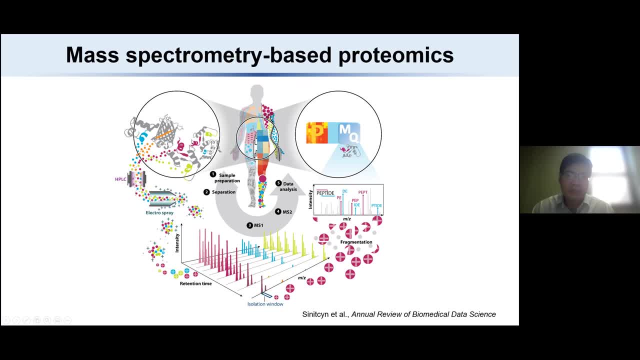 But it is optional, And protein are first extracted from the biological sample, Then it's digested into the peptide with enzyme such as trypsin and the mix-up peptide, then separated by HPLC, And the peptides are ionised and injected to the high-resolution mass spec. 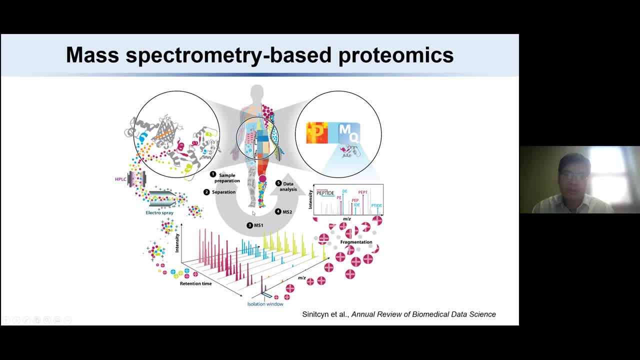 And what you will get is two types of information. One is MS 1 spectrum And then MS 2 spectrum. So MS 1 spectrum contains all the information about the mass and intensity of the protein. Okay, peptide and MS2 spectrum contain the mass. 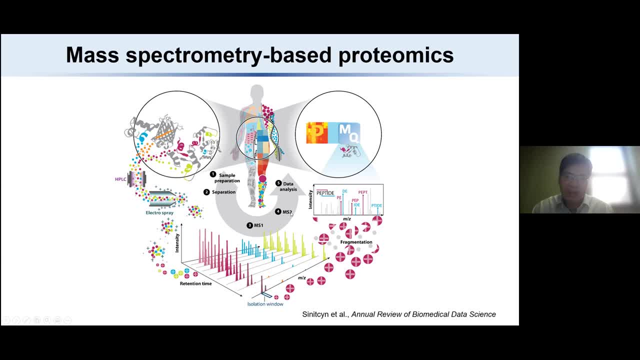 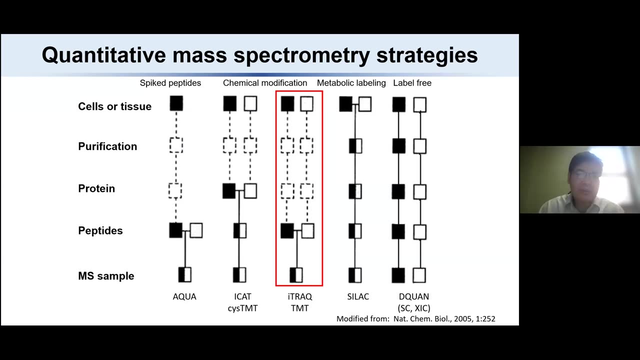 and the intensity of peptide fragments. And just for the last step of the proteomics is the data analysis. So I will introduce the data analysis later on. And so there are several approach for quantifying peptide and proteins, And so this approach can be divided into absolute. 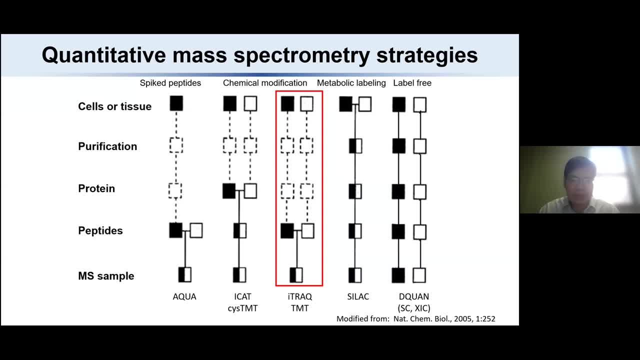 and relative quantification. In absolute quantification we want to determine the copy number or concentration of the protein within a sample, Whereas in relative quantification a ratio or relative change of protein concentration between sample is a measured and a calculated. So both absolutely and relative quantification. 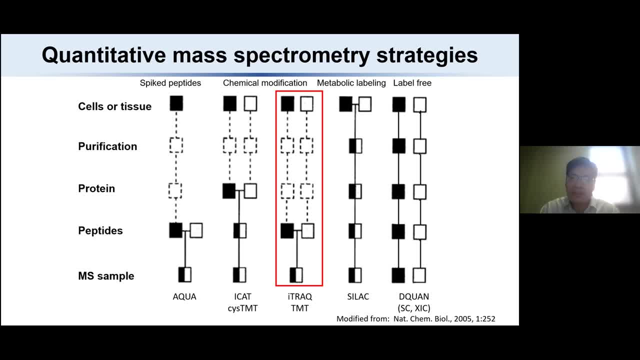 can be done with either label-free approach or labeling approach. So, for label-free approach, a bigger challenge for label-free approach is batch effect and the data normalization. And so, as you can see, this is the data normalization approach. And so, as you can see, 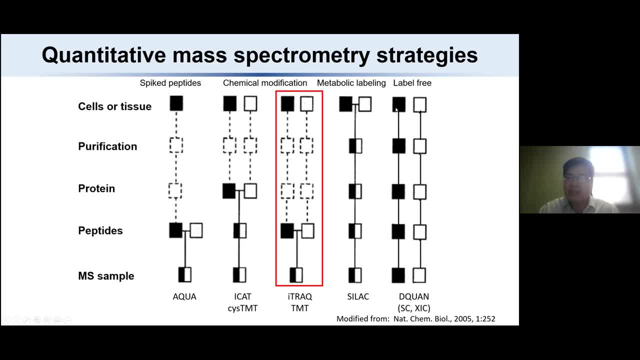 And so, as you can see, this is the data normalization approach, And so, as you can see, each sample is analyzed by LC-MS independently. each sample is analyzed by LC-MS independently from the example preparation to data acquisition, So it suffers a big variation between sample to sample. 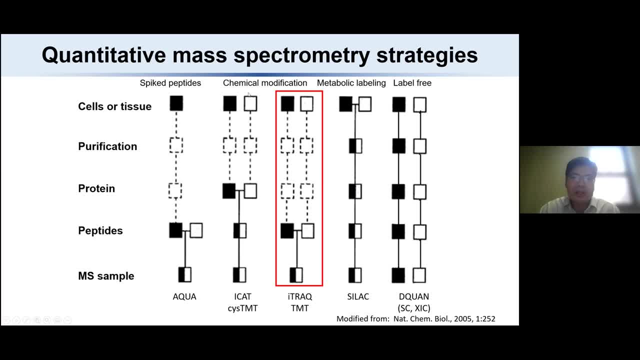 And so for labeling approach, there are chemical labeling approach and the metabolic labeling approach. So metabolic labeling, typically the master labels arginine or lysine with stable isotopic And it's labeled on the protein. So this approach is the most accurate. 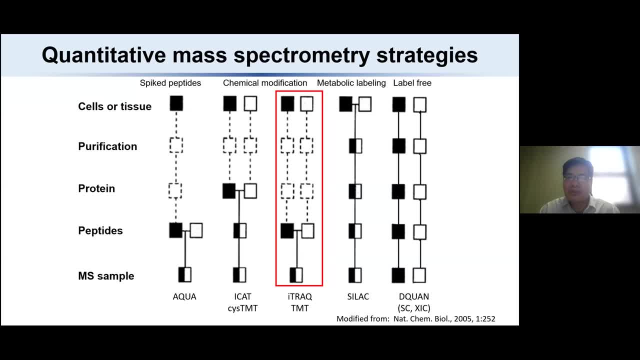 But the downside for this approach is they cannot multiplex many, many samples, For example the Silek approach. For example, the Silek approach only measured up to three samples for one experiment And for the isoponic labeling. 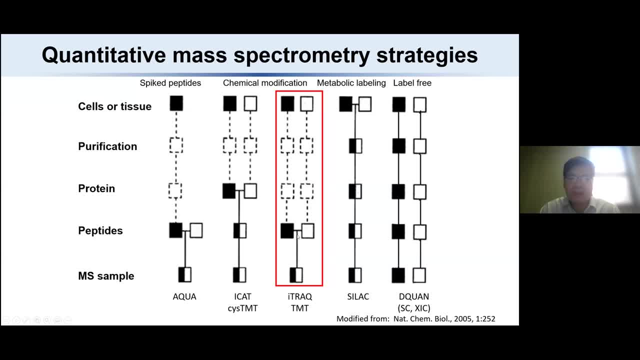 and it can be labeled at protein level or labeled at peptide level. But the good thing for this approach is you can measure 18, and right now up to 18 samples at the same time, And this is a big advantage compared to the other approach. 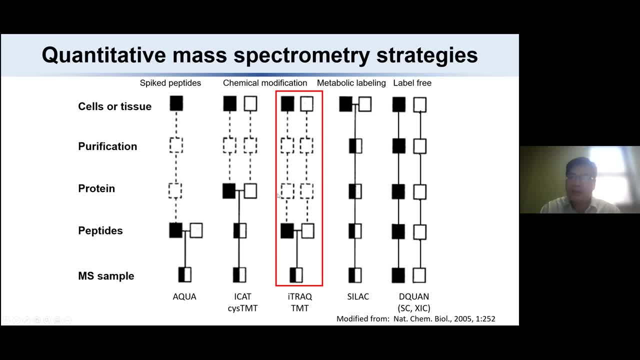 And. but the downside of this approach is the ratio suppression because of cool eluting peptides. So for some of the spiking peptide you can spiking the peptide into the sample, you can measure the absolute composition, And so the most widely used chemical labeling approach. 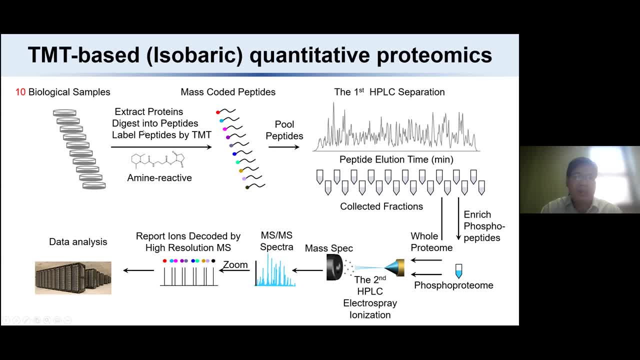 is a TMT based approach And, as I said, we can label 18 sample right now, but here I just take a 10 sample, 10 TMT, a 10-plex TMT experiment as example. And, for example, you have a 10 biological sample. 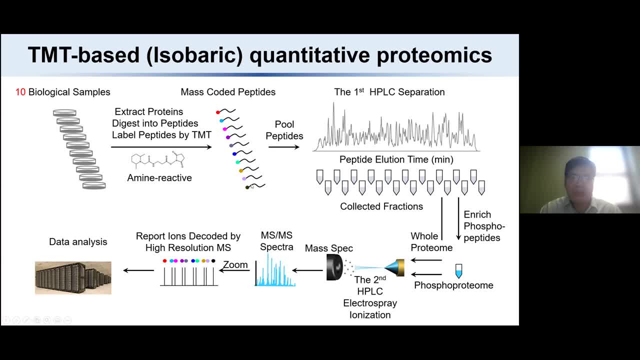 and it digests into peptide, then you can label the peptide with a TMT reagent And after that you can mix all this peptides and apply it to the sample And across all the samples and then you separate the sample or the peptide. 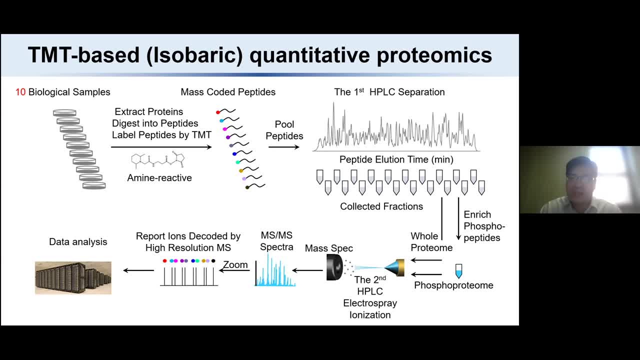 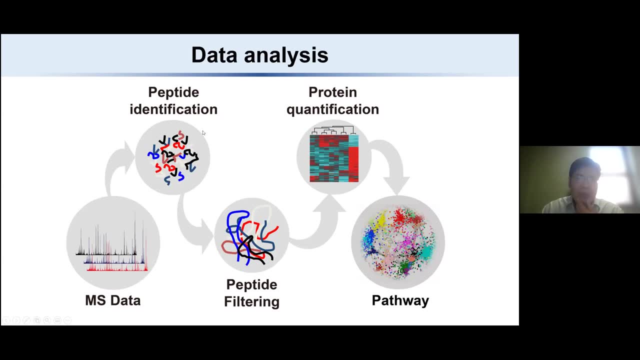 into different fractions using HPLC, And then you can take one fractions and inject to the mass spec and get the data in. So for data analysis, and there I think there are four major step involved in proteomics data analysis, including peptide identification. 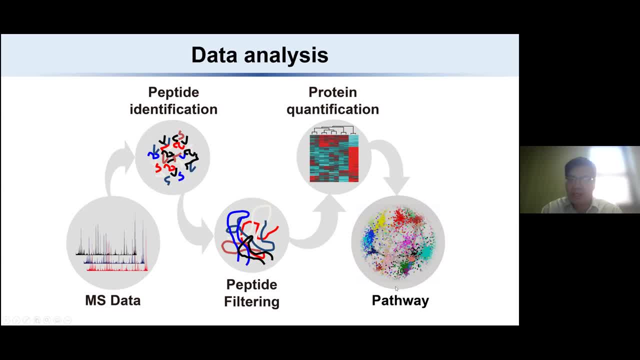 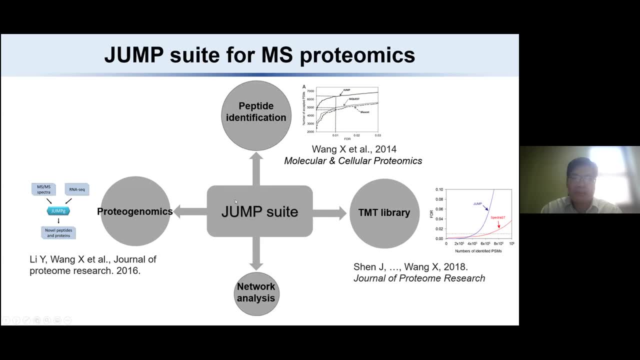 peptide filtering and protein quantification, as well as a pathway analysis. As Rob mentioned, we actually develop a nice comprehensive pipeline called the JUMP Suite and which includes peptide identification and for for the JUMP, we actually able to search. 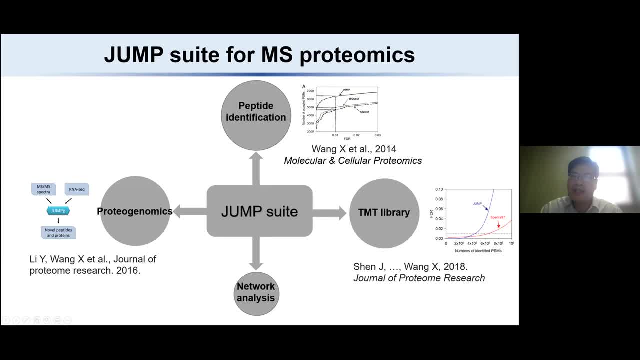 identify more- 20% more ID than two widely used approach like the Sequest and the Mascot, And to further increase the identification rate. and we developed this TMT Spectrum Library, which also allow us to increase 20% ID rate. 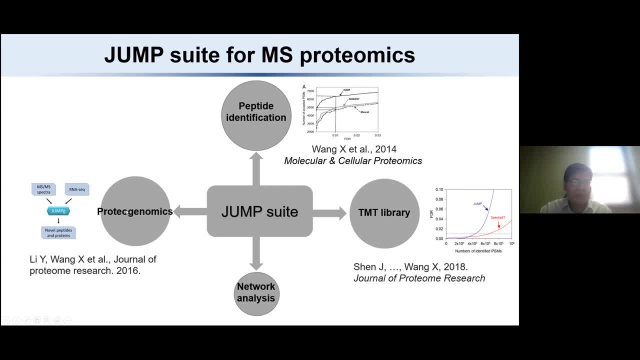 And we also develop, you know, JUMP-G for the genomics of pipeline, which is able to integrate genomics of transcription data and proteome data to identify novel peptide or variant of peptide, And recently we also published a tool called JUMP-N. 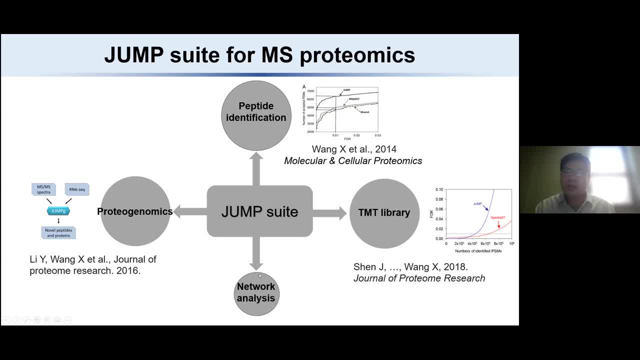 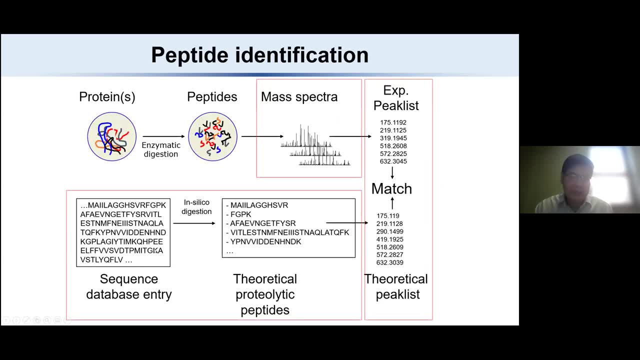 for you know, cool expression analysis. for proteome data, For database search, we first download protein sequence from public resource such as Uniprot and NCBI and NCGI or UCSC genome browser and then we can do incountable digestion. 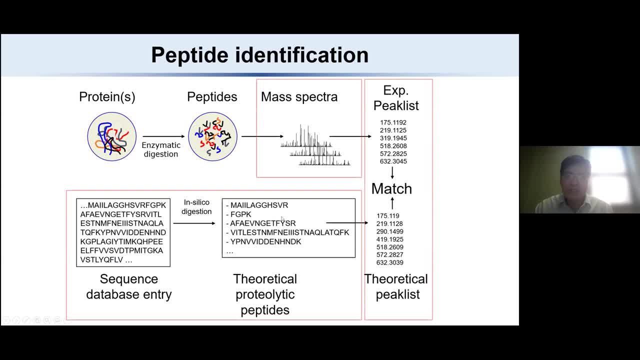 and to make all this peptides, And the search would typically calculate this theoretical mass for each, all these peptides that you might have this in silico peptide, And then for each spectrum we get from experiment, the search engine will calculate a matching score. 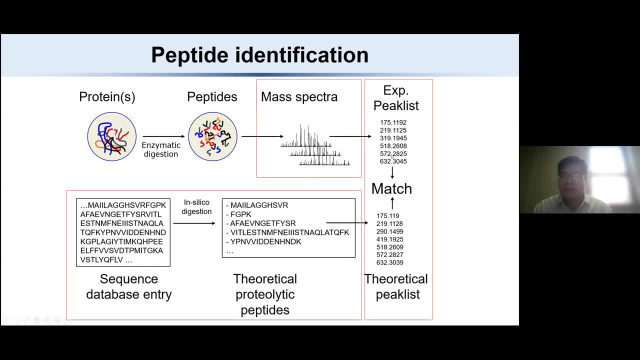 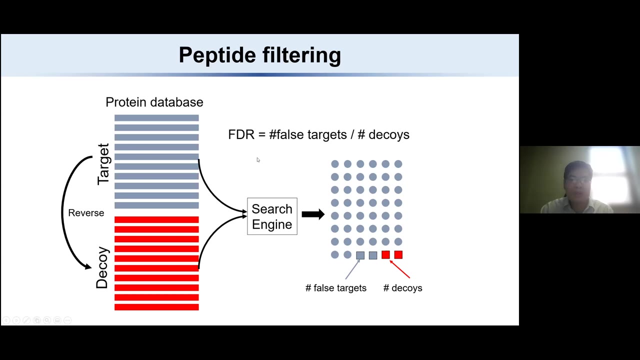 and basically match this measured mass against all the theoretical mass in the database And we will identify the best matching for a spectrum. And the best matching may not be the true quality, And so we typically control the FDR using the target decoy strategy. 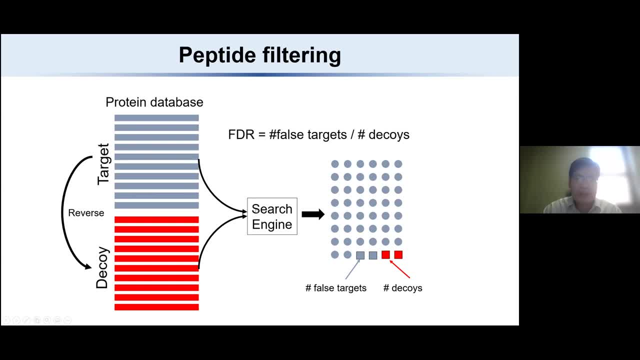 In the target decoy strategy spectrum are such against not only against this target database but also to decoy database, And at the end we will calculate the distribution of target peptide and the distribution of decoy peptide And then we define the FDR by a ratio of force target. 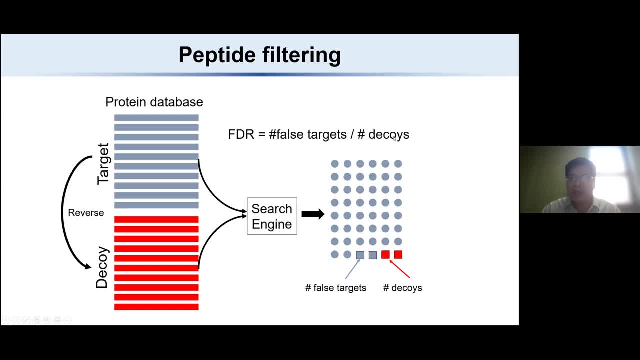 which is a decoy, the number of the decoy divided by target. Sorry, this is the target And to generate the FDR, we will use the FDR, which is the number of decoys divided by target, And then the decoy. we basically use the target sequence. 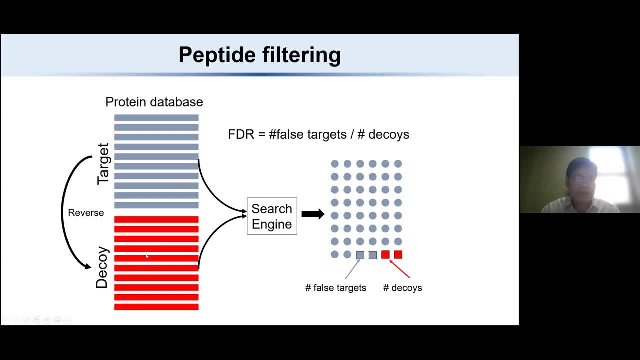 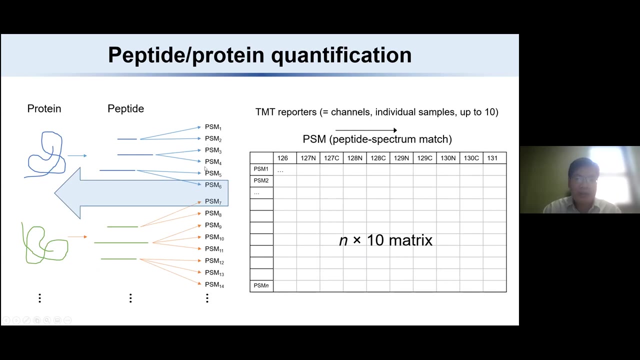 to reverse the sequence into the force protein sequence, then we do the digestion, And so this is a target decoy approach we use for FDR control. So, as I discussed and we actually what we measure is a PSM level, which means peptide, and the spectrum matching level. 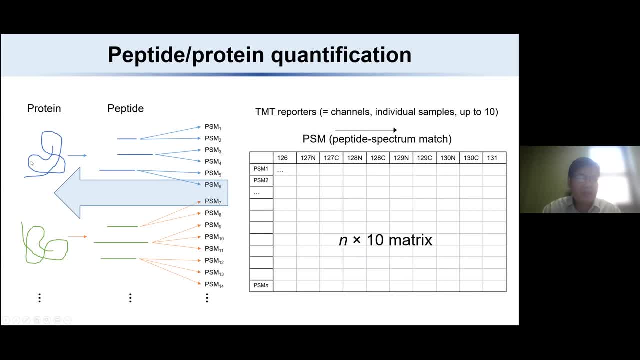 However, we are interested in the expression level at a protein level. So we need to summarize the protein, the expression level from PSM level to protein level. What do we typically? we first summarize the expression level at the peptide level first, and then we summarize the expression level at the protein. 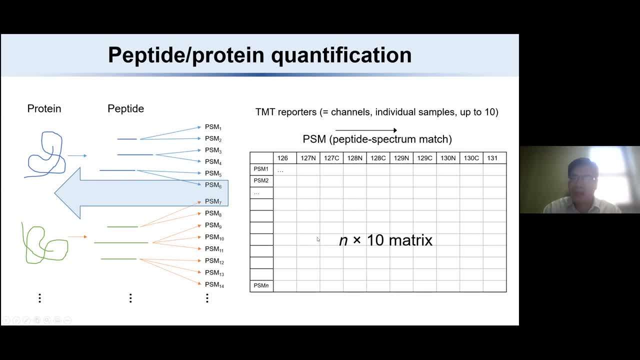 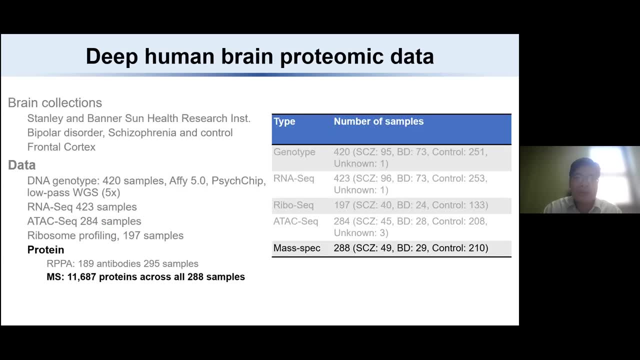 So at the end we typically have our three tables. One is PSM expression level and the peptide level and the protein level. So with this developed protein technology, we recently generated a human brain podium data And for this data we include 200 of the protein data. 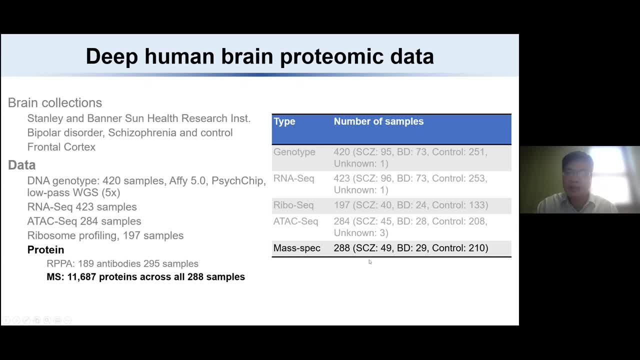 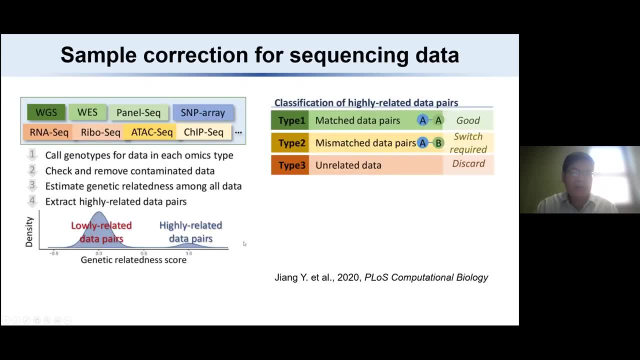 We included 10 normal control samples and 49 square linear sample and 29 bipolar samples. After we get to this sample, we realize this sample has a severe mix-up issues And our probably actually make this correction for other sequencing data such as riboseq and ataxic. 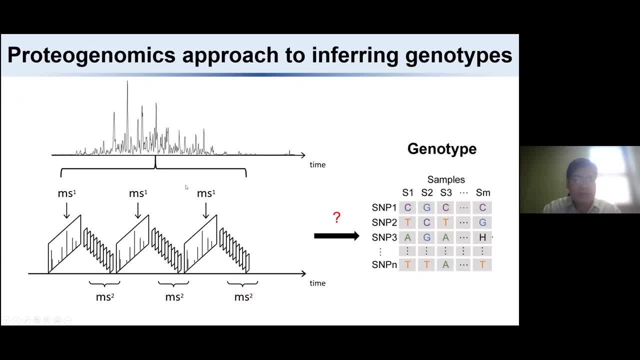 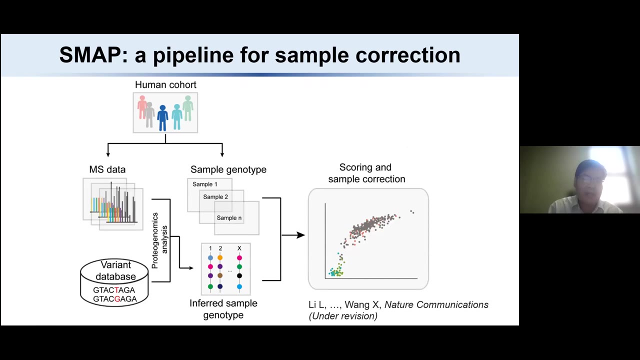 And, as I said, so proteomic data cannot provide those variant data or genotype, And what we got is all this spectrum, And then how can we get this genotype from this spectrum? So with that, we recently developed this SMAP pipeline for sample correction. 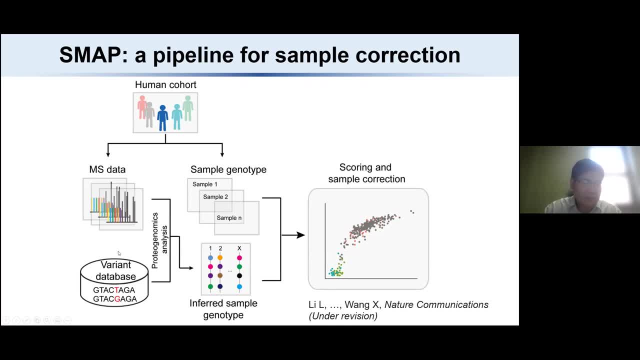 And SMAP actually contains three components. The first component is variant peptide identification using proteomic genomics approach, And the second step is inferring the genotype for each samples. And the last step, we just do the scoring and the verifying sample identities. 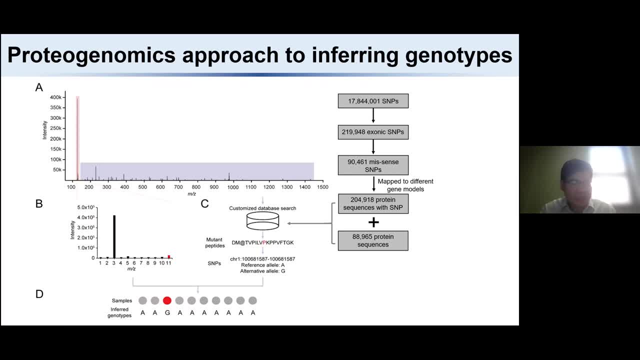 And to illustrate the idea of the SMAP, let me just give you this example. This is a typical spectrum from TMT-based proteomes, And so this is MS2 spectrum. On the left side, this peaks cause reporter ion and which is used to quantify the expression level. 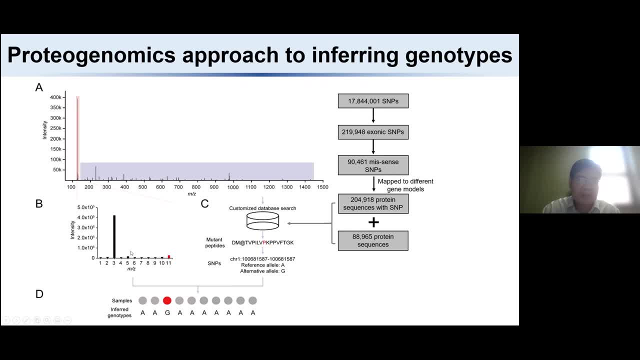 of the peptide across the samples in the samples And the peak on the right side is used for peptide identification. If you zoom in this one, zoom in this reporter ion, as you can see, the sample three has a high expression. 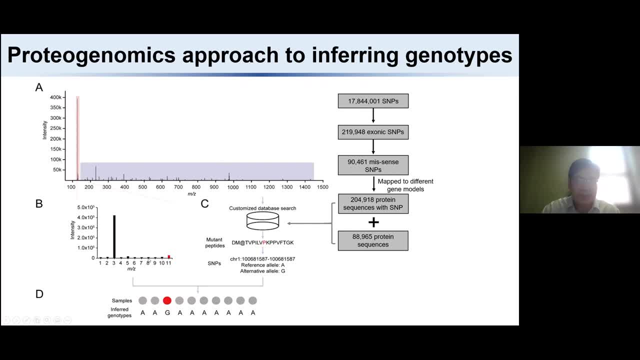 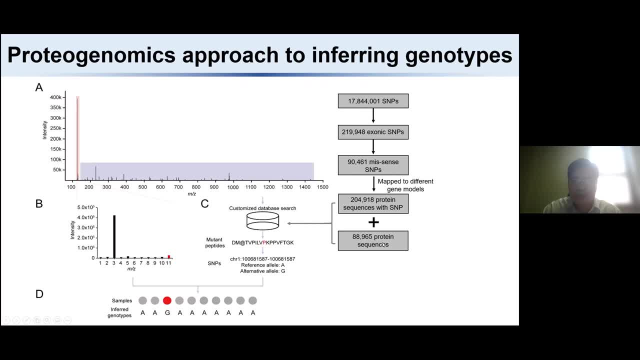 as well as all this connectic protein sequence And by searching the spectrum against this database, we can identify some variant peptide like this, And with this variant peptide we can get back to the allele information. So, for example, this is a reference, allele is A. 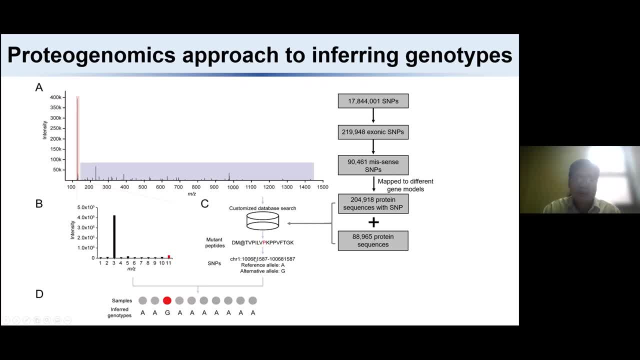 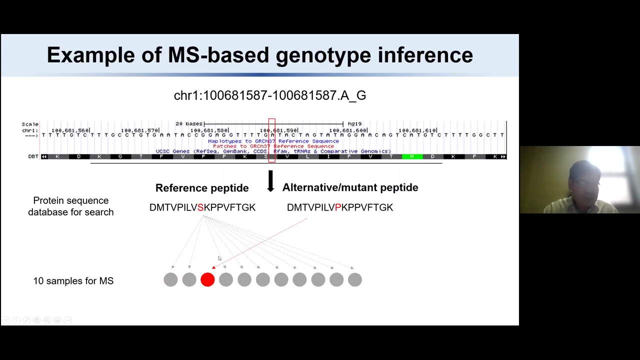 and an alternative allele is G. then, based on this expression data, we can say this: example three has this alternative alleles and all the other example has a reference alleles A, because this is a, this peptide is a variant peptide, peptide, and if this is still not clear to you, I probably 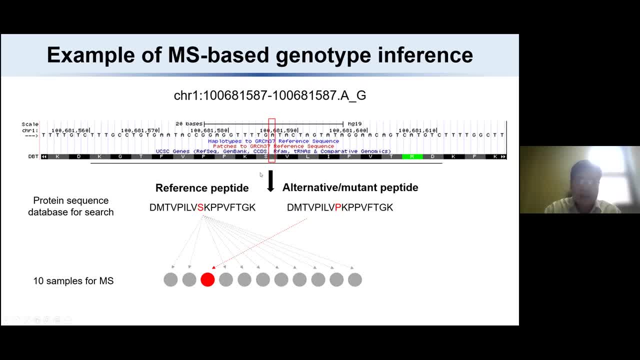 uh, we look. let's look at a more close about this example. so, for example, you have a SNP on chromosome one with this reference allele A and the mutant allele G, so the reference allele will generate this peptide- reference peptide- and this mutant allele will generate a mutant peptide. and 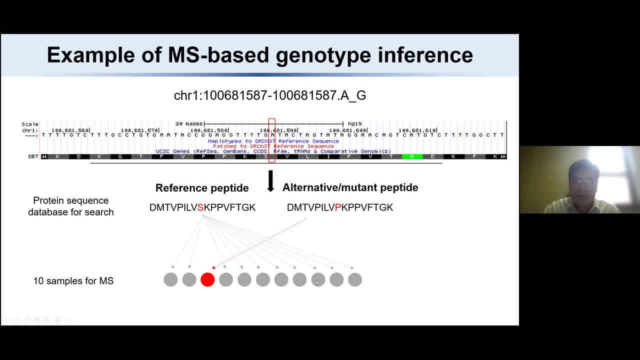 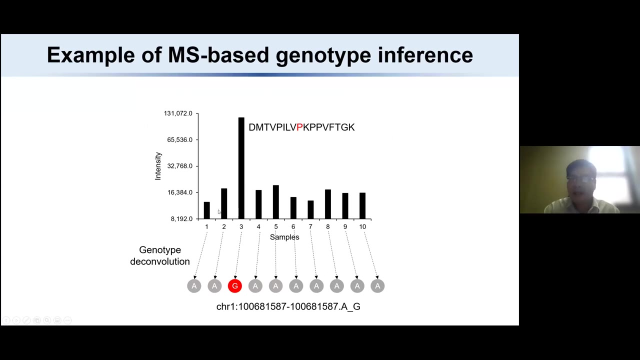 if you have a sample, uh 10 samples. so the example three has this mutant allele which will be observed, this variant peptide, because all the other example has this as a reference allele. we will not observe this reference, this mutant peptide. so if you look at the quantum data and you will see a highly 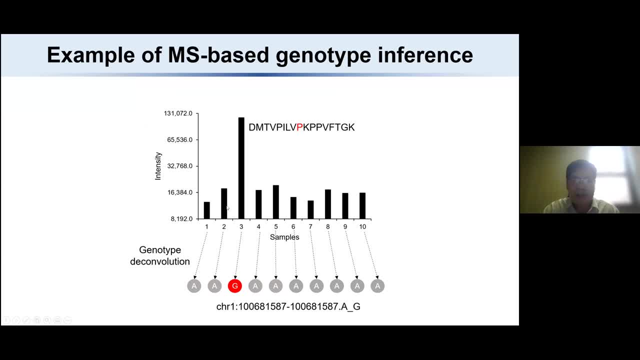 expression data in the sample three. uh, you have really low demonstration data for all the other examples. so ideally you should not able to observe any of these signals. but proteomes, you know, mass spec basically generous, a lot of noise, and so this is basically a noise level. 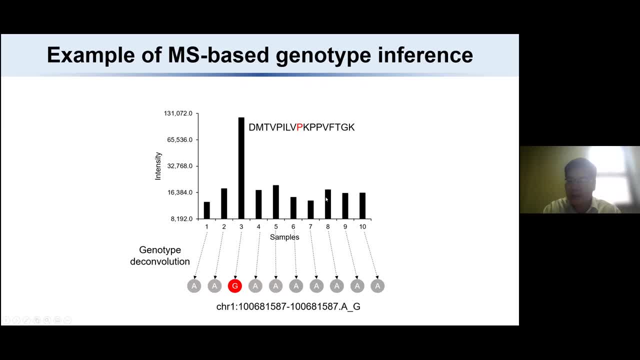 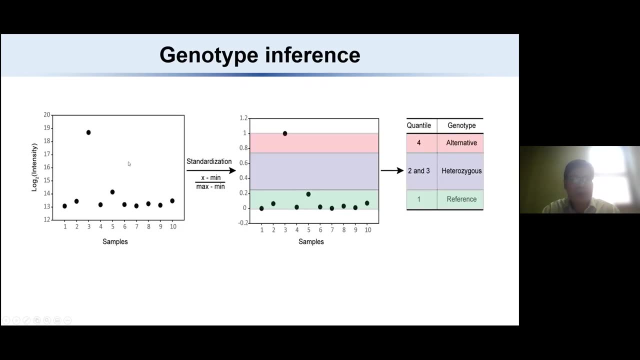 and which also makes this, our analysis, a little bit more complicated. yeah so, but overall you can. the example three has a mutant allele, but the other example has a reference allele. So again. so the peptide. when you measure the peptide, you typically will generate a very significant different magnitude of the abundance of different peptides. 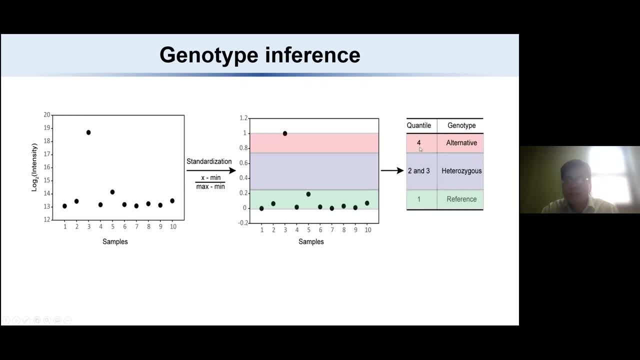 But in order to characterize this reference allele and mutant allele, we first standardize the expression level into a range of from zero to one, with the minimal signal as zero and the largest signal as one, And with this we classify the sample into three categories. and using this contour approach, and so the first one, 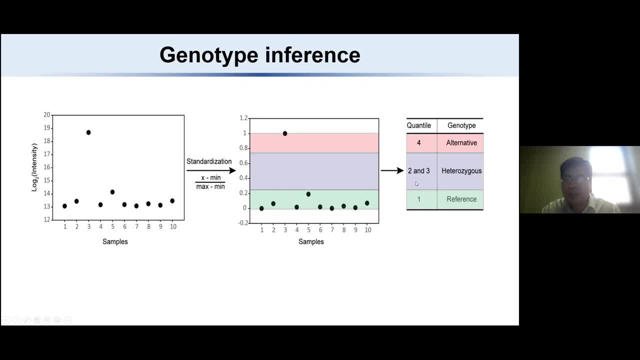 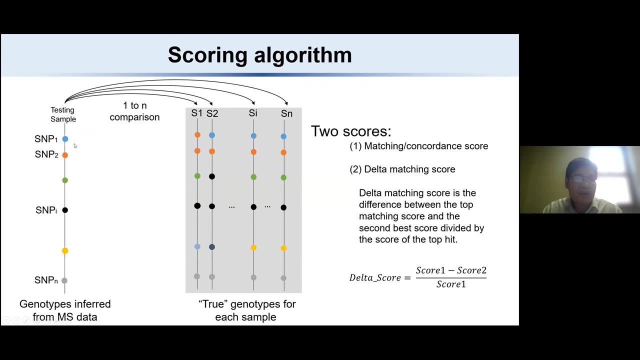 is for this first contour, which is a reference allele, And the above contour is the mutant allele and is the middle internal contour, which is the heterozygous allele. And so with that we can infer all the different number of different settings of the same frame. And in order to do this we need 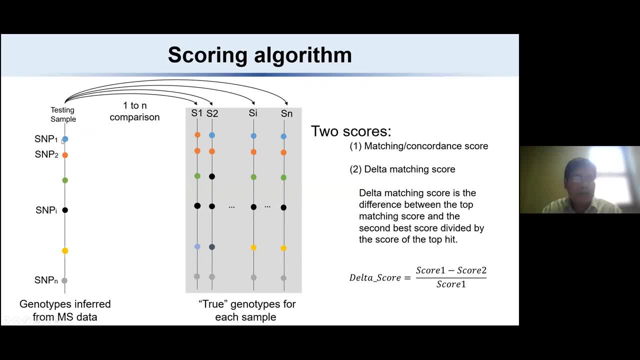 the entire range of the cytosine blend. So again we are looking for a close sort of complex leaf, all the SNPs for each examples, And then we compare these examples against all the genotype, the example in the genotype data. 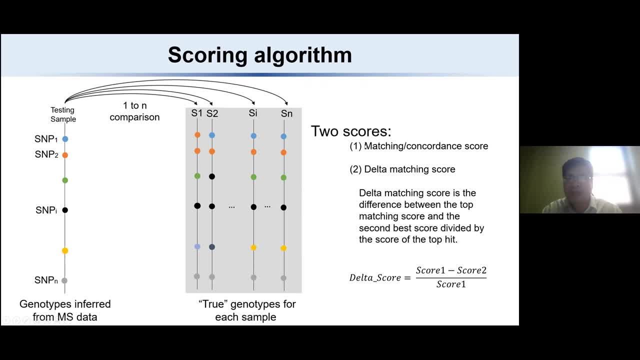 And we calculated two scores. One is a matching score, or we call the concordance score, And another one is a delta concordance score. And the matching score means you know the ratio of the matched genotypes And the delta score. 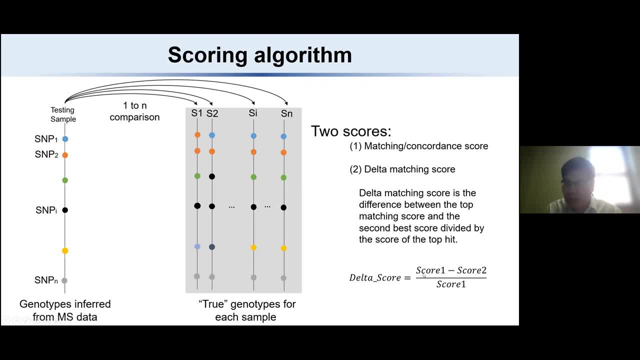 which is a measure of the first hits minus the second hits divided by the first hits, and which is kind of how specificity of the matching and which is actually also you ask very good indicate to separate it from the true hits, from the false hits. 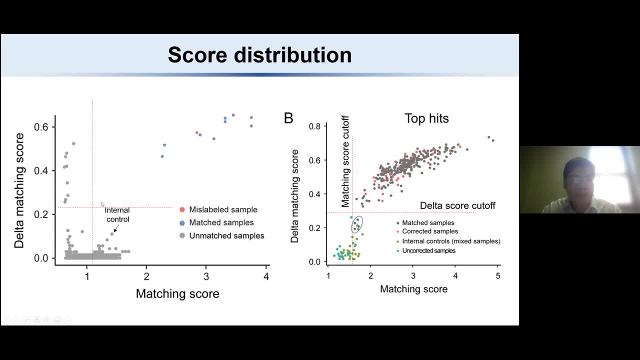 And here is the result from one batch And, as you can see, there's one example- is mismatched because we give our SNP view a higher matching score and a higher data matching score, But the example, the sample, the sample ID was mislabeled. 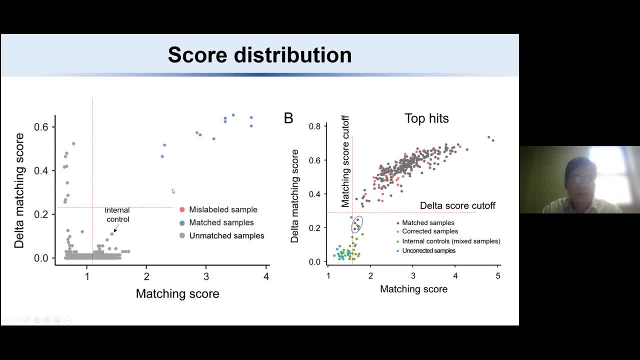 before all the other samples are cracked and matched to original samples. And you can also say the internal standard, which is a mixed example. it just give you lower matching score and lower data score because this sample is the genotype of this sample is a mixture. 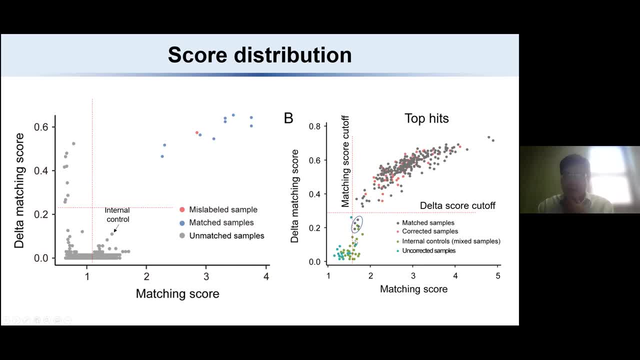 And then we also applied all this, our SNP program, to all the 288 samples And we identified 54 mislabeled example in our data And to where all the sample. we can actually cannot crack it through our approach And as also you can see, this internal standard. 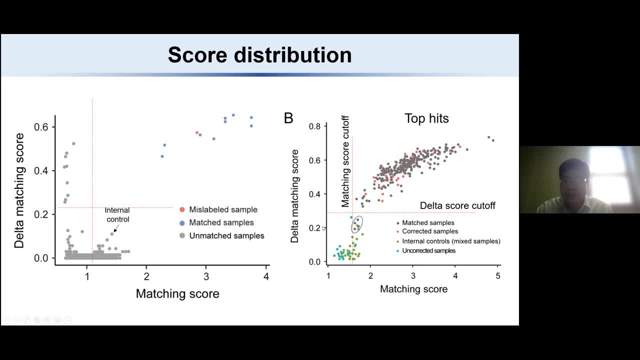 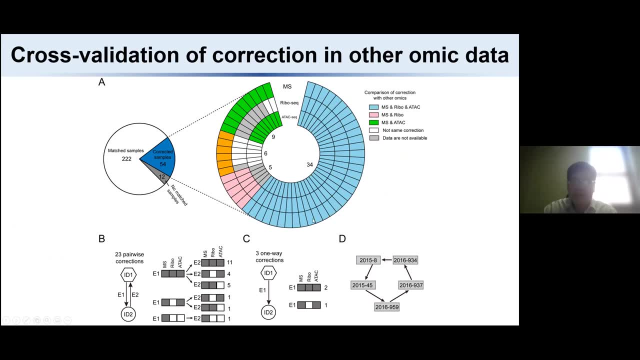 also show very, very low matching score, Matching score and the data score. So then we performed a cross-validation about our correction with other omics correction: As I told you, we make a correction for the ATAC-seq and the RIVAL-seq. 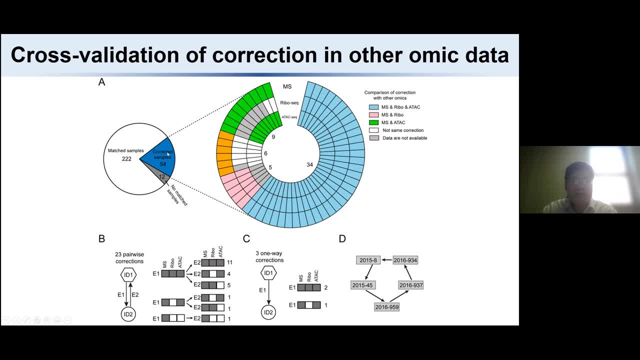 And among this, 54 cracked example, 34 example actually was cracked across three platform, including mass spec and RIVAL-seq and ATAC-seq, And five example were cracked between by both mass spec and RIVAL-seq, And nine mass spec and ATAC-seq. 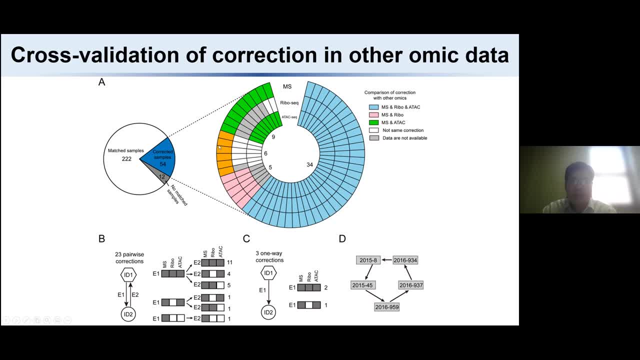 And also have six, which is mass spec, unique platform, specific fraction- And if you look at all this, we looking into the mass spec and the mass spec. And if you look at all this, we looking into the mass spec. And if you look at all this, we looking into the mass spec. 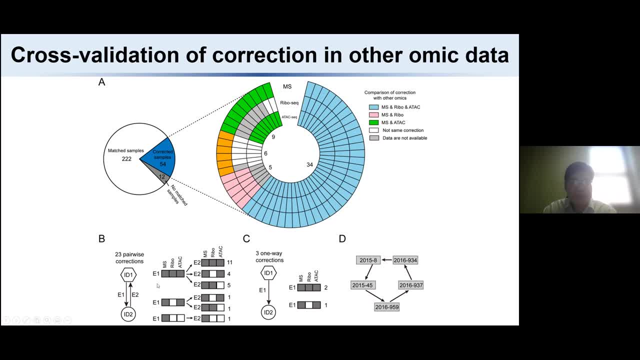 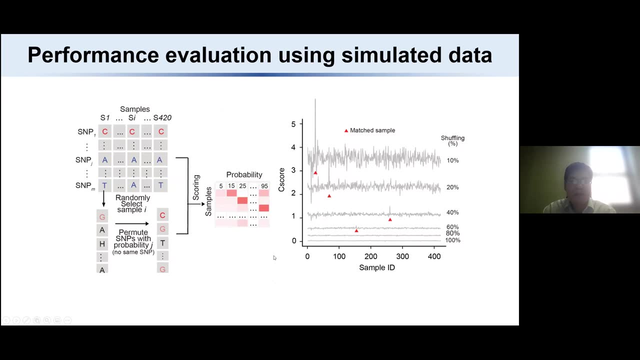 And more close about this swapping and how this mis-leveling occurred. And the vast majority are actually pairwise swaps And we also observe one example that is a loop swap, And so for our data, we also do some simulation to see how many SNP is enough for a loop swap. 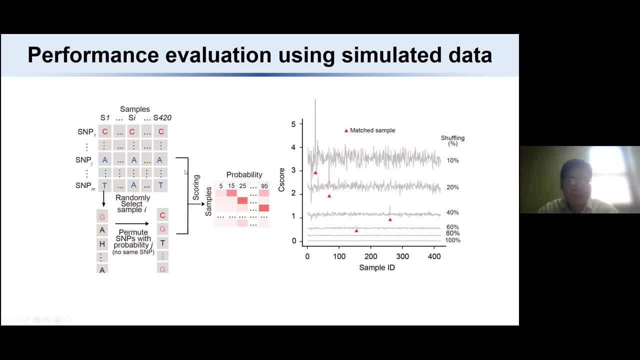 So we look for for SMAP to crack examples And we basically we simulate data by shuffling the SNP in example And, as you can see, if we shuffle 60% of the genotype, we're still able to identify the right examples. 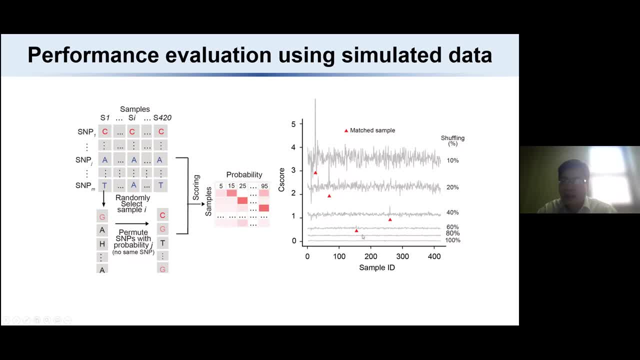 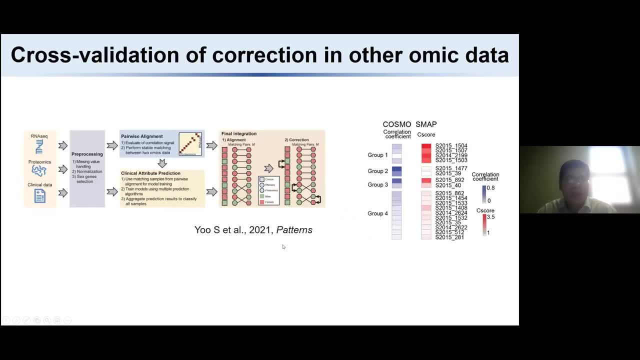 If you have more than you were not able to identify the right examples. And we also, you know, cross-validated with other tools and recently tools are published by Bing Zhang group and you know using expression level when they this tool called Cosmo. 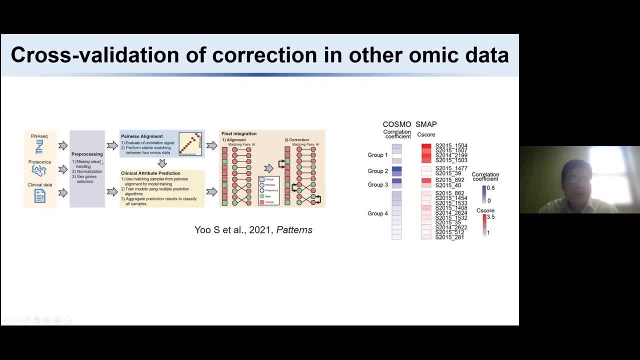 they first selected the features and then those features are highly correlated protein and genes across all the example And then they use this features to see whether this is a match examples And after we also apply this Cosmo to our data and about 94% was example of consistent correction. 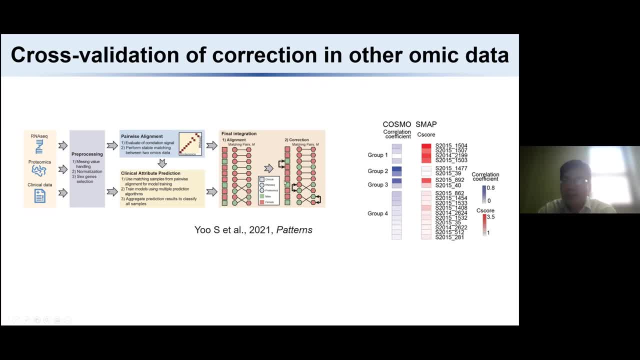 made by SMAP and Cosmo And so we found that we SMAP has four correct fraction, but Cosmo make mis-adjustments And also Cosmo made a two right adjustment. SMAP didn't adjust it And they have two samples both. 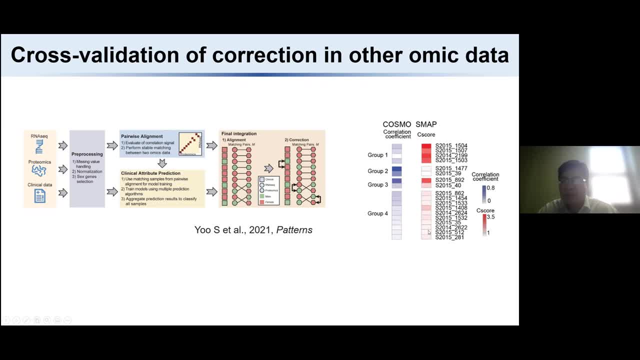 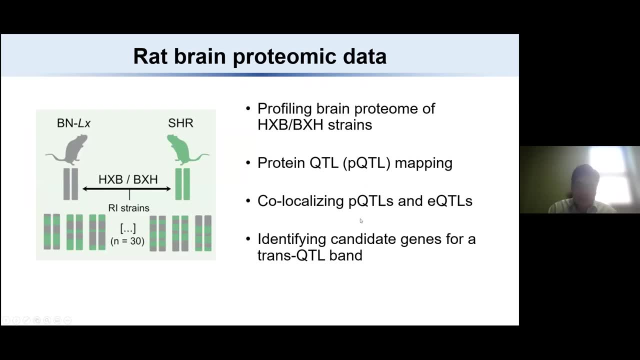 were assigned different IDs by COSMO and SMAP And about 10 samples. both approaches cannot give all right examples, And so at the final step, I will briefly discuss this red-brained proteome data And we, in the early this year, we propose a red-brained proteome from 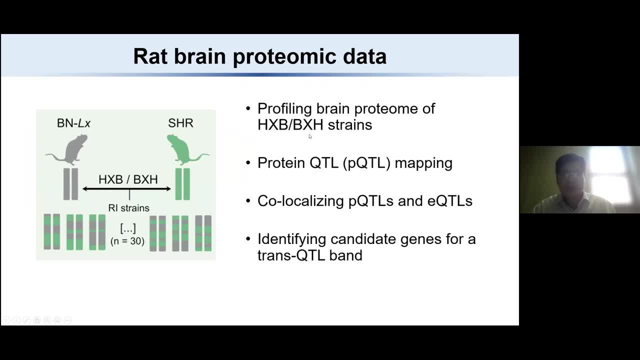 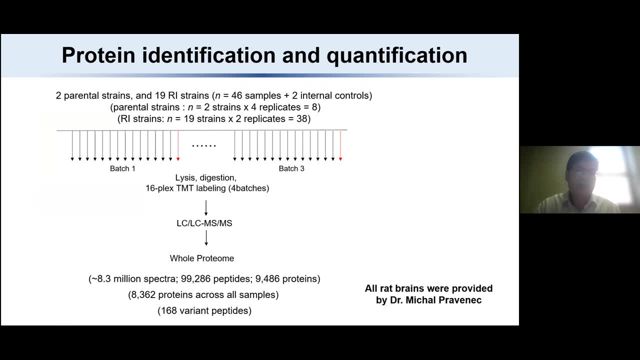 this HXB and VXH gene, And so we generated this proteome data from 21 genes, including two parental genes and 19 RS genes, And so using three batches of the 16-packs TMT And at the end we identified we generated 8.3 million spectrum After database. 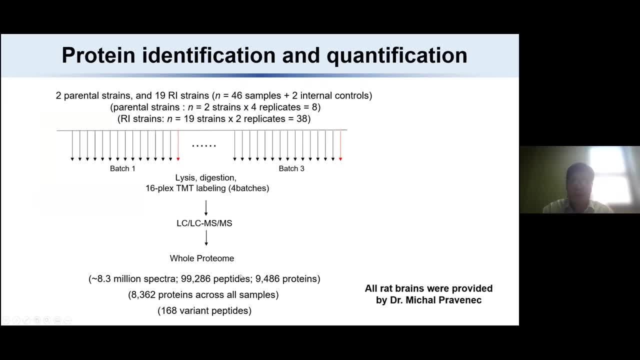 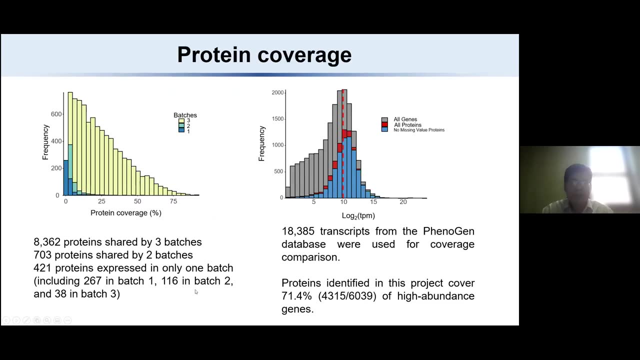 search, we identified 99,000 peptides, which correspond to 9,000 proteins, And among this 9,000 protein, 8,000 protein were quantified across all the samples, And so the vast majority of this protein was from the HXB gene, And so we identified 99,000 peptides, which correspond to. 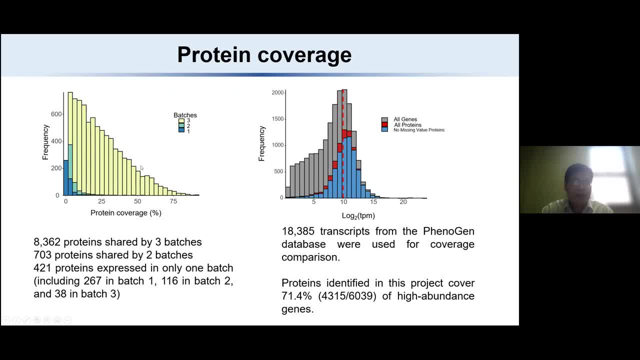 9,000 proteins And among this 9,000 protein, 8,000 protein were quantified across all the samples. And so we identified 99,000 peptides, which correspond to 9,000 proteins, And among this 9,000 protein, 8,000 protein were quantified across all the samples. And we also, when we compare the 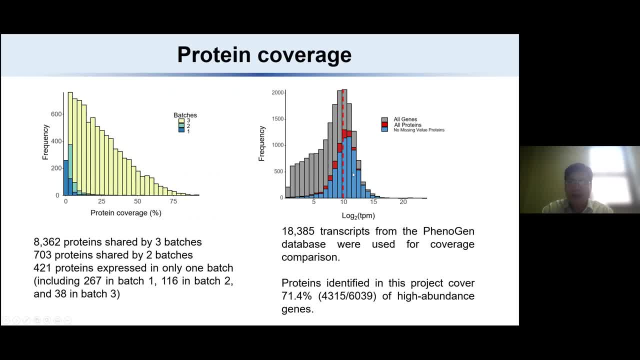 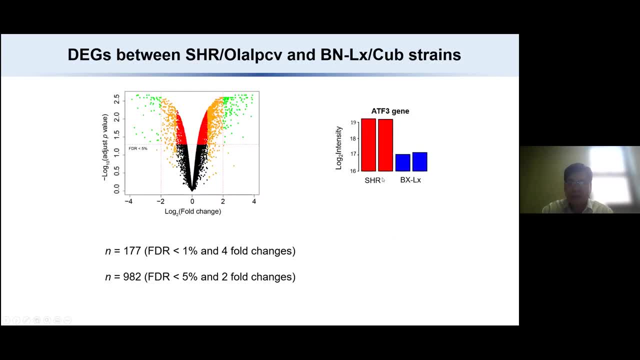 protein expression with the RNA-seq and we found that 70% of this highly abundant gene also detected by mass spec And because we include the two-parental gene and so we can detect the DEG DE proteins between two-parental genes And so we found that around. 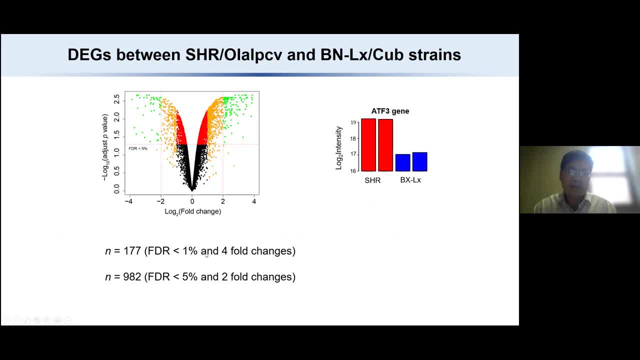 177 proteins at 1% FDR and four-fold change. Here is an example. For example, this ATF3 shows a four-fold change between SHR and BX. Here is an example. For example: this ATF3 shows a four-fold change between SHR and BX, And then. 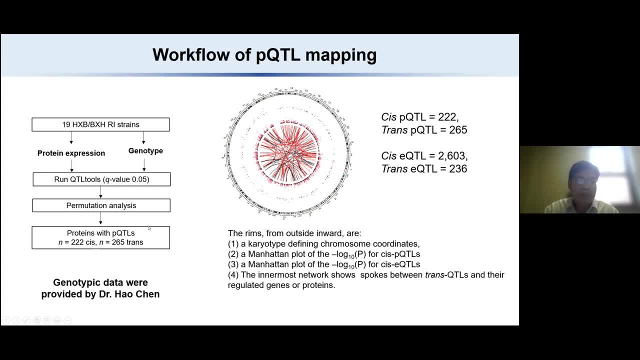 with this data, we perform PQTL analysis, And so at the end, we identified 222 cis-PQTL And we also applied the same procedure to the EQTL. We downloaded the transparent data from phenogen database and then we identified: 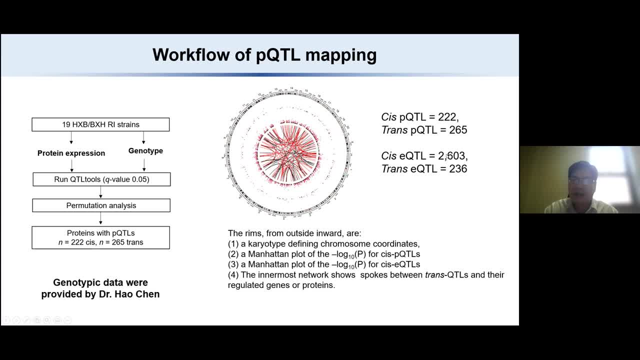 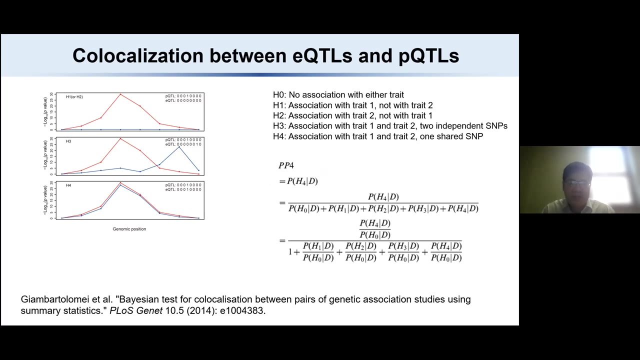 2600 cis-EQTL, And we summarized this PQTL and the EQTL in this circle plot And, as you can see, some of the regions for example. here they are how it shows a consistent PQTL and the EQTL. And so next step, we actually assessed how many EQTL and PQTL are co-log lines. 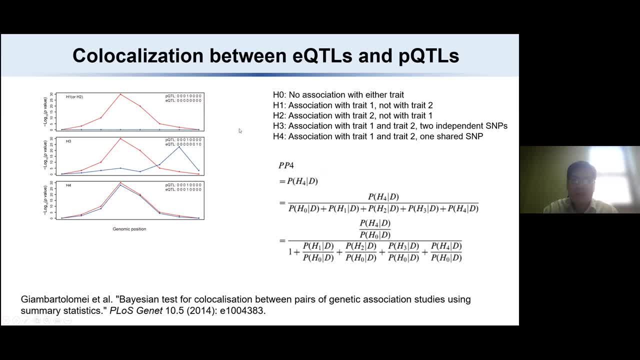 And we used one program called the co-log program. So the idea of this co-log program is: we can summarize this idea using this diagram. So if we use the one as a significant PQTL and zero as a non-significant PQTL, so then we will have either no association for either 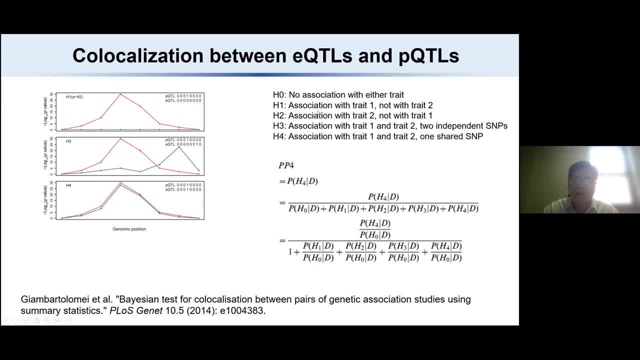 pqtl and eqtl, Or we have association in the pqtl but not in the eqtl, Or we have association in eqtl not pqtl. The first case is you can have both significant qtl but we have a different SNP control the qtl. And the final case is we have the same association but they also have the. 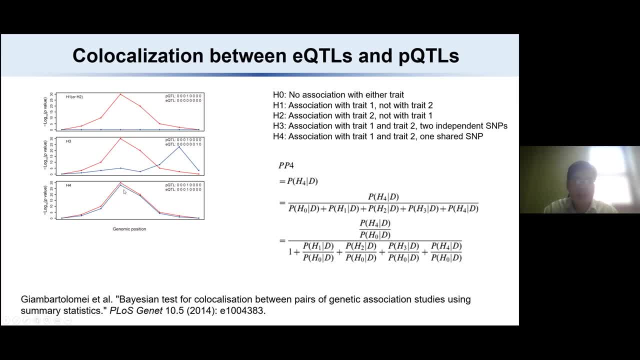 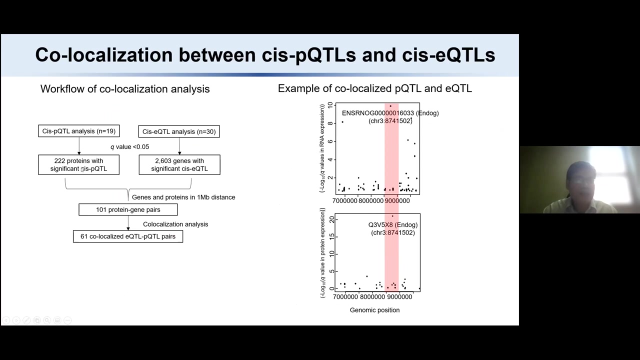 same qtl, the SNP control the expression And with this assumption and they calculate the probability at the end, they calculate the posterior probability for this pqtl, this assumption, If this assumption is the largest probability, and then they think this is a chloroxyme. So, as I said, we detected 222. 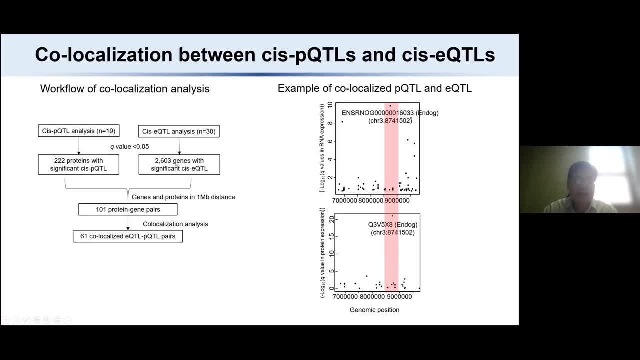 spqtl and 2600 seqtl. And then we look at how many protein and the gene pairs are within the one megabits distance And then we identify 101 pairs and analyze it by correlation localized issue program and we identified 61 co-localized eqtl and pqtl. And here is just. 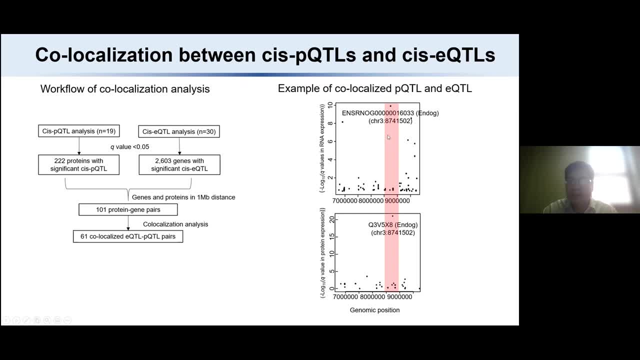 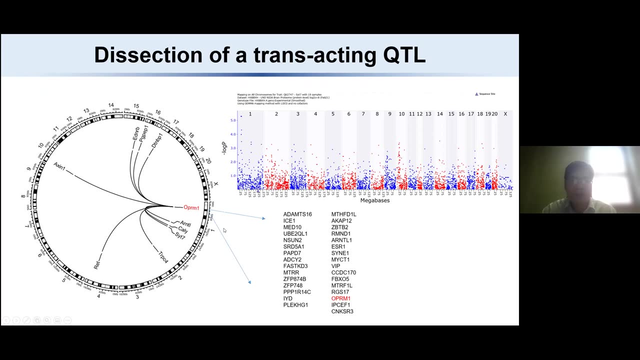 give you one nice example, and this is a show. this eqtl here and the pqtl here. Both are punctured by the same scene And here this is a one of the nice transqltl from this proteome data. I will pass this one to Rob and Rob will tell this nice story about transqltl. 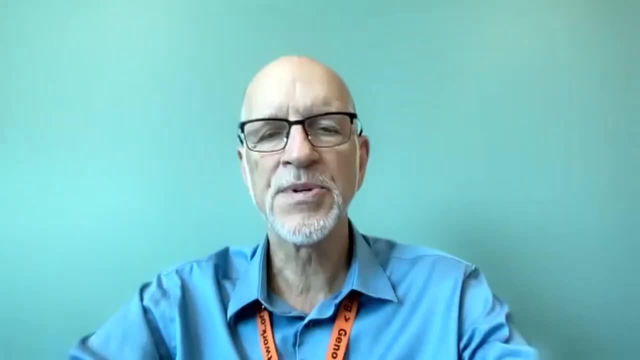 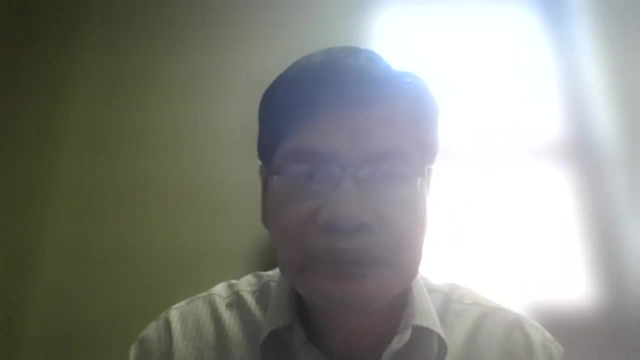 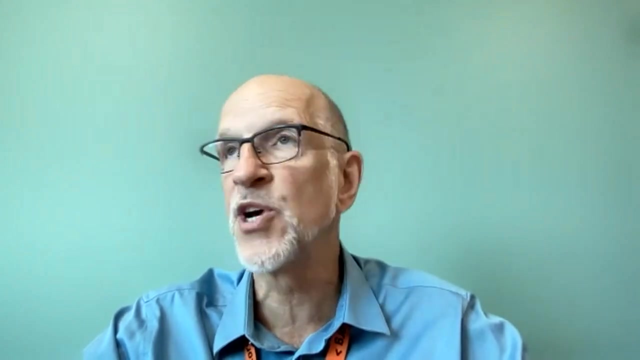 Thank you so much, Xu Sheng. That was. that was great, And I just in the chat it just. you know what I thought was great about what you presented is it was a really good summary of the alternative methods for doing the proteomics. But the beauty for me, 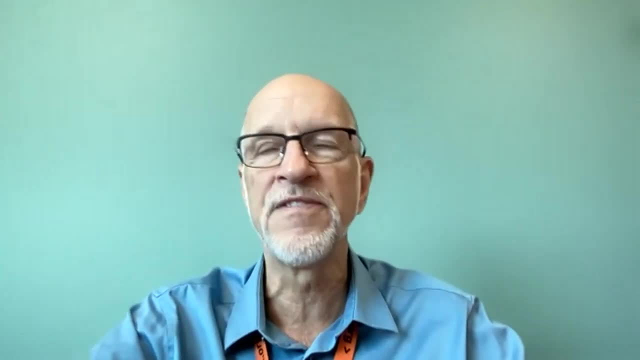 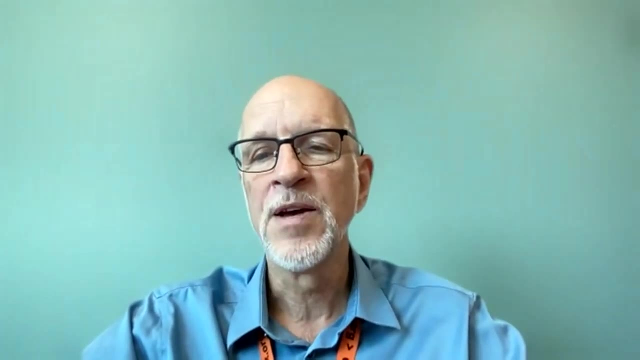 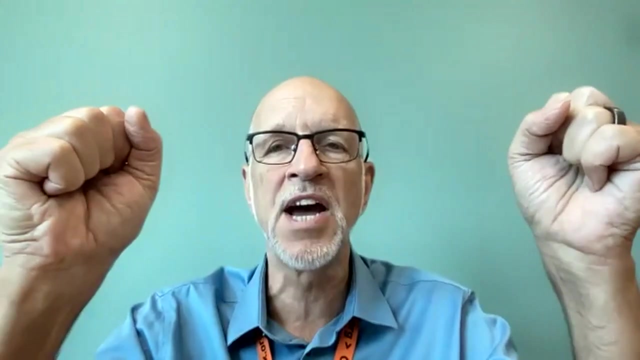 was the recognition of the importance of error control at all stages of these very complicated protocols. So proteomics has been one of those poster childs of almost there for the last 20 years. It's fun, Finally there. So proteomics is now a quite mature technology and the prices 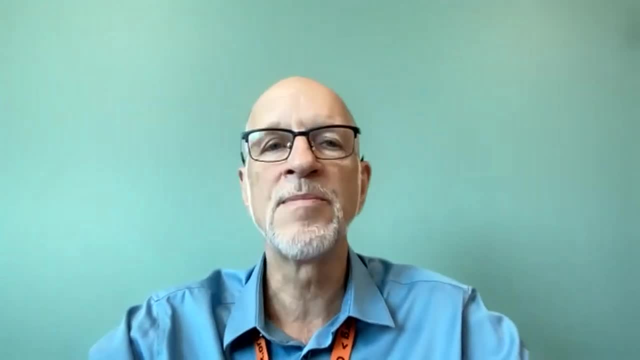 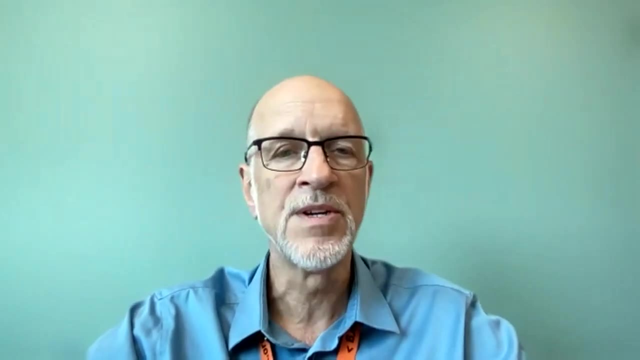 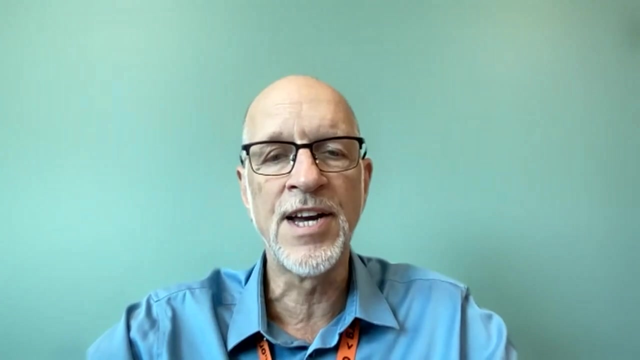 come down, and I think Xu Sheng will have some time to talk about that in the discussion section. But I'm delighted to see the technology come so far so fast. So I'm going to share my screen and we're going to do a dive- not too deep a dive- into Xu Sheng's dataset. 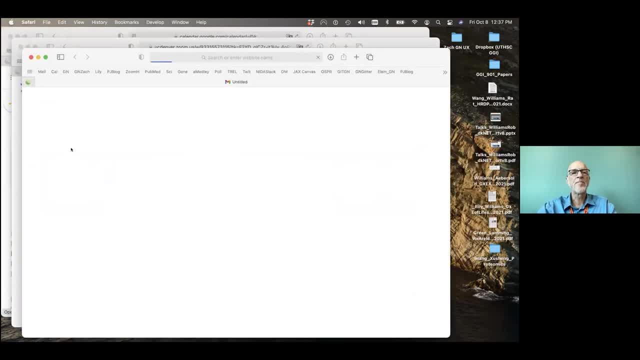 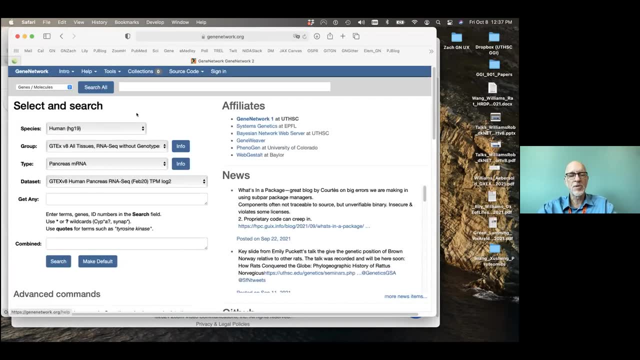 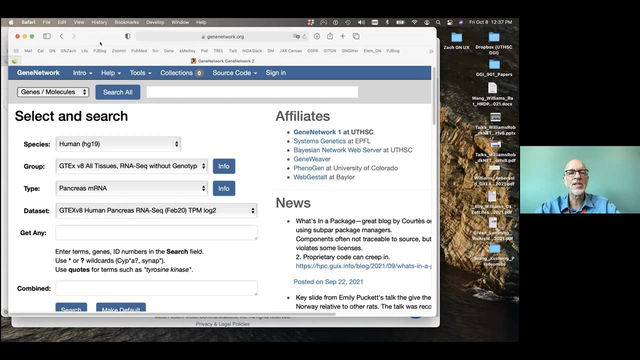 So I'm just opening up a browser and anybody that wants to do this can also do this. I'm going to genenetworkorg, which is a web service that's integrated in the P30, but it's a web service that's also funded independently to Xu Sheng and Piotr Prince. 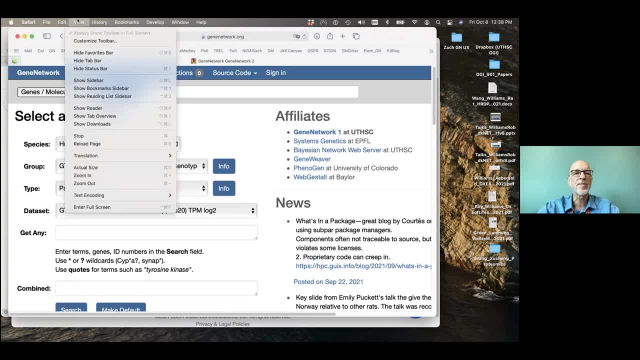 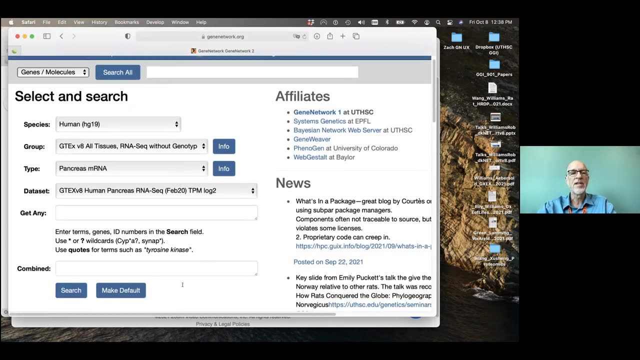 It's actually- I may have said this before, sorry, it's getting probably boring to hear it from me- It's actually the oldest web service in biomedical research, So it started in 1994 as the portable dictionary, the mouse genome, And now it has a lot of human data. 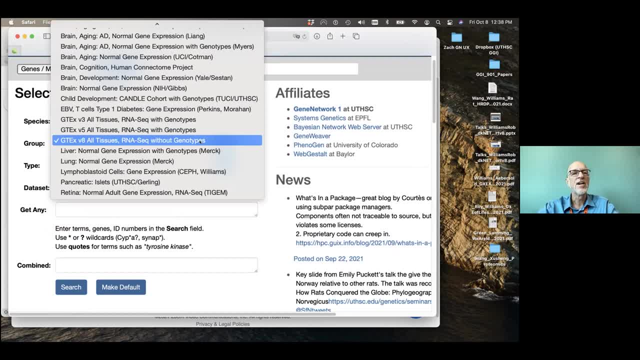 So GTex, for example, is all of there In the human data. you will look long and hard and you will not find any proteomics data yet. So if anybody knows of genetic data, genetic proteomic data, please let me and Xu Sheng and Laura and Seanak know, because we'll put it in. 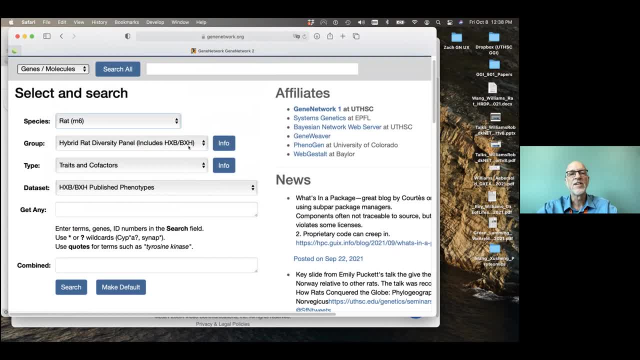 there. So I'm going to switch over to rat, where we do have the impressive data that Xu Sheng and team have already generated. It is in the hybrid rat diversity panel, which includes CHXP, BXH. It's not a traitor cofactor, So traitor cofactor would be something like body weight or a classic. 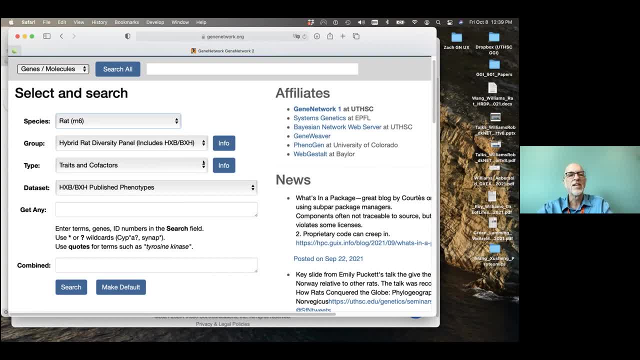 phenotype, like response to cocaine or morphine. It instead will be down here in the molecular traits, aka endophenotypes, And what you just heard about is one of two data sets that Xu Sheng has put in here under brain proteome. I don't think time will permit, but I'm going to show you. 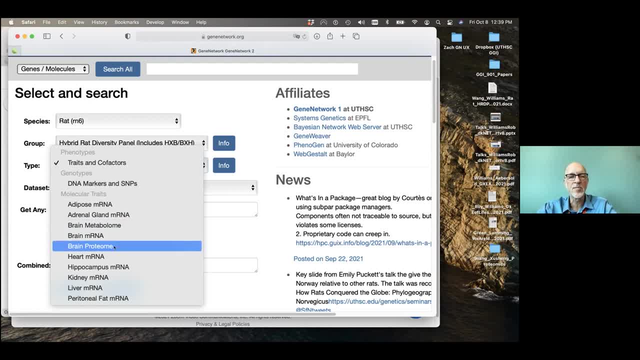 I'm going to include a little document for you so you can look at the brain metabolome. This is the data that Laura and team have generated over the last five plus years with Boris Tabakov and colleagues Paula Hoffman. It's a really beautiful RNA for the whole brain. Some of these are older data sets that our group 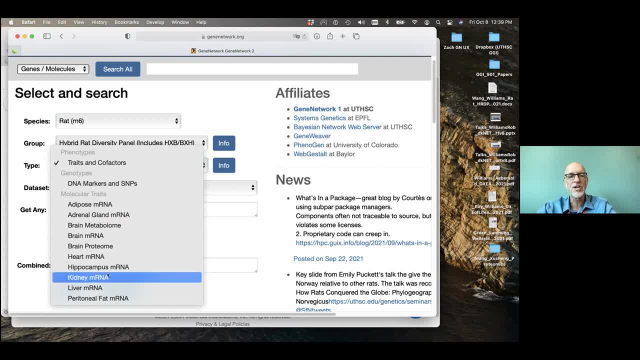 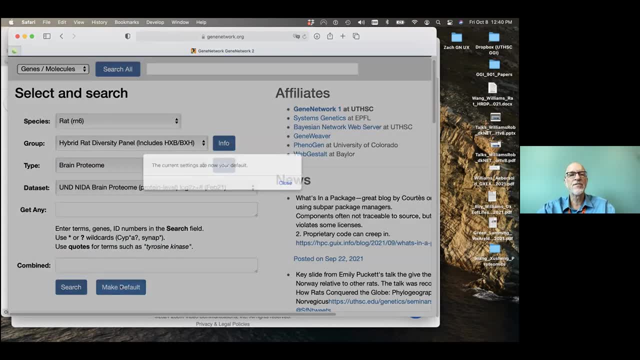 here generated for mRNA. A lot of these are star consortium data sets, but this is our data set of the day. I'm going to make it my default Before I dive into it. I just want to show you that there are actually two data sets that are generated for mRNA. One of them is a. 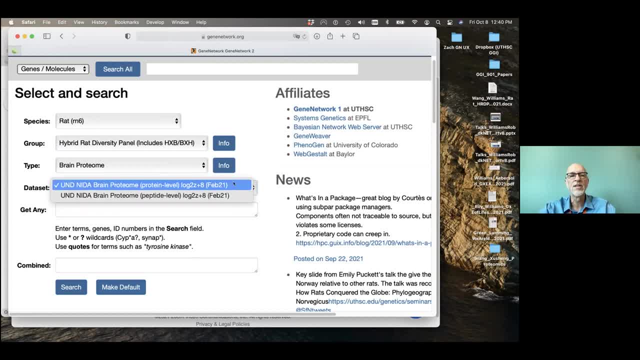 gene-type-2 data set. where we can. Here is the gene type-2 data set. This is the gene type-2 data set that goes into the genome. Just a little bit of an introduction to gene type-2 data sets. It's going to give you a little. 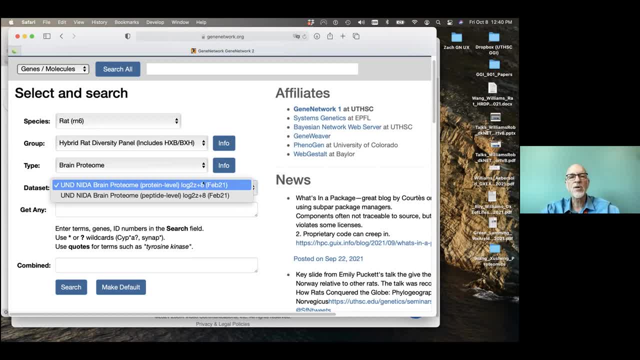 bit more detail about gene type-2, or gene type-2.. The brain itself is made up of two levels: Xu Sheng, a late 2021 data set, or maybe a 2022 data set, which will be slightly larger. I am going to now share. 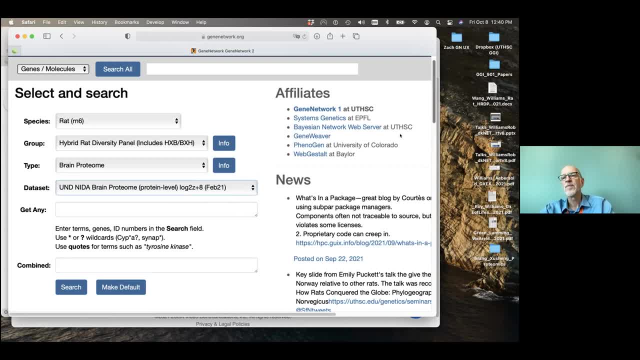 a document with you in the chat. so make sure you've got your chat window open and I'm going to send you a not very long word document. I hope most of you can get that. I still consider- unfortunately still consider- word to be our lingua franca, So have a look at that if you want. 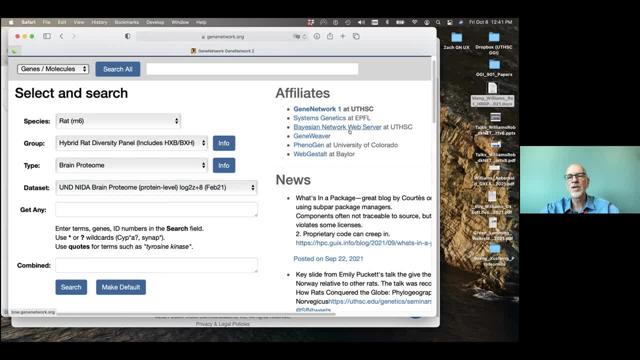 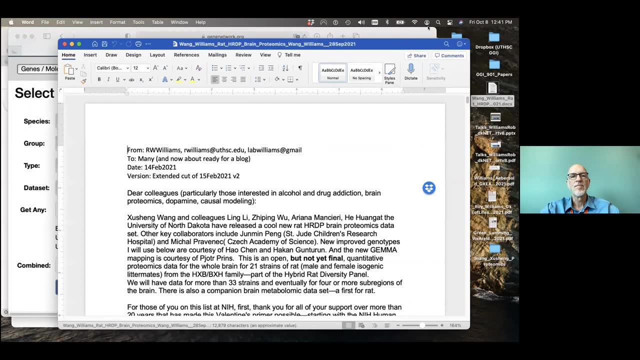 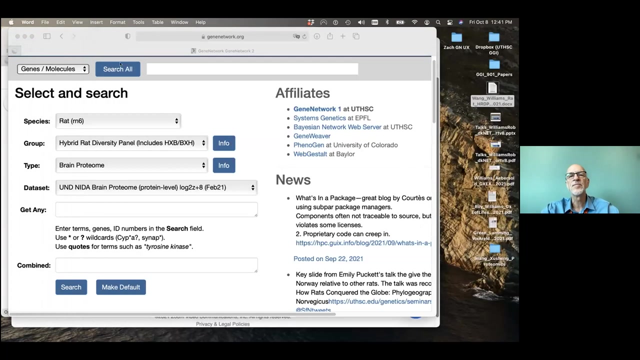 to basically do what I'm about to do. And what I am about to do is basically go through this, this document. Let me open it up just to give you a feel for it. So actually I think I might have given you the old version. Let me get the new version. I'll put that. 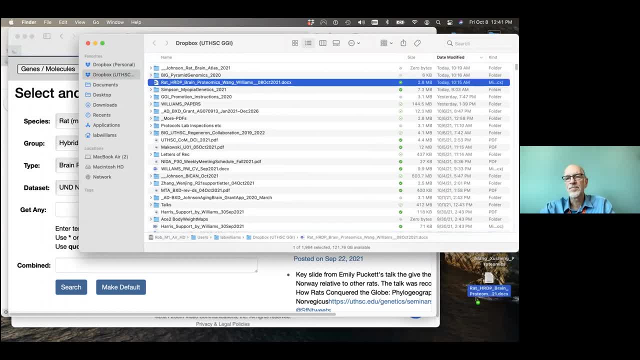 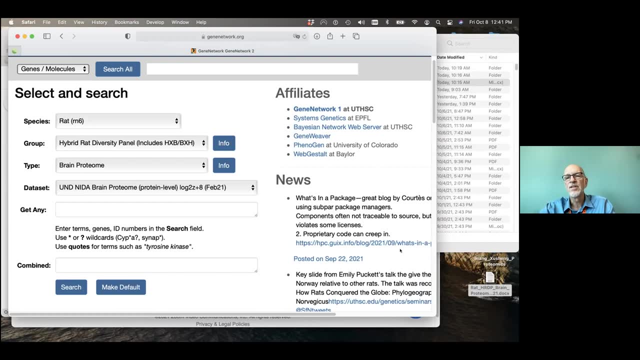 This is the new version I actually want to give you, So let me update that. You can, if you downloaded that one, throw it away, Giving you a slightly beefier version that doesn't have as many typos. So take that second one. 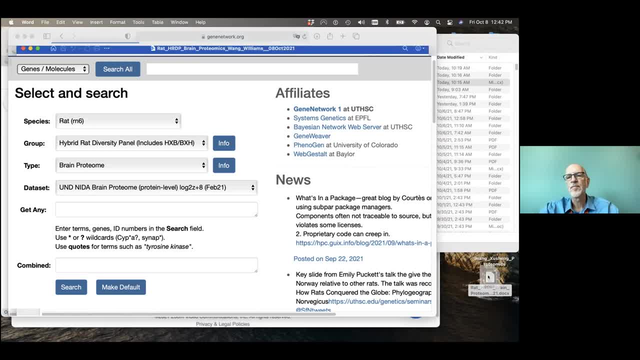 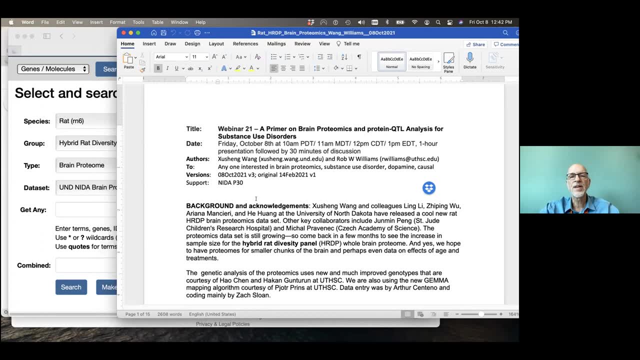 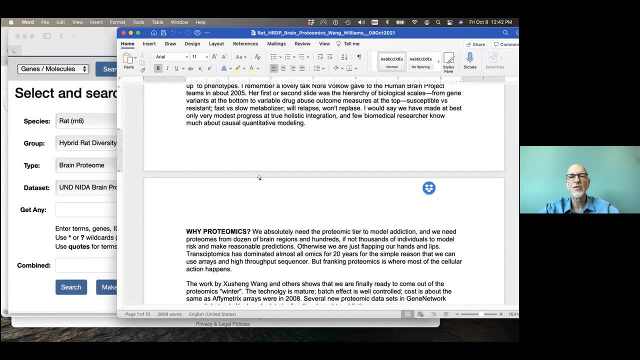 And let me open it. So here is what that'll look like. It probably is something. the good thing about having this on a Friday is now you can spend all of your Saturday and Sunday going through this and making sure you can do some cool things with proteomic data. 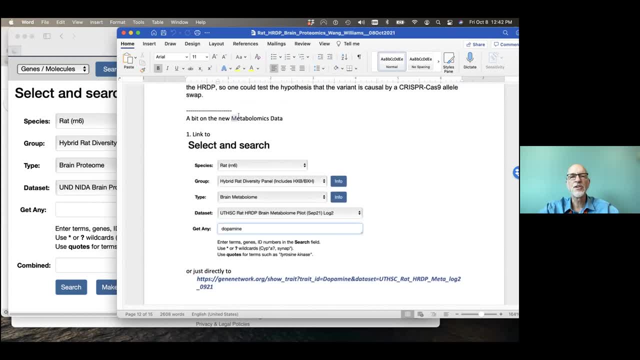 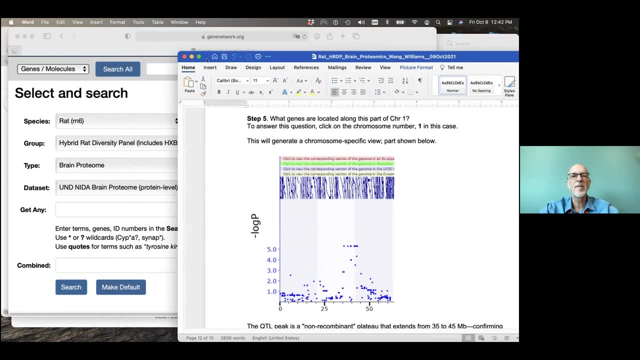 and if you're interested in the metabolomic data itself will probably let me open it here- And then probably did all this with a little whiteboard data. There's a little bit about that, So I will keep that in the background in case. 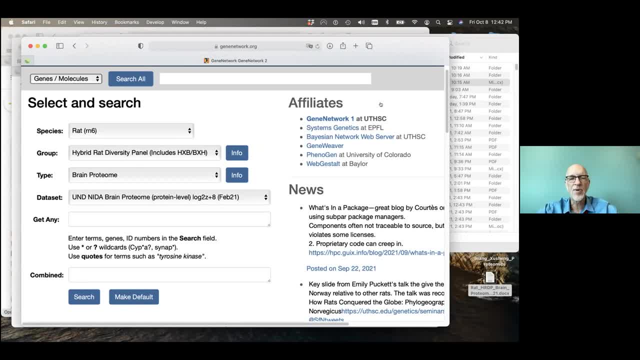 Gene Network does something persnickety while I'm talking, But let me show you how to use these data sets. Hybrid rat diversity panel proteome: choose your level. So if you're really interested in peptide level, as Xu Sheng mentioned, there are about 100,000 peptides in there. 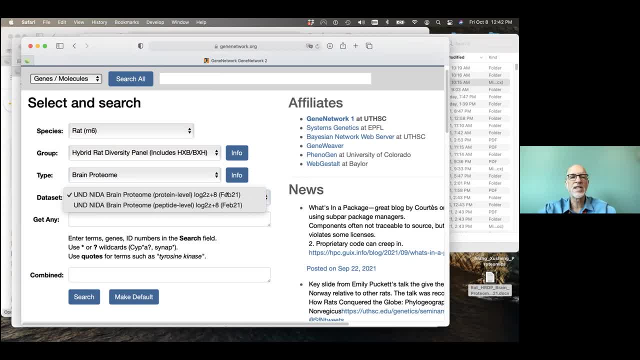 and about 8,500 protein assays here. I and many of you that are interested in substance use disorders will be interested in a large number of proteins that are, for better or worse, for worse. for today are membrane fractions, or membrane-bound proteins, If you look for DRD1. 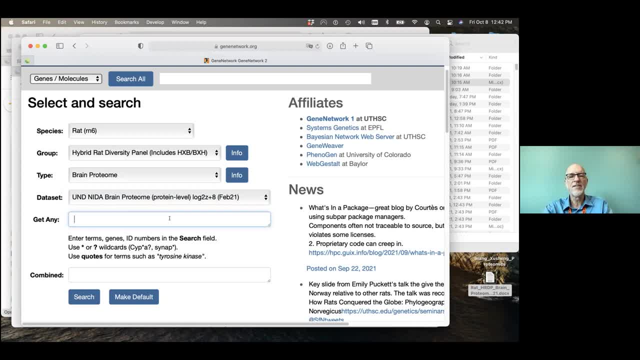 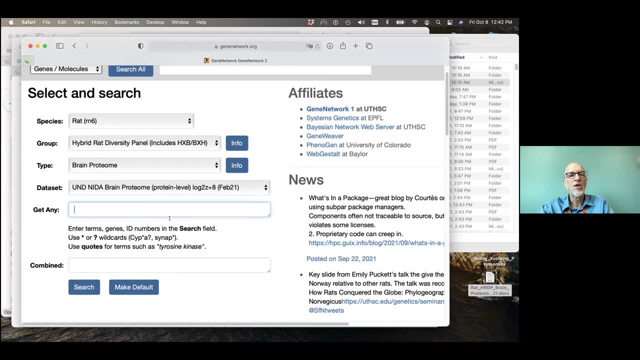 or DRD2, expect to have a little bit of a heartbreak. If you're looking for a GABA receptor, expect a bit of heartbreak. But here's a way to overcome some of that problem. There's some advanced commands down here and I'm going to use this. 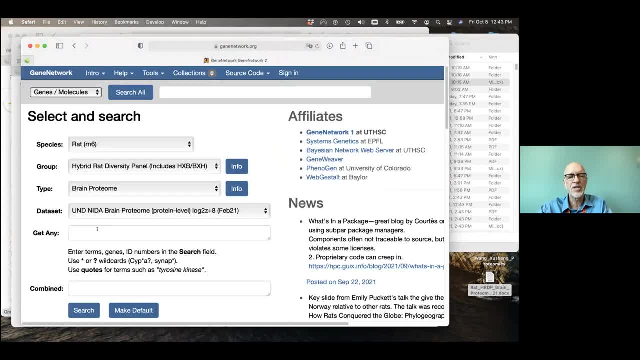 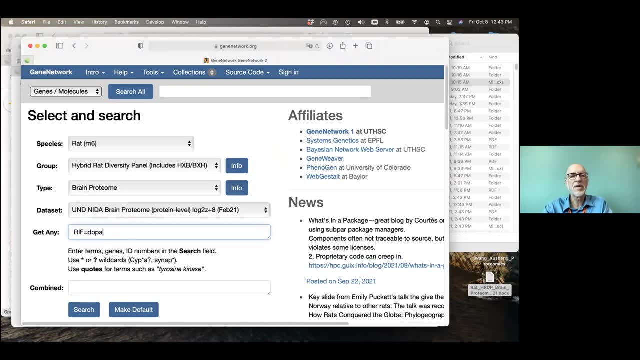 advanced command. I'm just copying it. I'm going to put it in the get. any, I'm not interested in mitochondria today. I'm interested in dopamine 1,001, 1,002.. If I'm not competing, 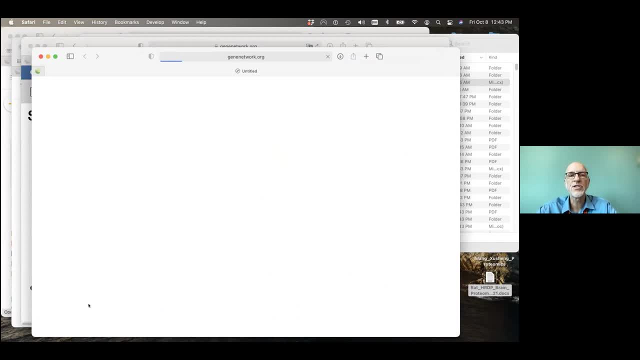 I'm not competing with too many of you for using the service. This should take about 10 seconds. It's looking through every one of the proteins, comparing it to RIF. RIF stands for reference into function- and asking: do any of the reference into function entries in NCBI for gene X, Y? 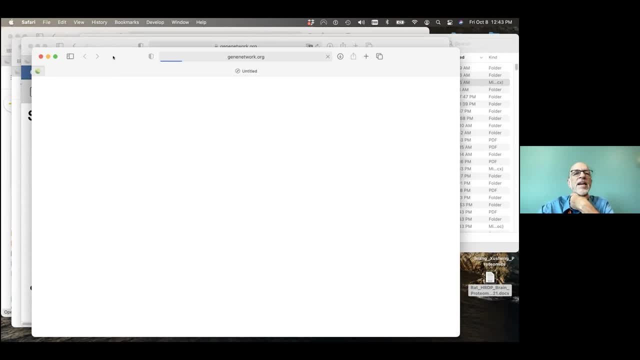 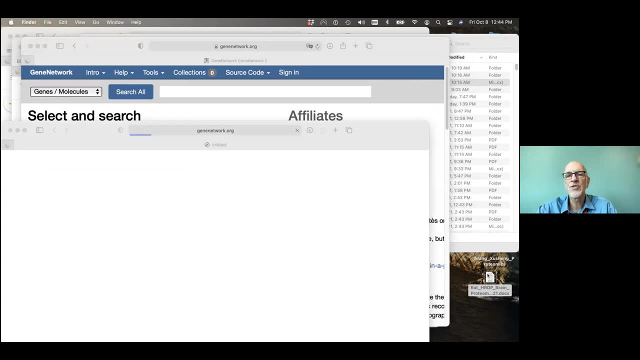 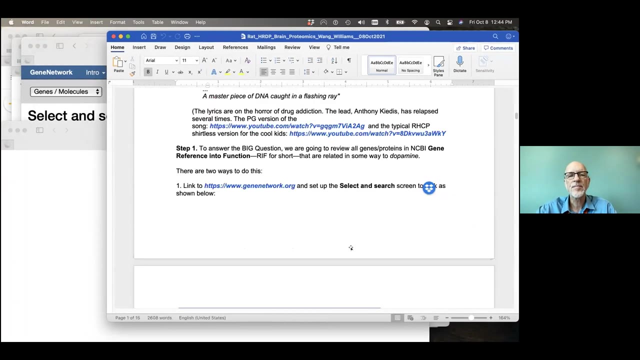 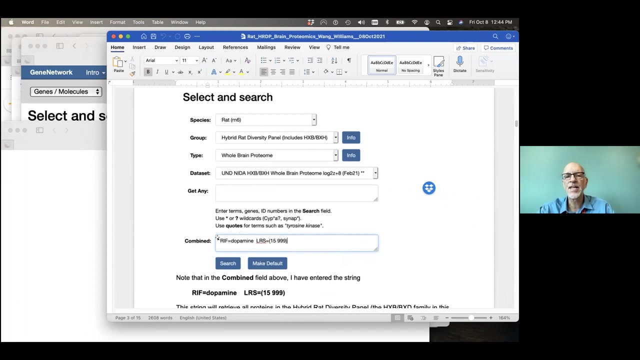 and Z have the word dopamine in them. Working on that, I will show you what the result will be, just in the interest of efficiency. So this is basically what we did In this case. I actually did a slightly more sophisticated search. 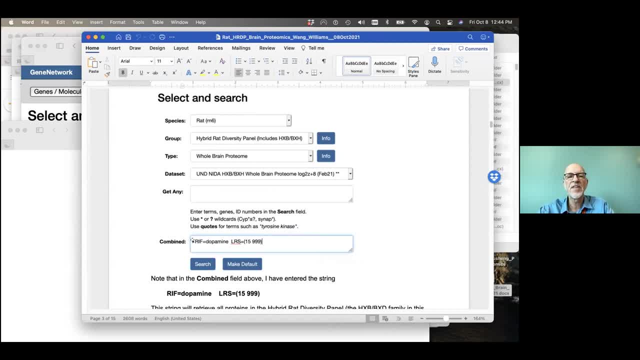 I did a search that combines two terms, The one that I just introduced you to: RIF equals dopamine and LRS equals 15.. So I'm going to do a search that combines 15 to 999.. That means that the LOD score, or the minus log P, 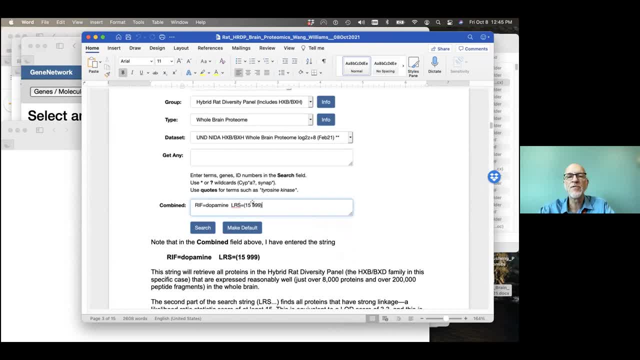 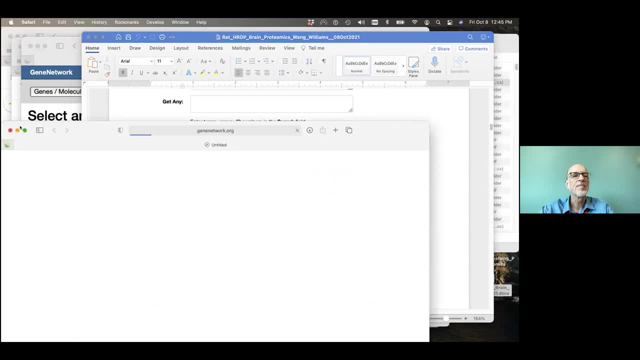 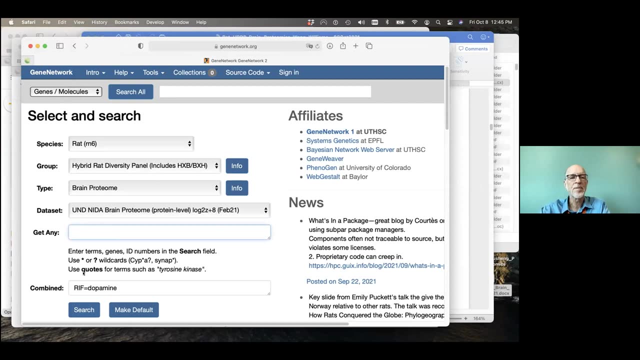 or the likelihood ratio statistic has to be between 15 and 999.. 999 is a very high number and will not be a problem. Let me try to literally do that and see if it's still cached somewhere. So I'm just going to do what you see there in the document. 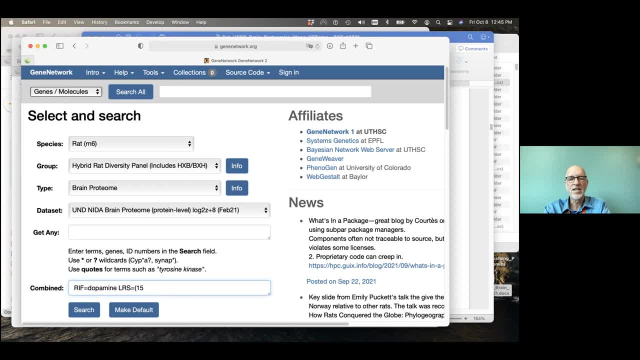 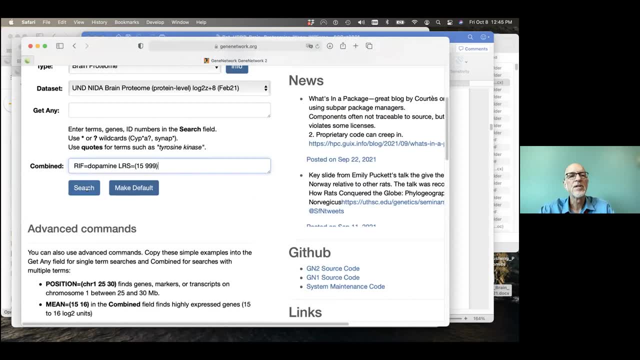 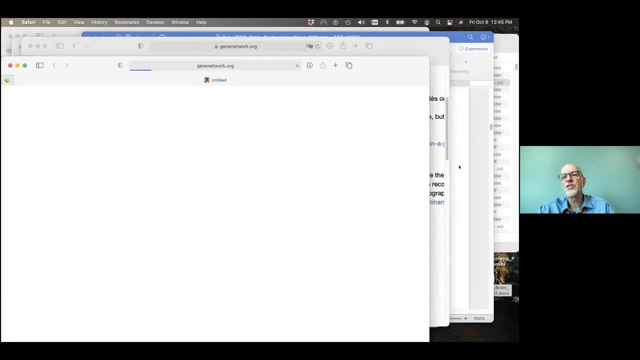 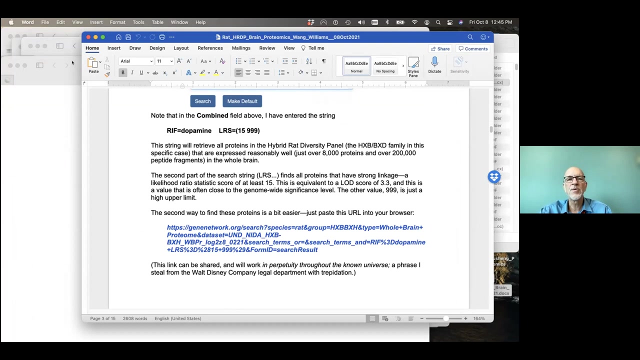 Here's P equals between the range of 15 and 999.. And we'll do that more complicated combined search, And I will let that run in the background with a little more patience than I did. So what this should do if I'm again not competing with too many of you. 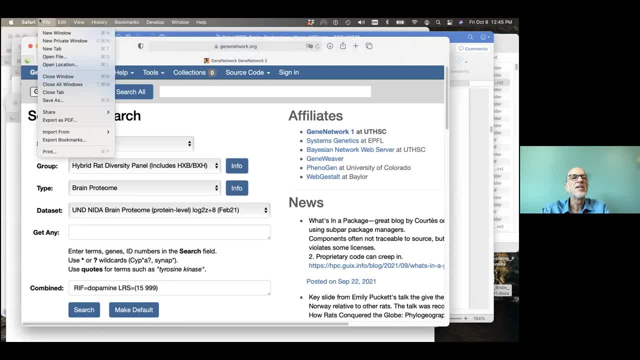 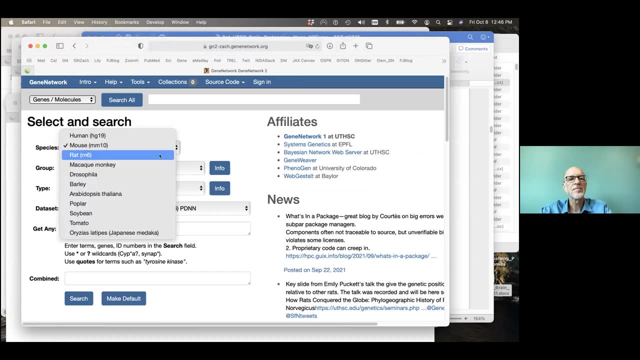 And in case I am competing with too many of you, I'm going to do this. RIF equals between the range of 15 and 999.. do something a little bit tricky. I'm going to go to another service And go here. I'm going to make this my fault. So this is a staging system we use. 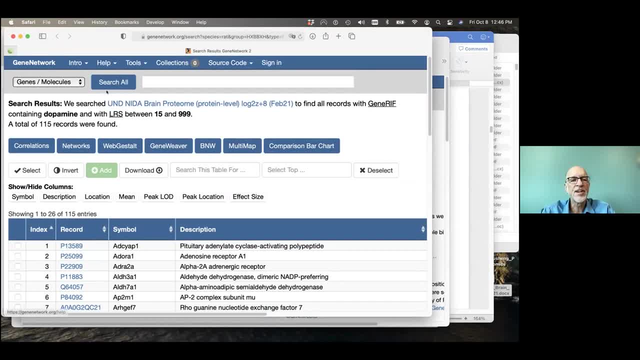 Oh, okay, So I just am not quite patient enough. So this now found 115 records in that particular database associated with the gene riff containing dopamine and a pretty good linkage statistic where 15 is sort of low but reasonable. And these are the names of the genes: 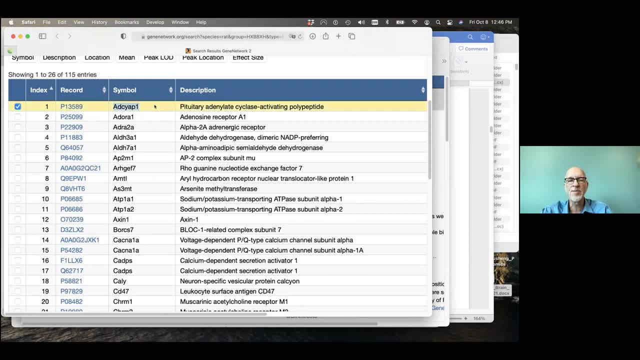 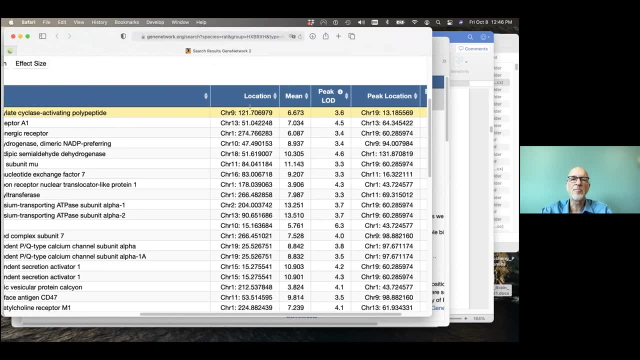 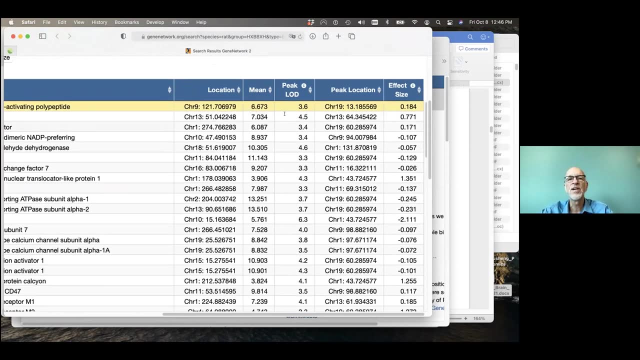 or proteins actually. So these are actually protein symbols, or should be. They should be all capitalized: The location of the cognate gene of that protein, the mean expression level in this log two space that Xu Sheng introduced you to, the location of the peak log score minus log p, and where that 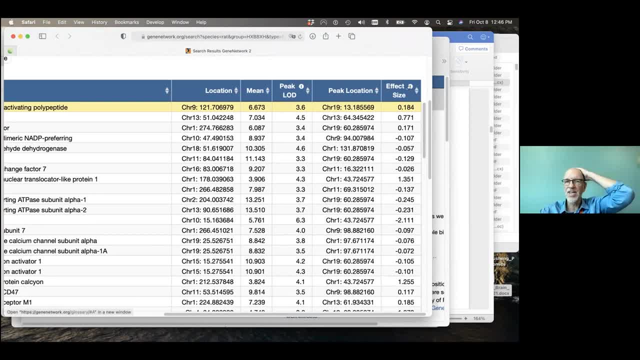 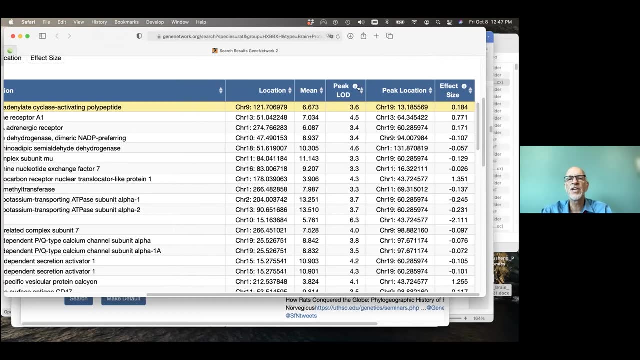 peak is located and the effect size- The little. i here will tell you what the heck is an effect size. I'm going to finesse that. for now I'm going to do something pretty crude, which is called fishing. I call it trawling. So we're going to trawl for all of the good genes that are linked to dopamine. 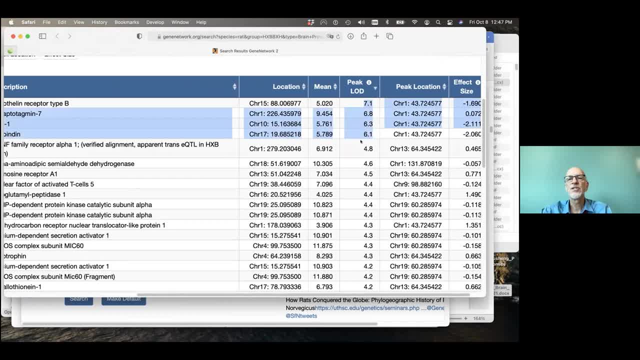 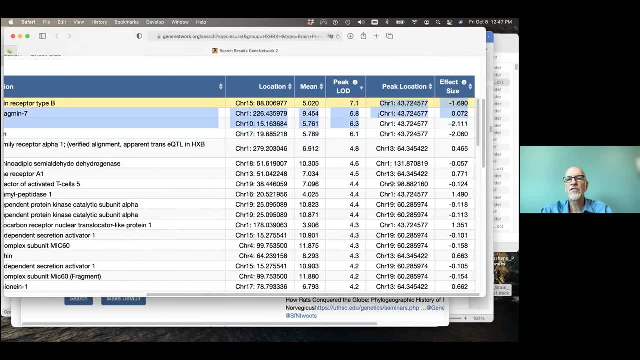 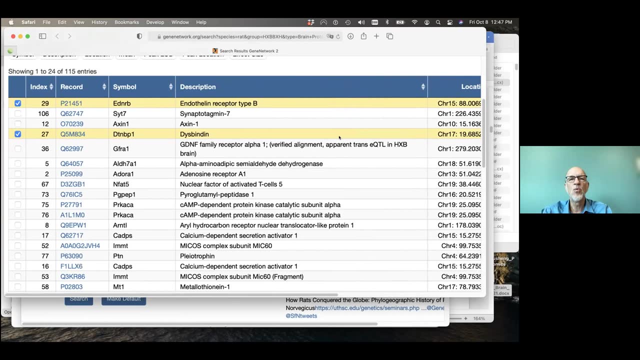 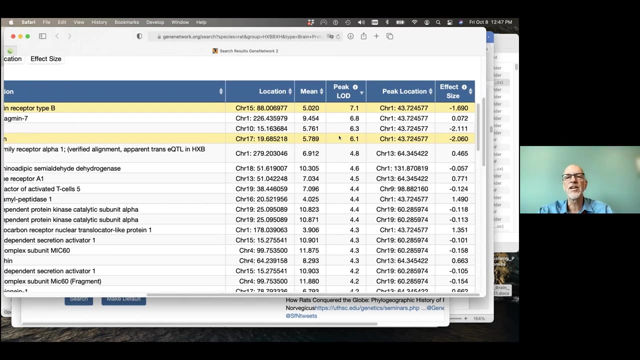 and have very high statistics. So these are log scores above six. And what's interesting is those first four all map on chromosome one at roughly 44 megabases. What is going on? Xu Sheng showed you that he can systematically map all cis-eQTLs and trans-eQTLs. 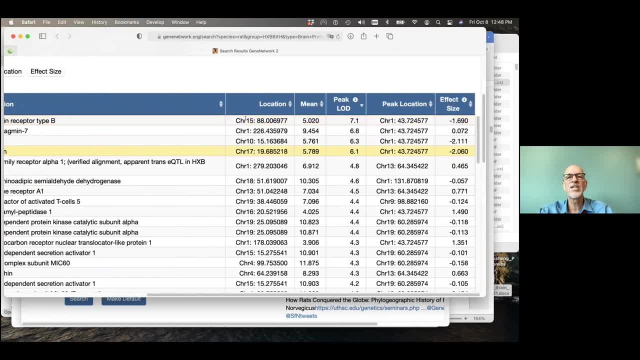 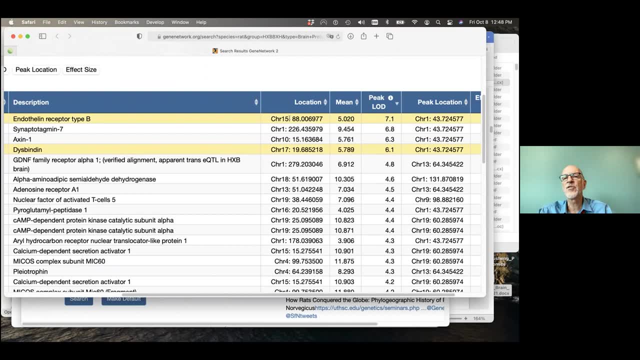 So the first question is: are any of these proteins cis-eQTLs? So the endothelin B receptor, the gene, is located on chromosome 15 at 88 megabases. The peak is on chromosome one. So that is actually a trans-eQTL or trans-pQTL P for protein, but E works in a trans-pQTL. So 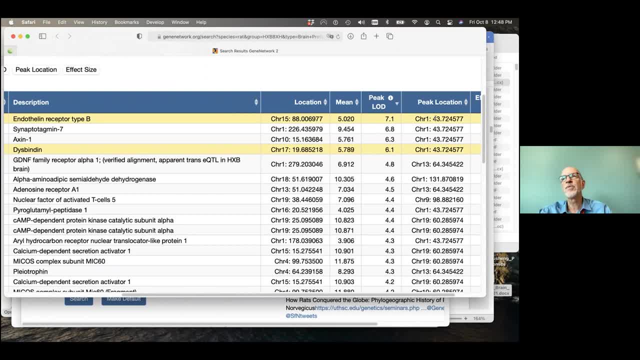 trans-eQTL is a trans-pQTL, So trans-pQTL is a trans-pQTL. So trans-pQTL is a trans-pQTL P for protein, but E works in a trans-pQTL. So trans-pQTL is a trans-pQTL. So trans-pQTL is a trans-pQTL, But E works equally well in my book. 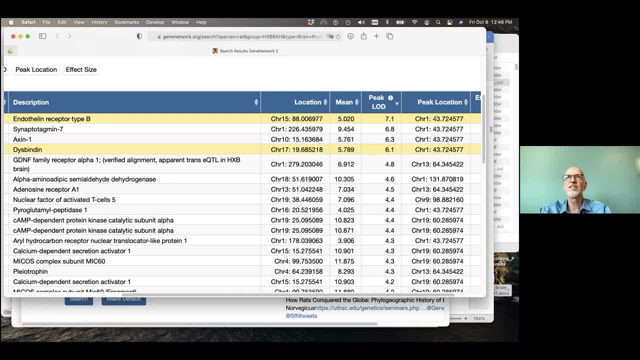 because it's an expression of a protein And the E does not mean anything other than expression, And protein metabolites, peptides, all have expression. So the second one here is synaptotagmin 7, chromosome one at 226, also trans, trans, trans. 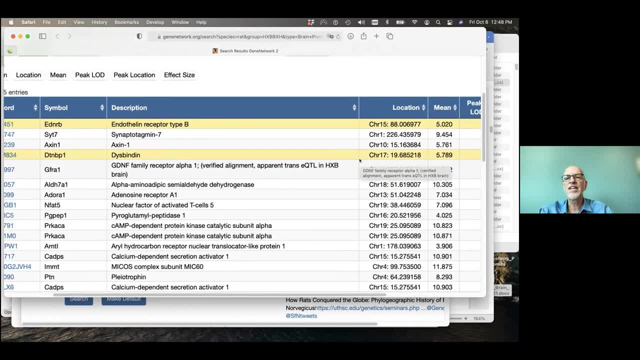 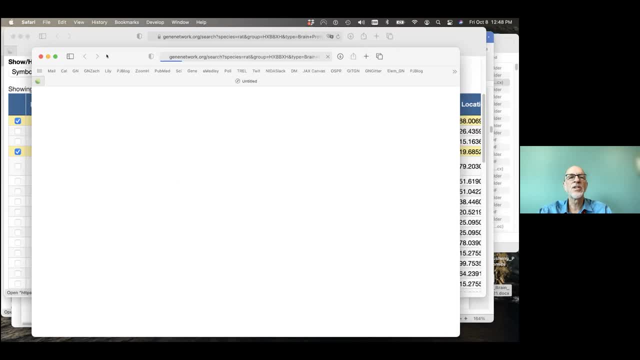 So this is the trans band that Xu Sheng showed you, And let's play with it a little bit. I'm going to pick the second gene on this list And we're going to treat it like a dog would treat a good-tasting bone. 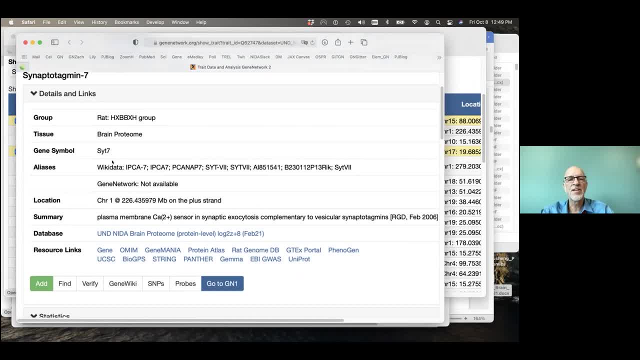 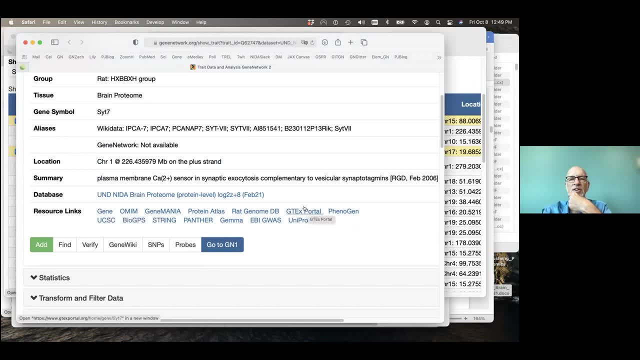 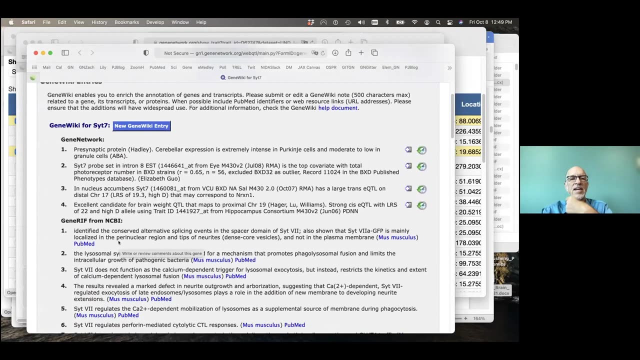 So here it is, synaptotagmin 7.. We want to know a little bit about synaptotagmin 7.. We could go to another link over here, the rat genome database: phenogen. I'm going to go right to the gene Wiki and see what it says. So it's a presynaptic protein high in Purkinje. 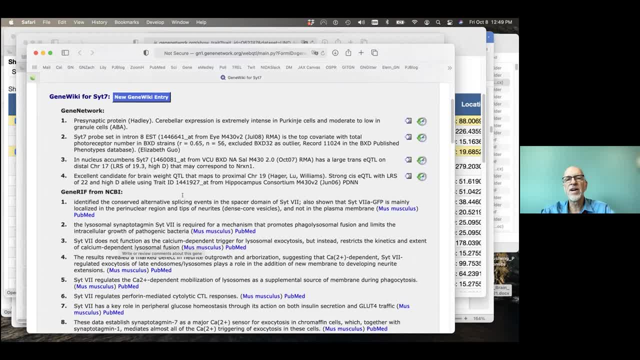 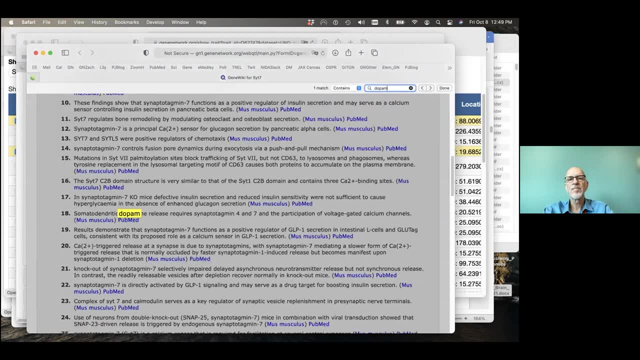 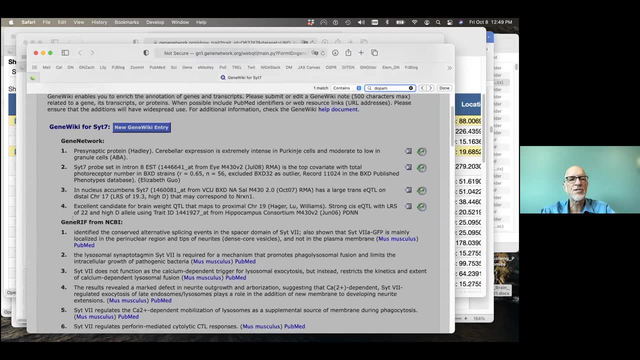 cells, excellent candidate for brain weight in certain datasets. Where did the word dopamine come in There? So I just did a search for dopamine in here. These are all the reference and defunction entries. gene riffs, So somatodend Lyndris. 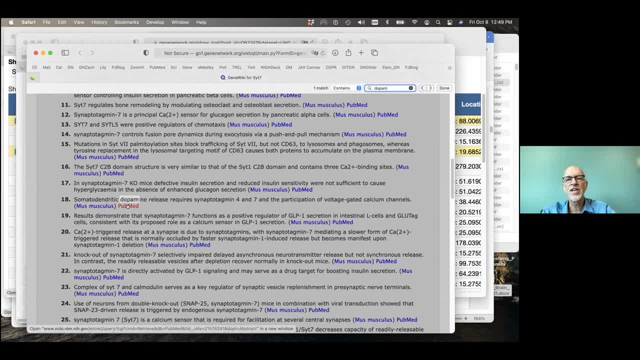 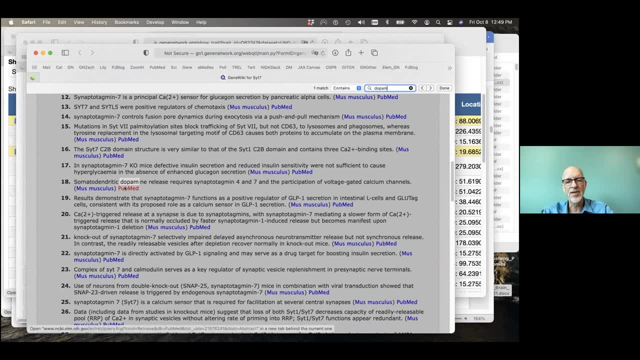 So somatodendrous gene, somatodendritic dopamine release, requires synaptotagmin four and seven voltage-gated calcium channels, And if you wanted to read the paper you could do that. Is that the only appearance of the word dopamine? Yes, The only appearance of the word dopamine. 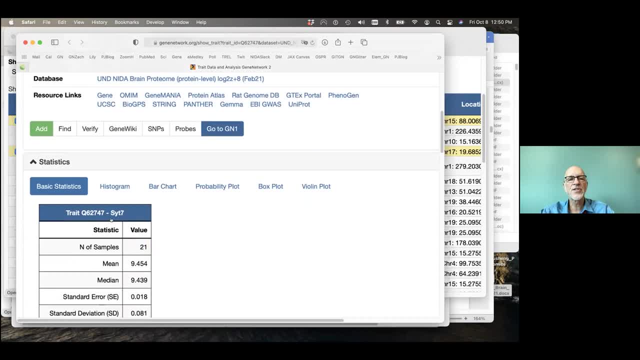 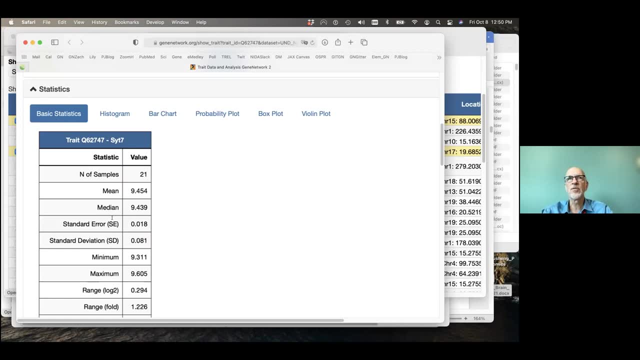 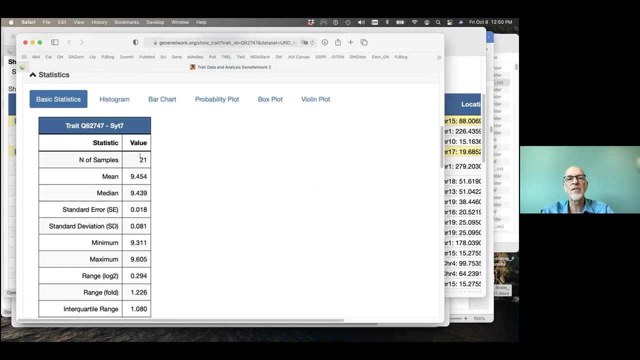 But let's take it anyway. So let's look at the data. So now I'm just giving you a little overview of what we call findable, accessible, interoperable, replicable, robust. what have you So? fair data: 21 strains that Xu Sheng told you about in the second half of this talk. 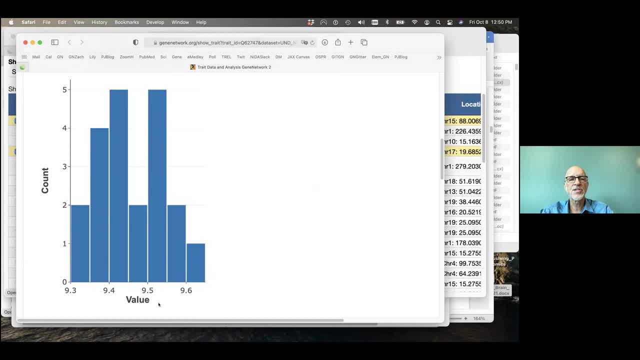 Histogram of the distribution. You'll notice the counts are still low, right? We only have 21 cases here. If this were based on 200 cases, we would talk about a bimodal distribution. We can't do that here, So this is just a sampling artifact, probably the way the histogram was. 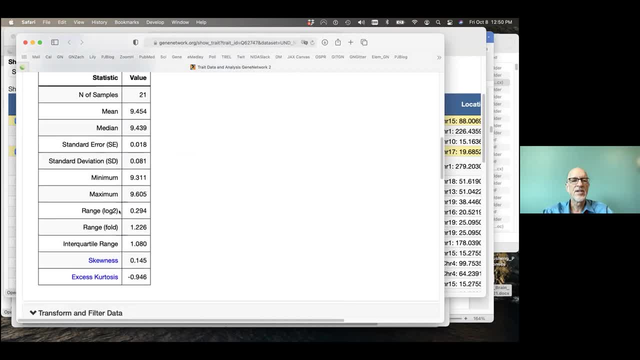 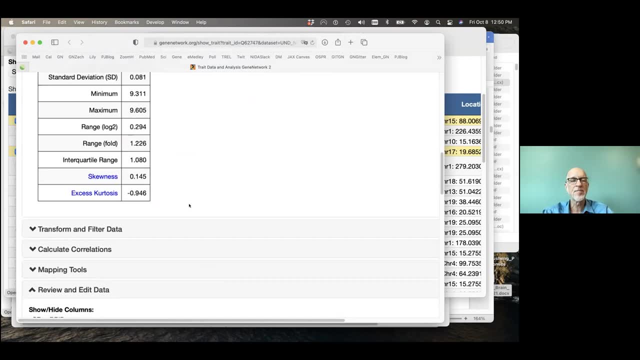 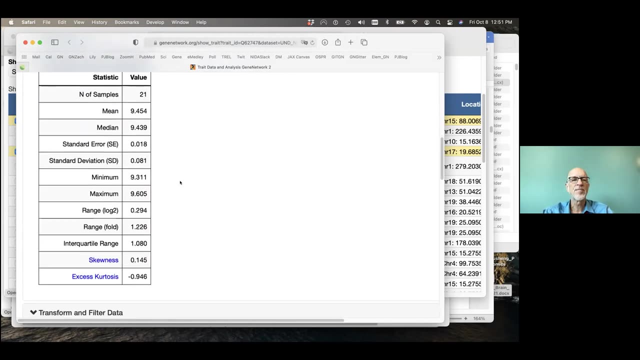 constructed. But we can ask: what is the skewness? What is the kurtosis? Is it sharper than expected or flatter than expected? Is it skewed in one direction or another? It is a little bit flatter than expected for normal distribution, So that's kind of an interesting finding. Let's look at the 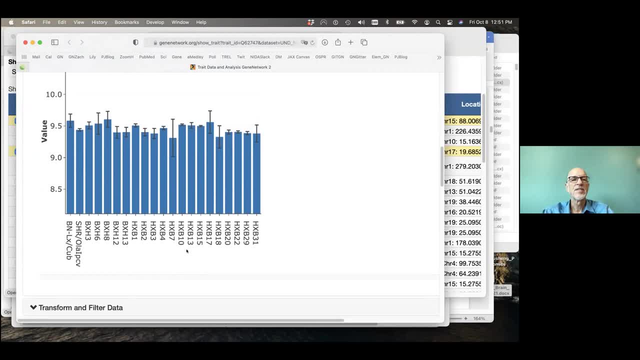 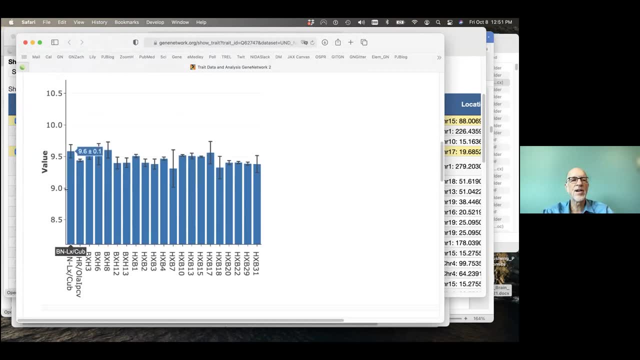 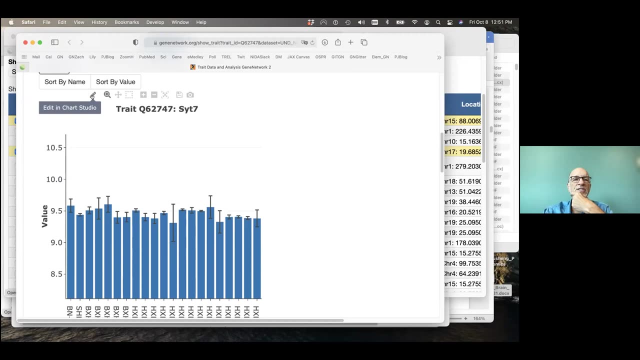 bar charts for the 21 strains. So there they are. This isn't even going down to zero. So this is a fairly small difference. Notice that we're truncated here at a value of eight, If you put this, if you click on this. 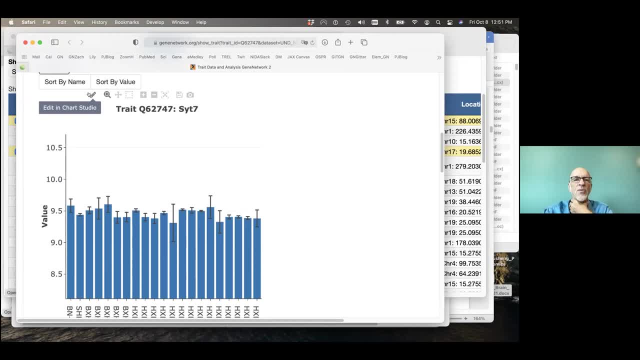 edit in Chart Studio. you can change this figure any way you see fit. It'll open up the data in Chart Studio totally free of charge. It lets you do some cool things. You can see that two of the strains are pretty noisy. Maybe you can't see them. So this is a fairly small difference. 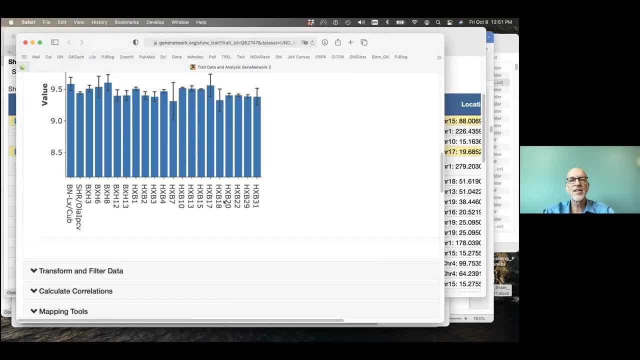 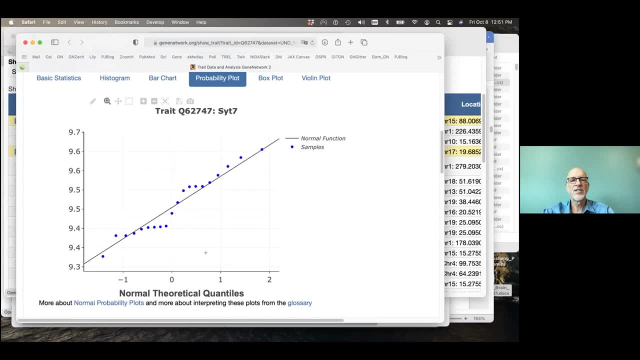 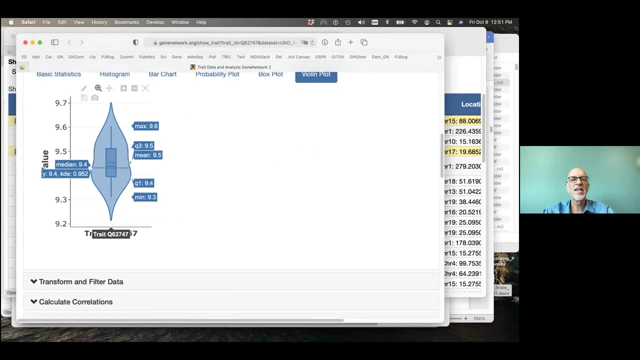 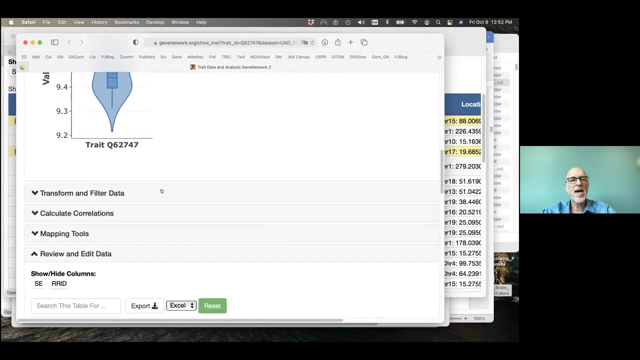 Maybe three strains, But in general that is not terrible data. You can look at the probability plot and you'll see that little jump there that we noticed in the histogram. And let's look at it as a violin plot- Again a little bit broad, So let's map it. So we know that this maps well. 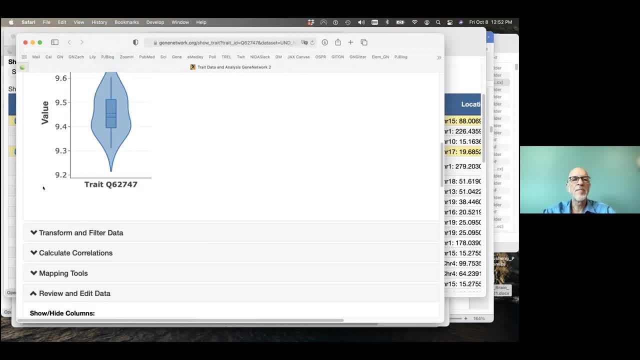 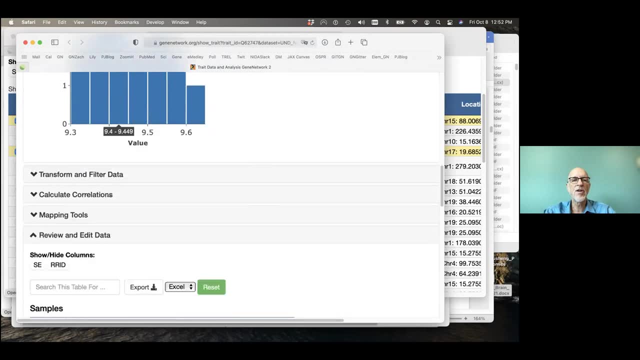 because that's pretty much why we picked it. It does not have any blatant outliers we have to fix. So I'm not going to do anything to the distribution, although I could. So there are all kinds of options here for fiddling with the data. 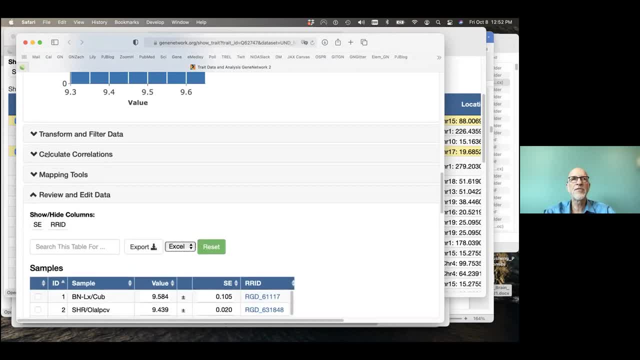 And you should fiddle with the data. Do not be afraid to fiddle with the data. It's really important in some cases. If you don't fiddle with the data, there's a very real risk that your mapping will go astray. So please be bold and do not consider the data. 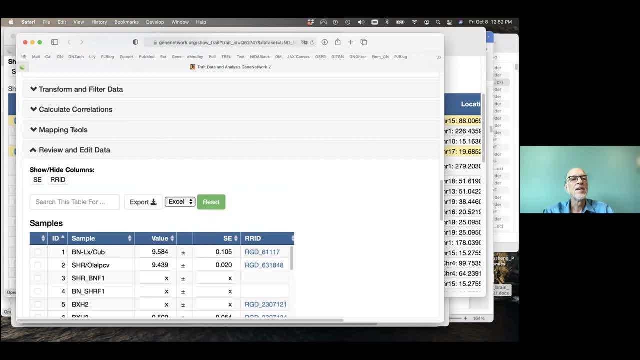 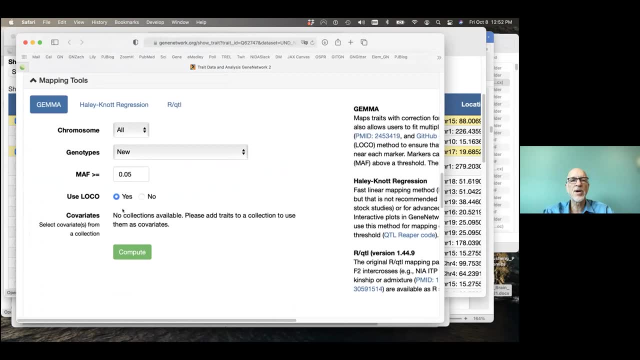 sacrificial. It's not sacrosanct. It's not sacrosanct. We're going to go to mapping tools and I'm going to map this with a linear mixed model. that is quite powerful, But you could map this with RQTL1,. 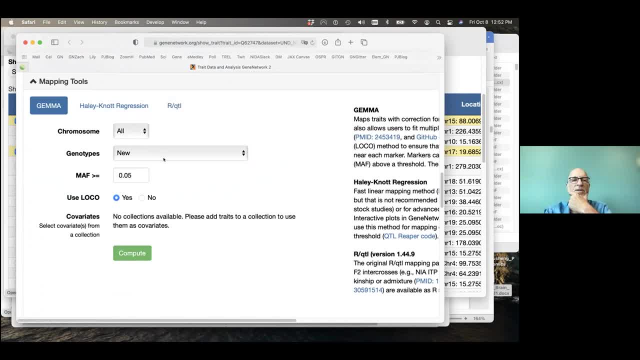 RQTL2, Haley-Nod, et cetera, But I'm going to map it with this. I'm going to use the super new genotypes that Hao Chen and Hakan Gunterun generated from SQL And I'm going to map this with. 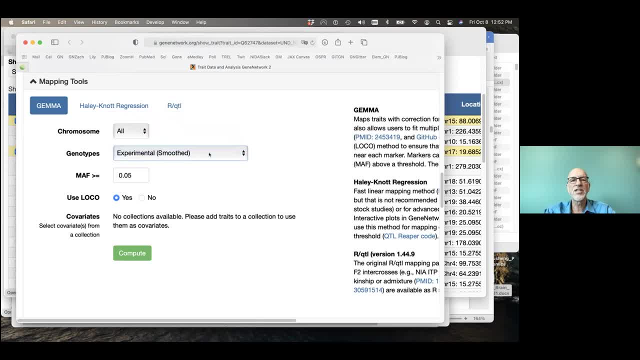 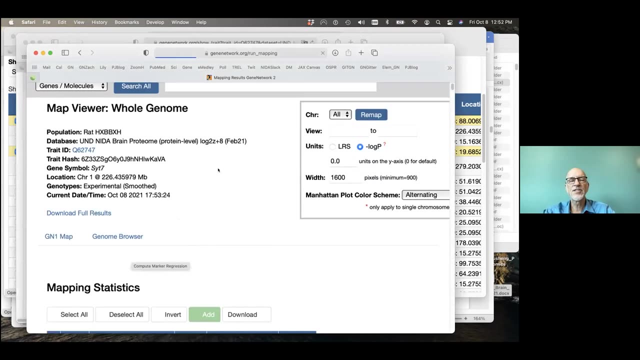 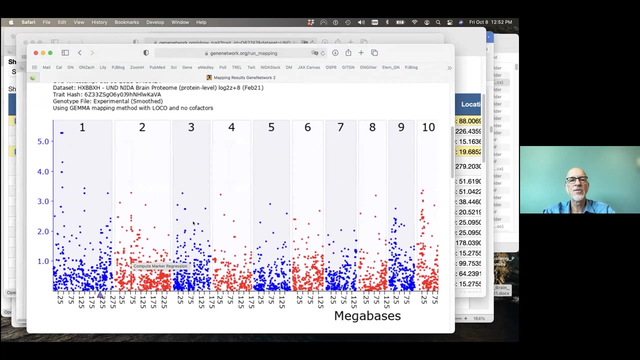 sequence data. It's experimental, but it's actually quite a bit better than our not so new new, So let's map it. It gives you good metadata about what it's doing. It does it so fast that it didn't even update the second, probably because it was cached, And what you see here is our QTL peak on. 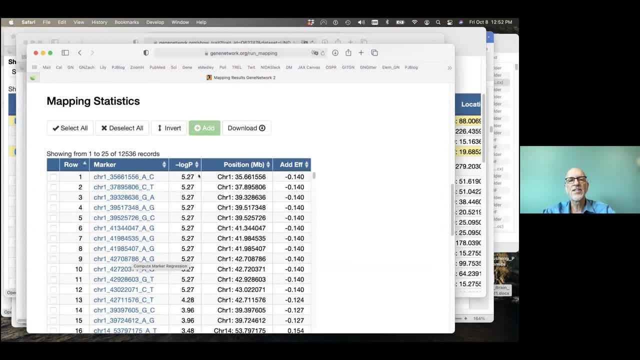 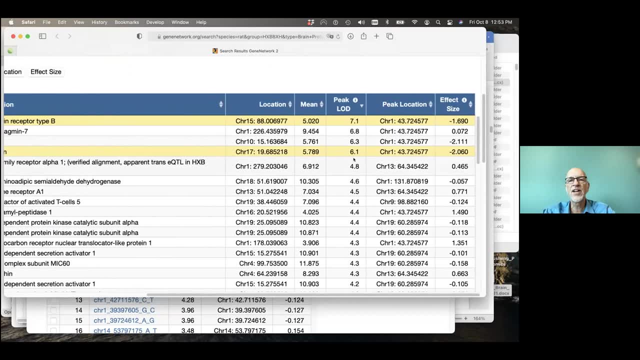 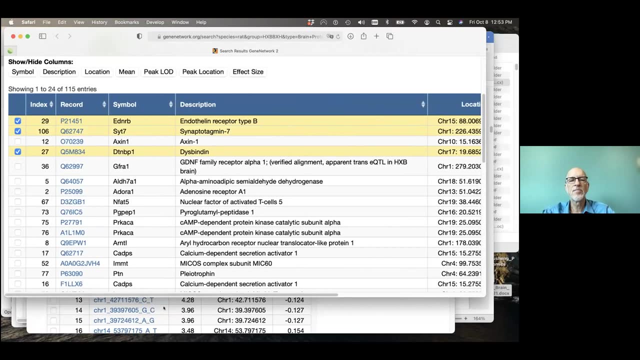 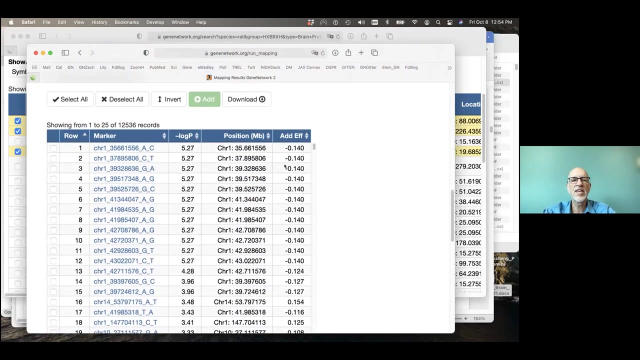 chromosome 1.. at, it's not quite the same value we had in the over here. remember here we had a value of 6.8. this was computed using a different code. we just computed it with gemma, which is a more accurate, better way to map the traits. so the value here isn't exactly the same. 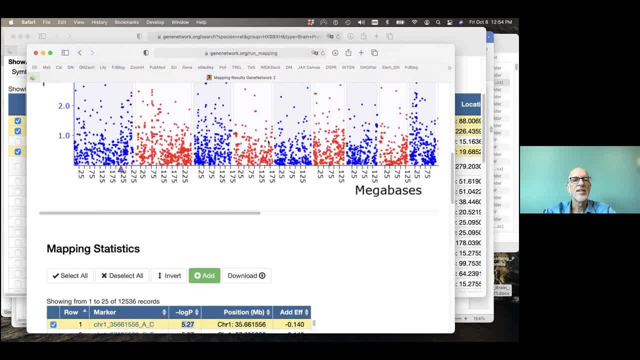 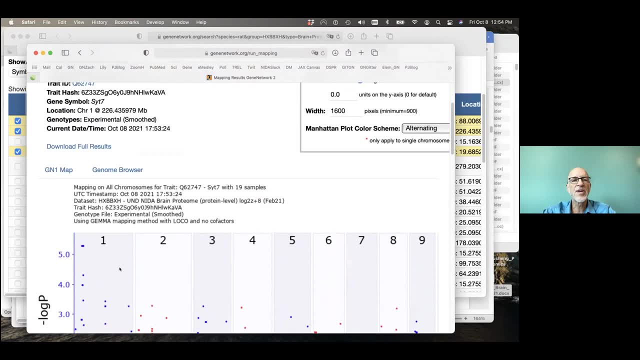 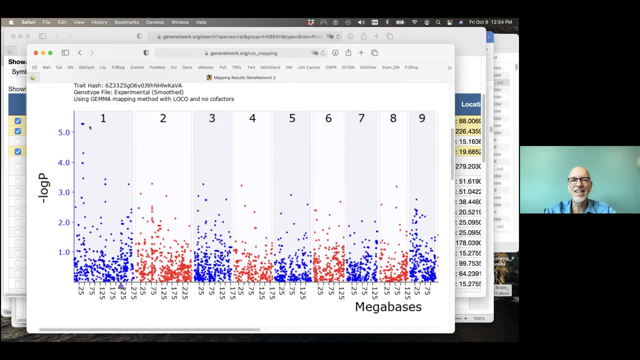 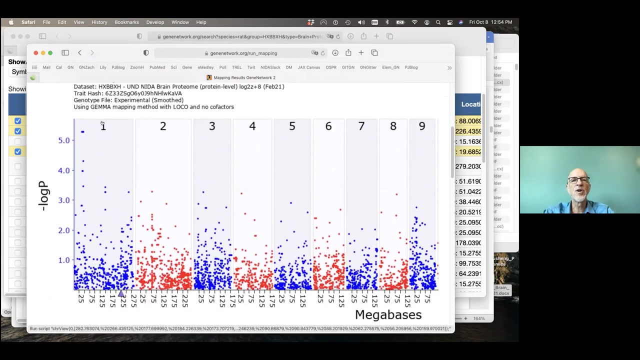 but the location is the same. this is the location. this purple triangle right here shows you the location of synaptotagmin 7. this is the location, the peak way over here. they're not linked at all. they're both on chromosome one, but they're not linked. so let's zoom in to chromosome one, and i have about two more minutes. 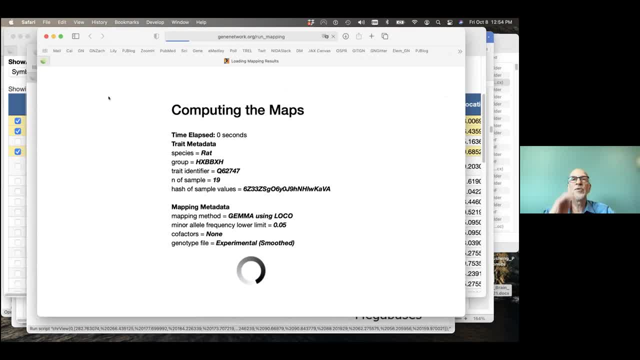 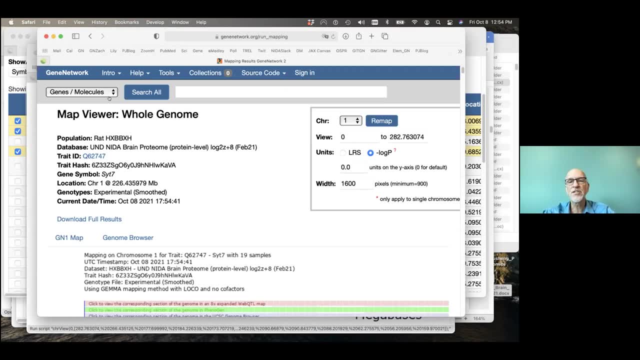 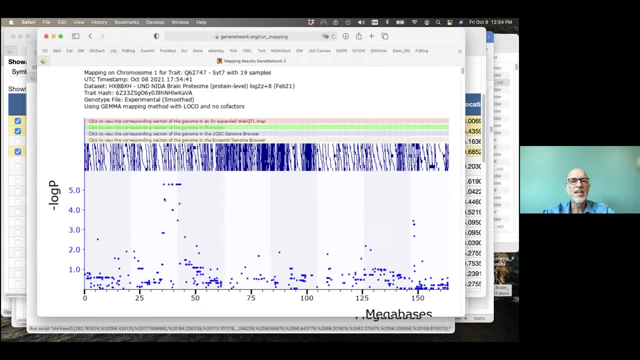 that i can show you how to do this, but i will show you that in this particular case, we have not a good candidate, but an absolutely fantastic candidate. this is: these are all the genes on rat chromosome one. here's our qtl peak. it's not tiny, but it's not. 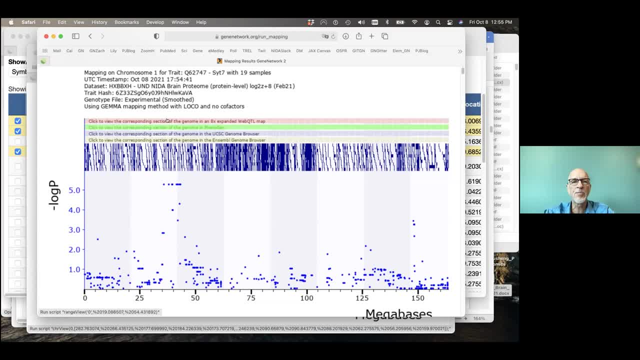 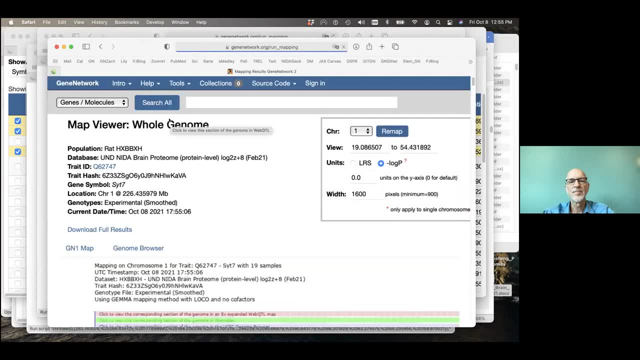 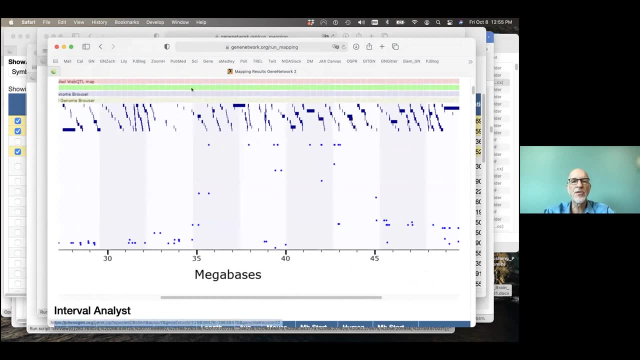 huge. let's zoom on it. i'm going to click right here on this purple or pink area to zoom on it. now we're getting there, so this is our interval. there are about 100 genes there, so we're going from 35 megabases to about 43 megabases. 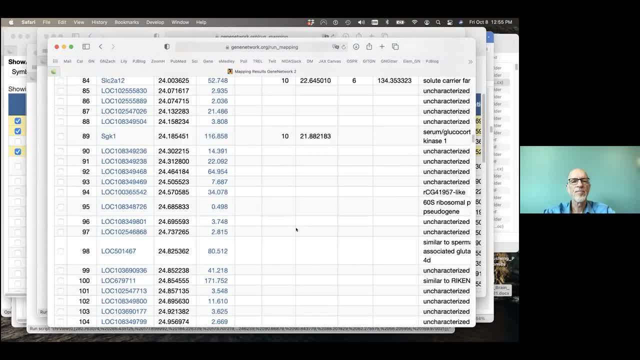 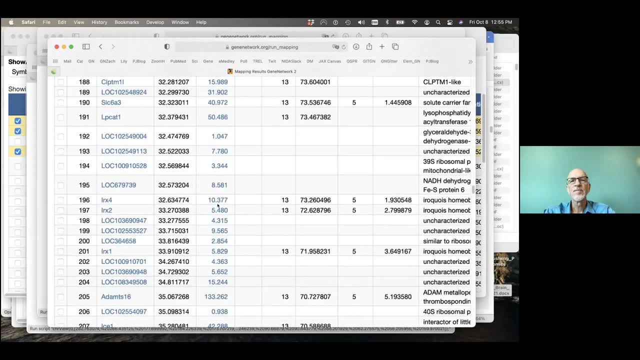 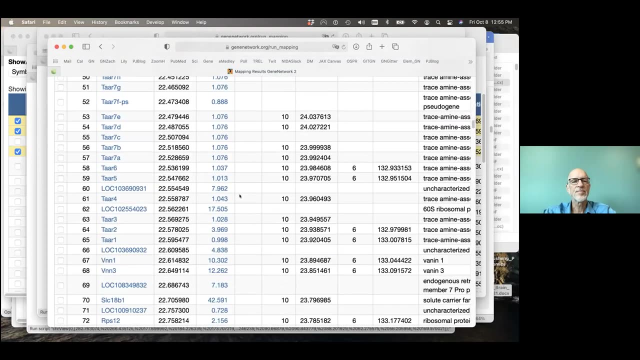 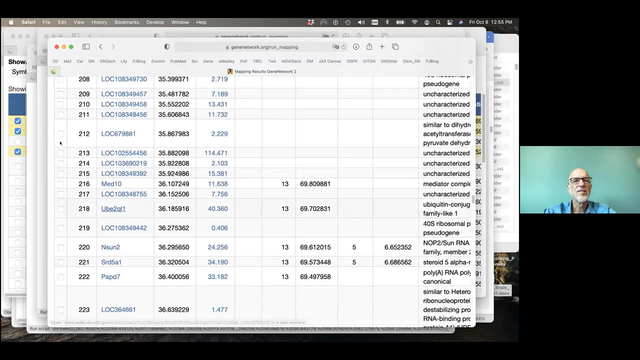 did i say 32 or 35? i said 35. we're only got between 22 and 24 megabases as a first generationavirus. it's not going to need to give and Oczywiście, khaf at the top of the child is 16. 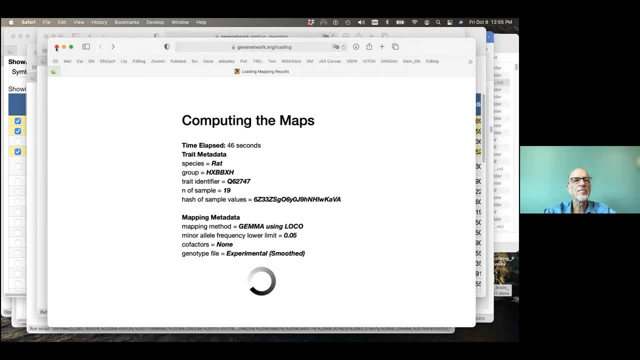 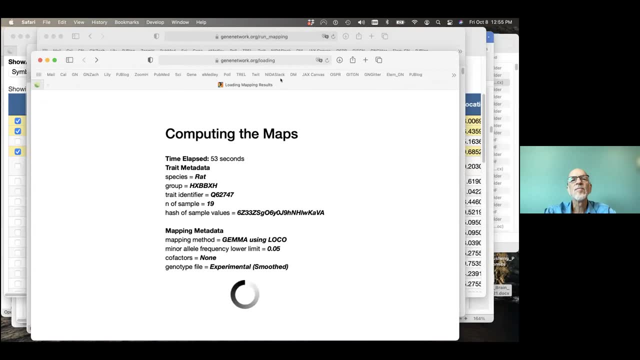 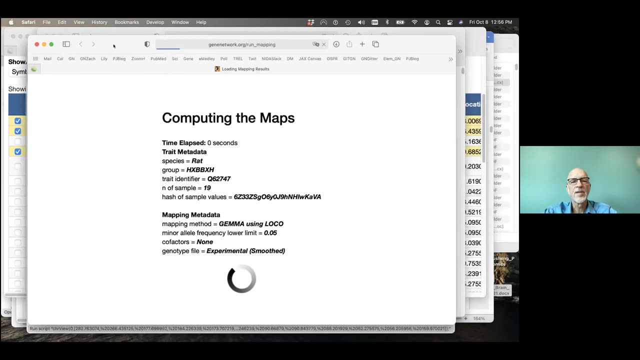 the즘 at the bottom of the DNA. that's how this is going to look to solve for스. we have also three preferences and we're going to bring those, i would say, worldwide on the spring. so let's do this again. sorry, just wurde here alopecia. 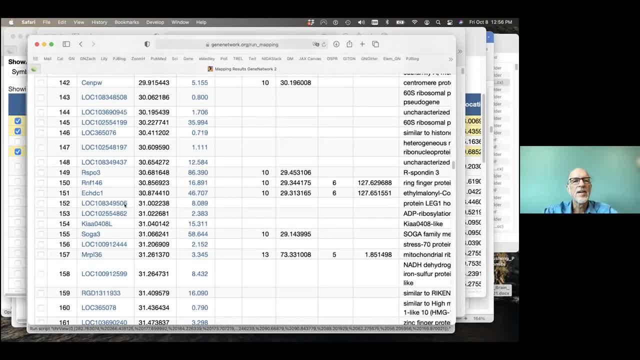 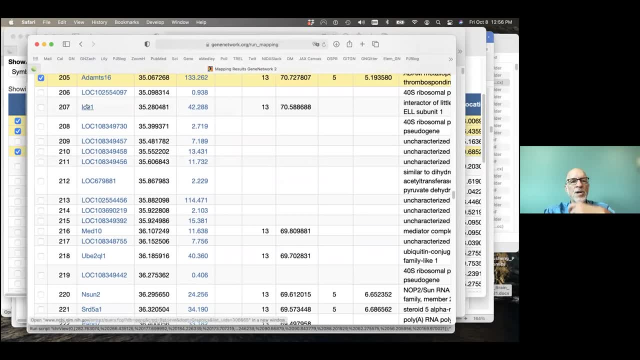 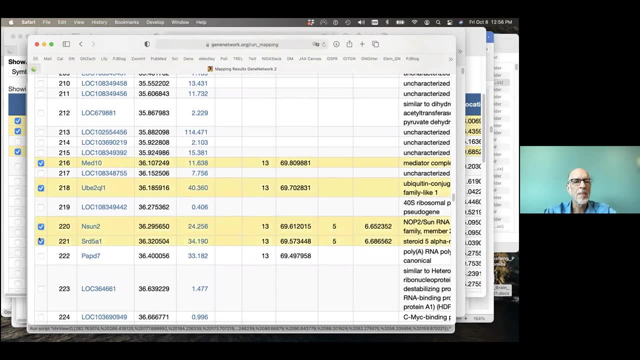 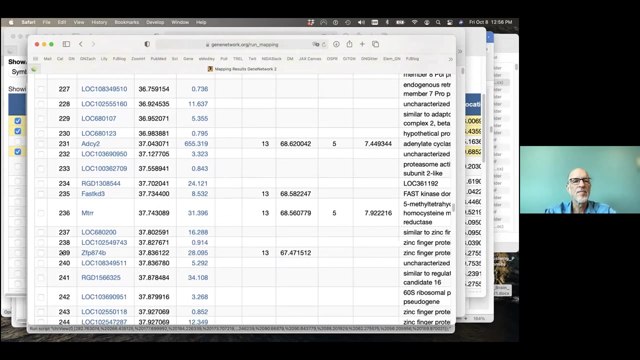 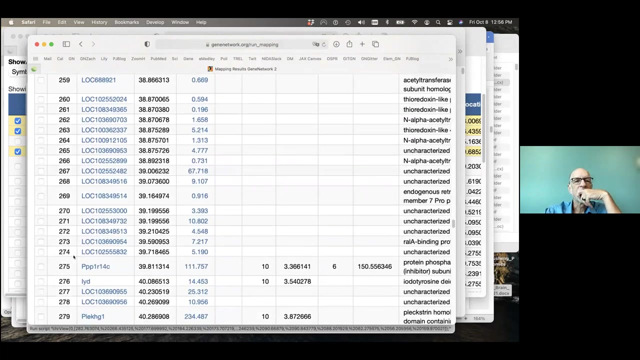 So I want to go to 35 here and I want to start scanning for candidate genes- ICE1.. I'm going to ignore all the unknown, unloved genes that don't have good names. You can see the human equivalent over here on chromosome 5.. 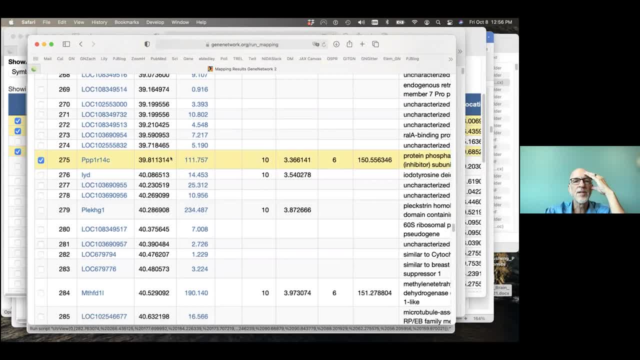 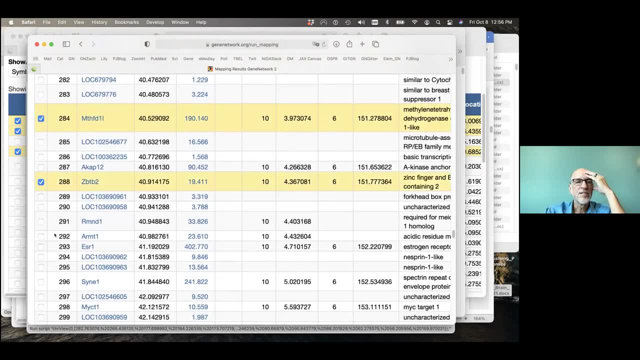 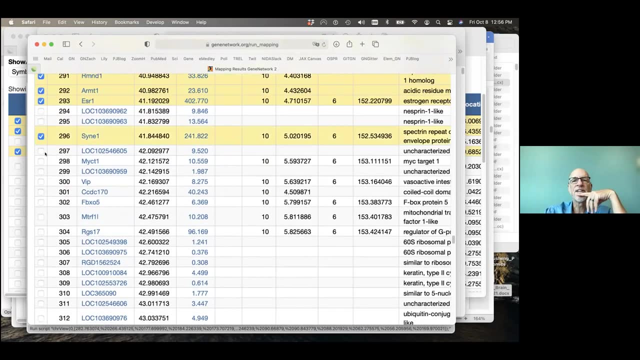 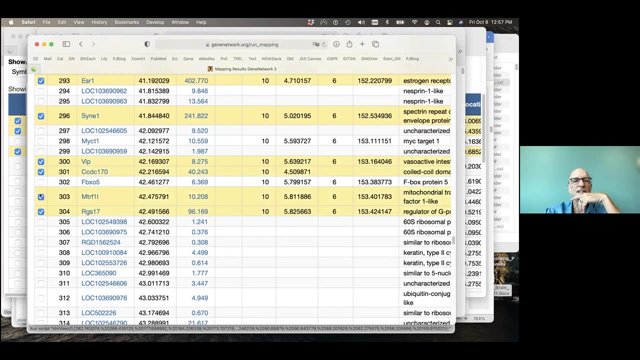 I'm going to skip over some genes. That's obviously interesting. A big gene with lots of variants probably aren't Estrogen receptor- Okay. Another synaptic gene, Vip- cool. this, yes, interesting, okay. End of story. 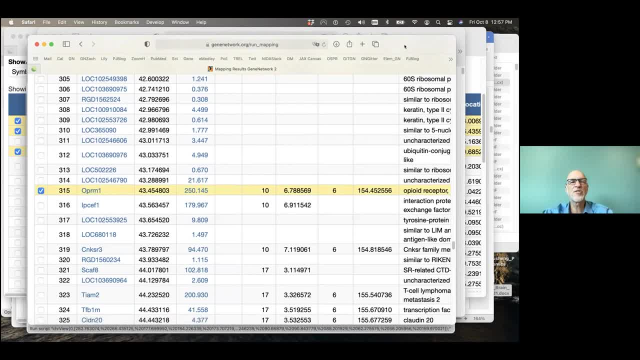 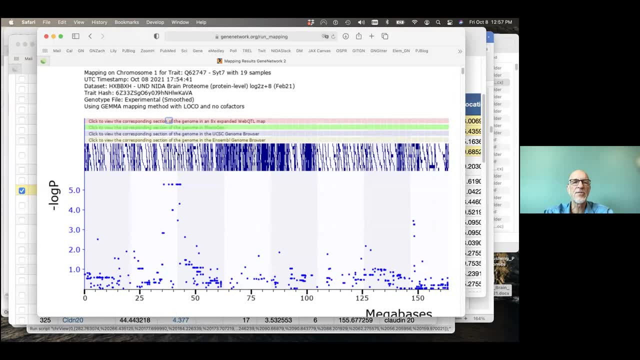 So I mean, it's not literally the end of story, but there's the mu opiate receptor And obviously a huge leap of faith, but the mu opiate receptor is located right here. The mu opiate receptor is, as you'd expect, a ginormous gene. 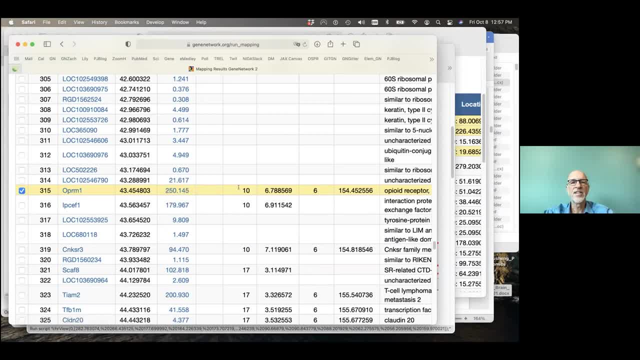 It's 250.. Kilobases And it is something that if you talk to Hao Chen or others, they can actually give you a list of all of the sequence variants in that region. So we cannot pretend that we've cloned the mu opiate receptor as the modulator of these. 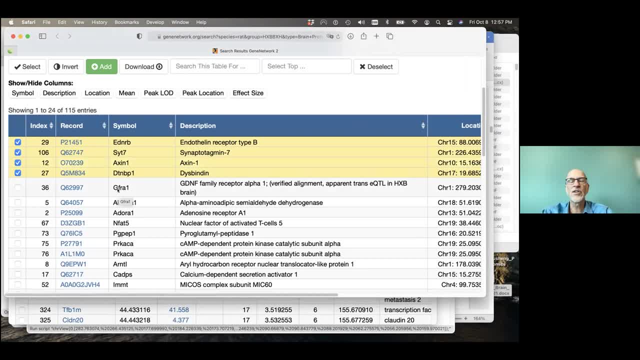 transcripts. but I can definitely tell you that it's a hypothesis, and it's a well-structured hypothesis with a causal basis. And the question is: well, is it really mu opiate receptor if we did a CRISPR-Cas9 and 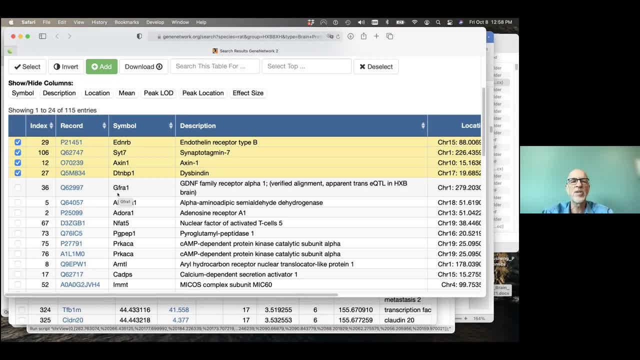 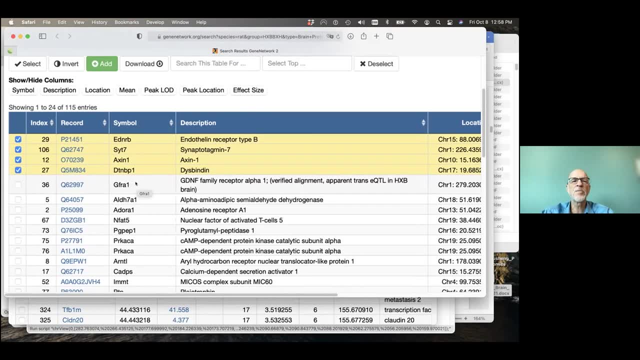 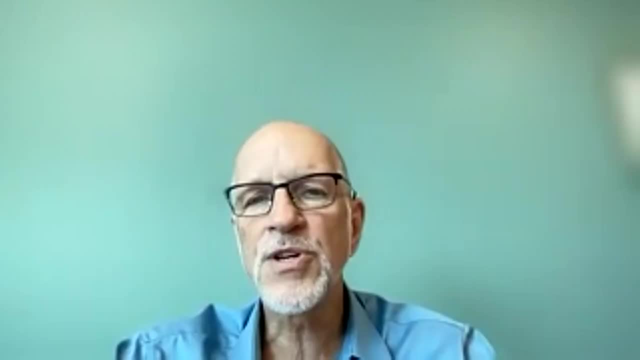 converted a B strain to an H strain or an H to a B. would we see modulation of these transcripts? That's about a two-year project, But there might be some clever bioinformatic ways to avoid that. So I unfortunately have to leave now. 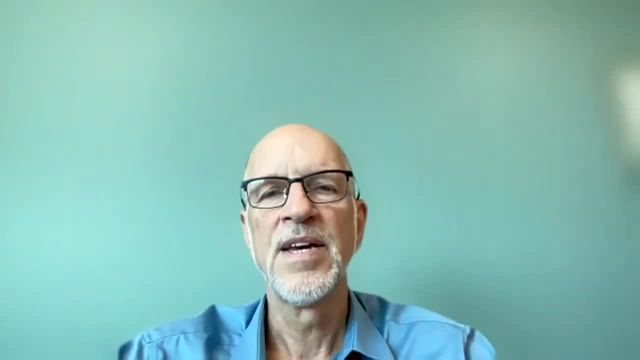 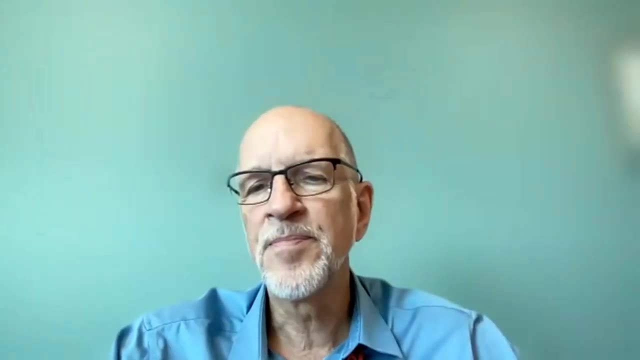 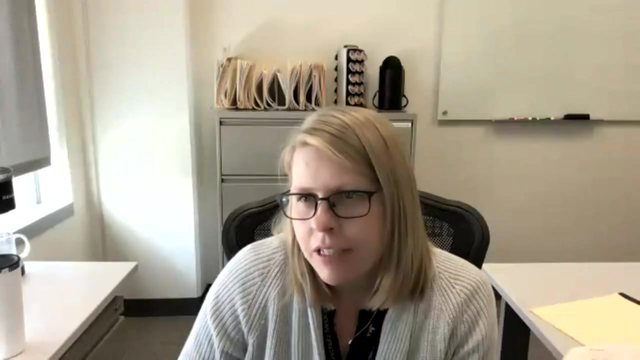 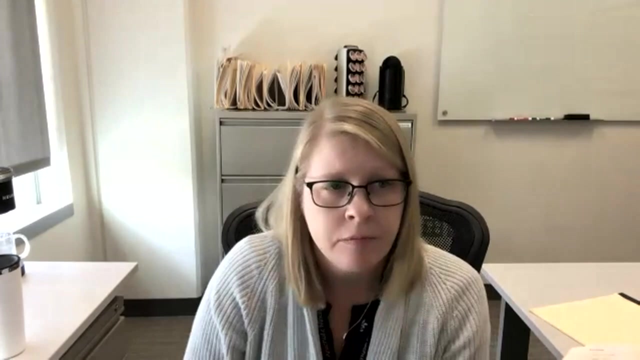 So I'm going to pass it back to you, Xu Sheng, And Thank you everybody. Thank you, Rob. Are there any questions from the audience? I don't see anything in the chat yet. Xu Sheng- great talk. 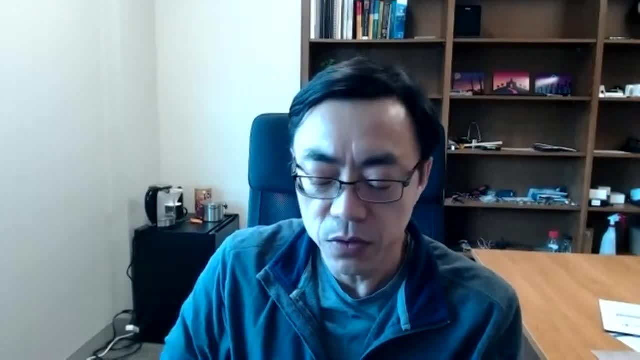 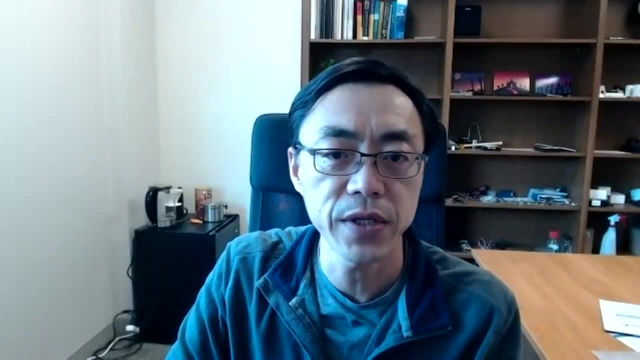 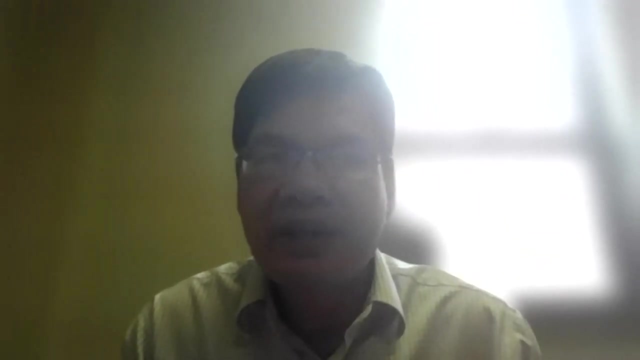 I also have to leave right away, but I'm wondering if I think you have a fantastic pipeline for detecting. I'm sorry, SNPs, Is it possible to detect splicing variants as well? Yes, yes, As long as you curate the splicing variants in the database we were able to. 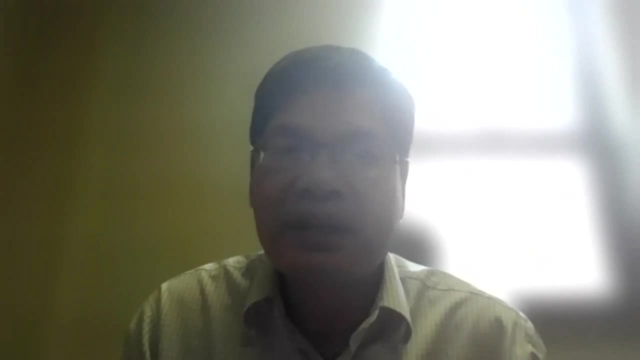 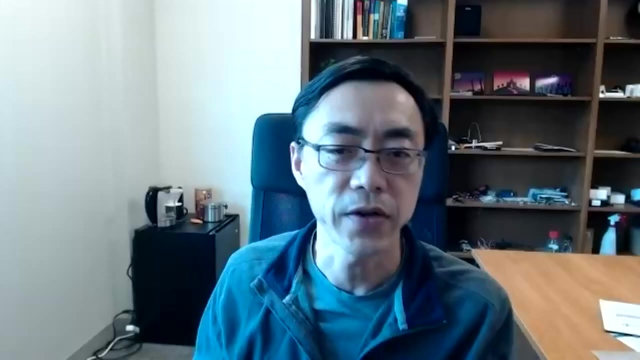 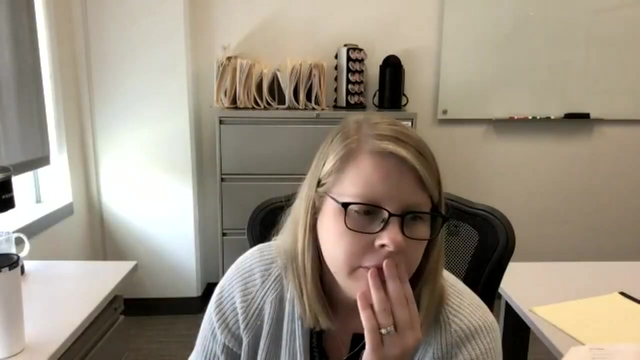 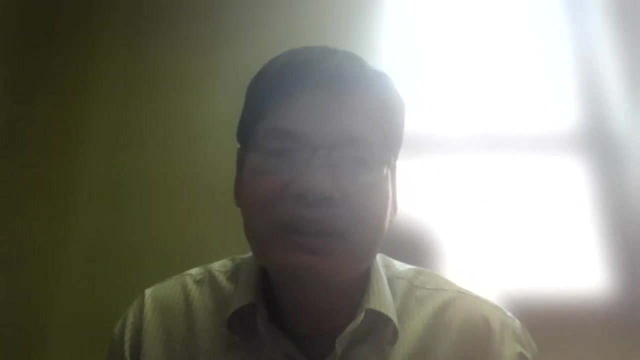 detect whether this splicing variants in the proteome data, Great, okay, Any other questions, Any question about sample preparation or, you know, price or cost or any. I've got a question for Xicheng to kind of get us started here. 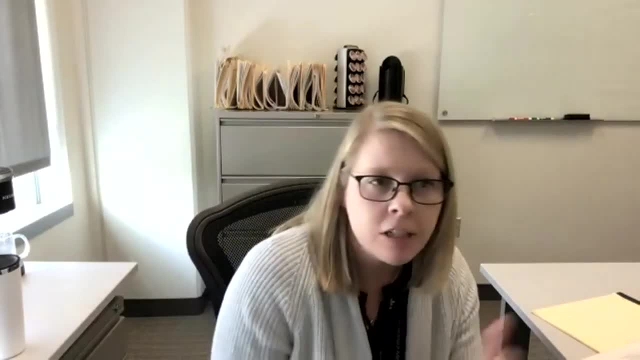 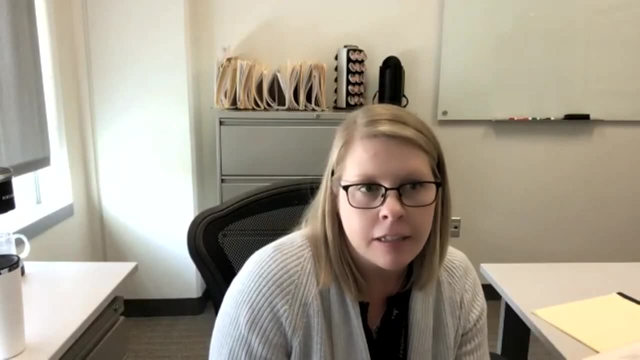 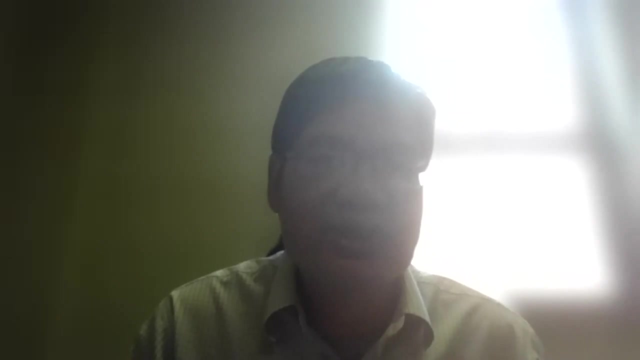 Can you talk a little bit about the batch effect? So when you did this, you did several large groups. Where were your biggest sources of variation? How would you best design the study to do that many samples Right? So batch effect can be contributed by a lot of sources. 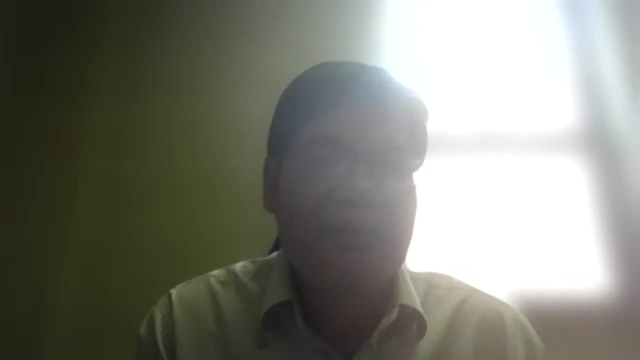 So like if we're doing brain right, human brain for the data, for the data we generate, And there's a bigger batch effect for brain back And they also have a core example: quality And, for example, some of the quality has a broader contamination. 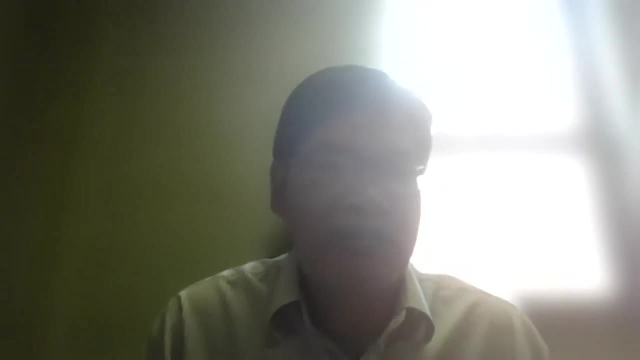 and they clearly show the batch effect. So normally we can correct this batch effect by internal standard. Oh, you know we're using the PC method to correct, And for this 288 examples, we even correct it by the internal standard and we still cannot fully remove all this compounding effect. 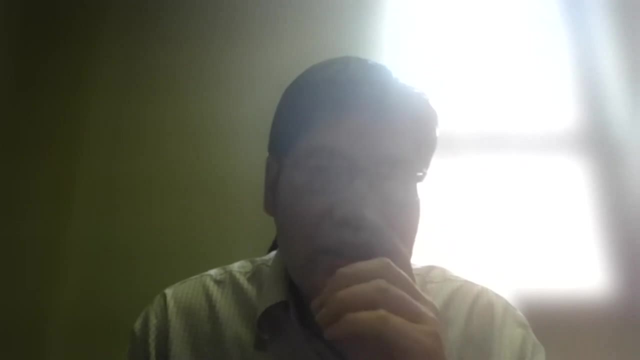 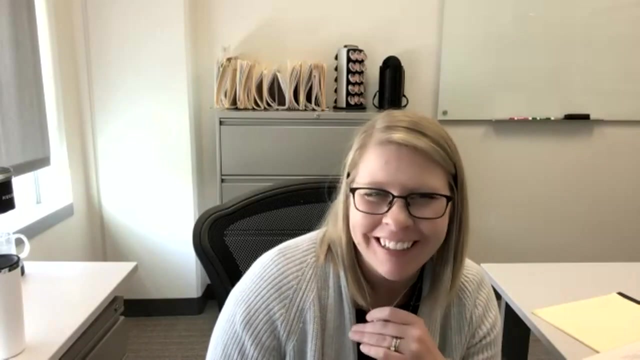 Then we use one other tool called a peer, developed by the Richard Dubin group, And we try to remove all the hidden co-founding effect. After that we get a pretty good mapping result. Any other questions from the group? I've still got a couple more, but I'll leave it open to. 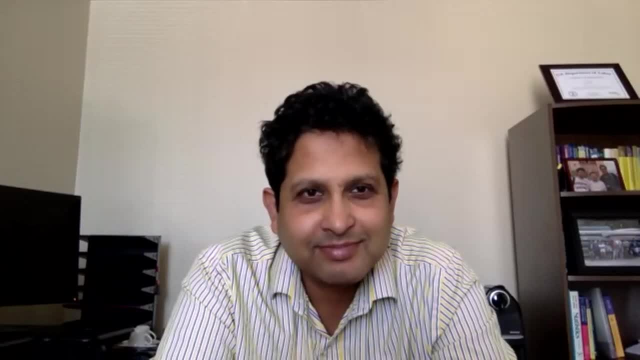 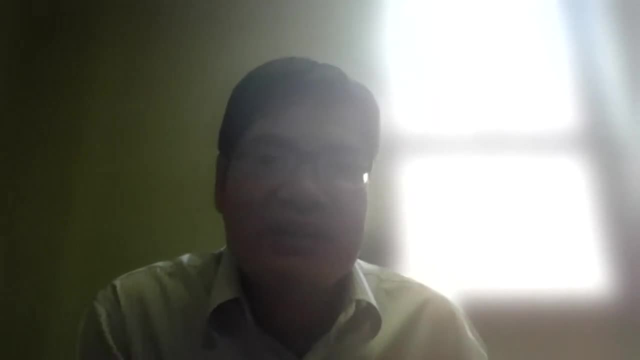 Tell us about the cost. Oh yeah, So, so it's, it's a dependent right. If you want to send your example to the company or you know some service core, and it's roughly five more than $500, per example. 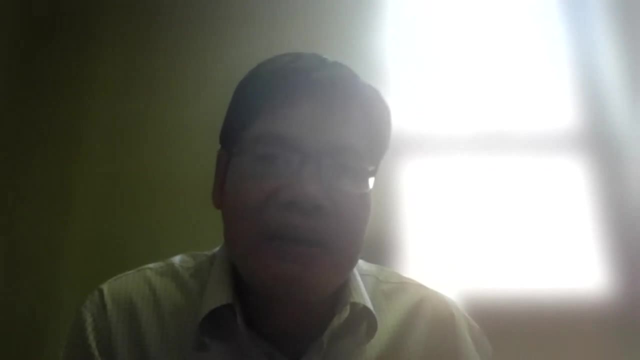 But if you're doing, you know, by our lab, you know if you have a technician or you have a person doing all this experiment, maybe it costs $300.. $300 per example, two to $300 per example, execute, without considering this personnel cost. And it also depends how deep you are going to be. Sometimes, if you want to generate 3,000 or 4,000 proteins and which will, you know, cost much less than you generate the 10,000 proteins, And that's why we are talking about gaps. 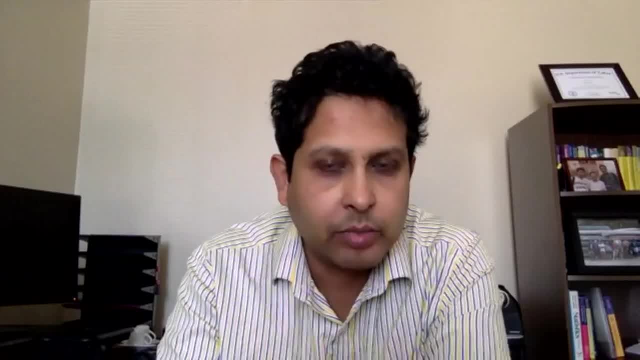 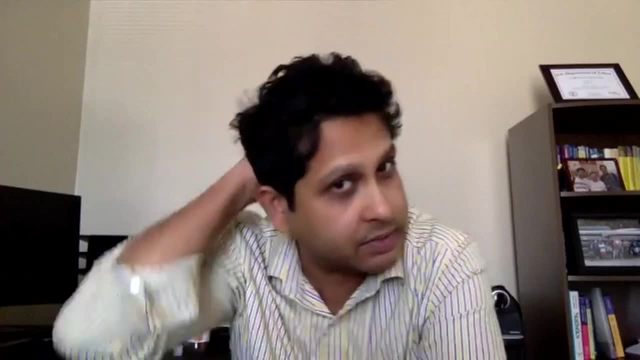 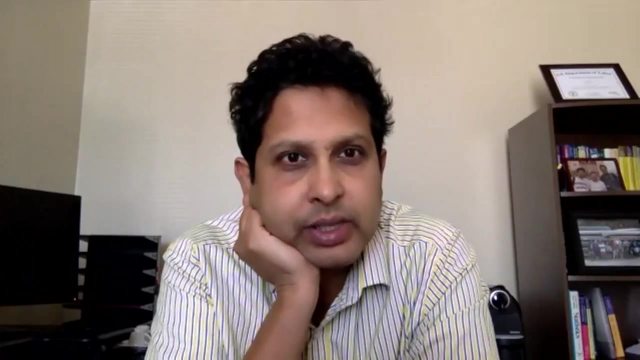 Another question is: you know we had a talk about metabolomics earlier in this webinar series. Metabolomics and proteomics are both using mass spec. How are these? you know what are the similarities and differences in the way you do proteomics. 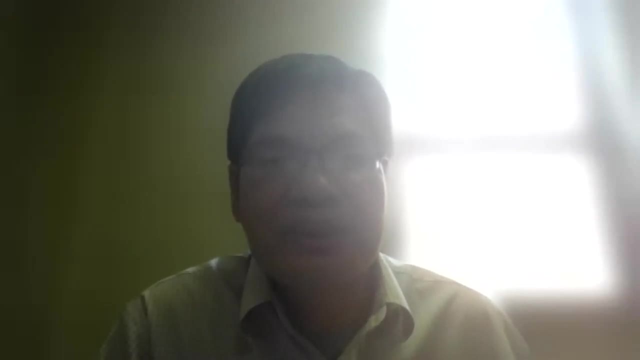 versus metabolomics or libidomics. One is the extracted protein, one is that you have to check the metabolites And I would say proteomics technology is more mature compared to the metabolomics And right now for the metabolomics we cannot do labeling, especially for the human example. 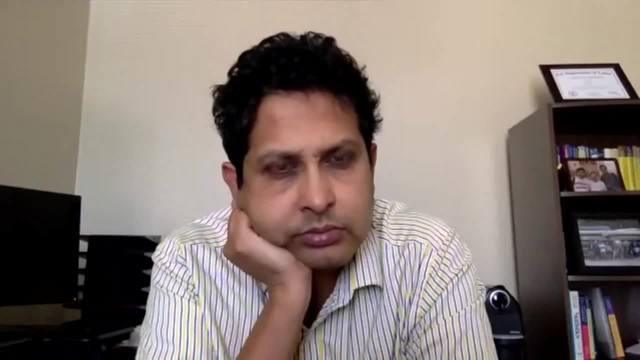 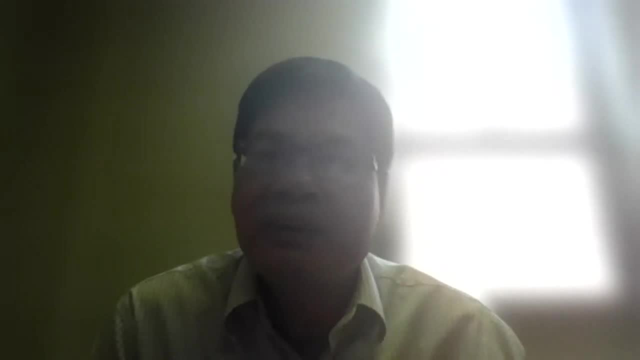 or any other example. So most of the time we only do label-free approach And in the metabolomics field most of the people are still doing target approach And when we say target, you have a standard component first And then you detect this U-example match to the standard to see whether this is a label. 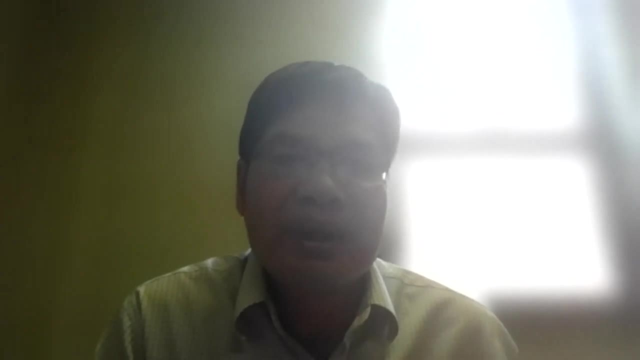 or not. The compounds in your example also match to the standard based upon the mass and the retention time. So I would say proteomics technology is much, much more mature than metabolomics data, And normally you only get a maximum of 500 ID for the metabolomics. 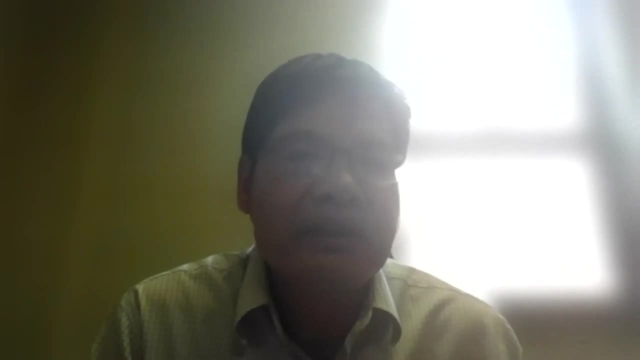 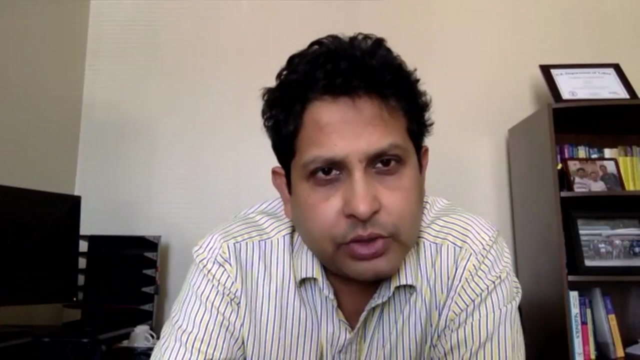 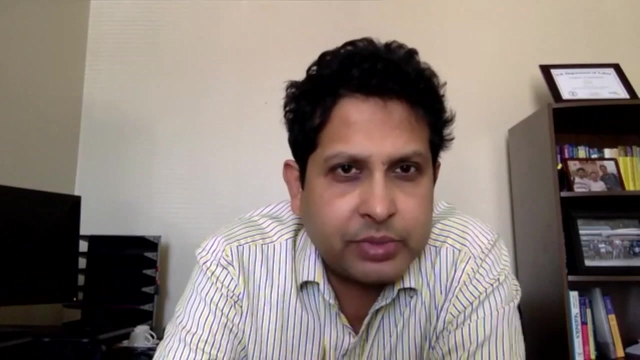 And most people, you only get 200 ID. So in the proteomics, as I understand, there's also this deconvolution step right. You're breaking it into peptides, then reconstructing it. Are they doing the same thing in metabolomics? Metabolomics don't have this issue. Metabolomics just detects the compound And proteomes. because we measure the peptide, we have to break the peptide into a protein, into peptide. So we have to bring back the peptide, So we have to break the peptide into peptide. 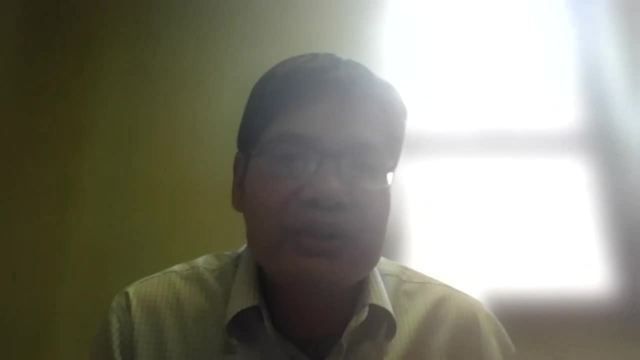 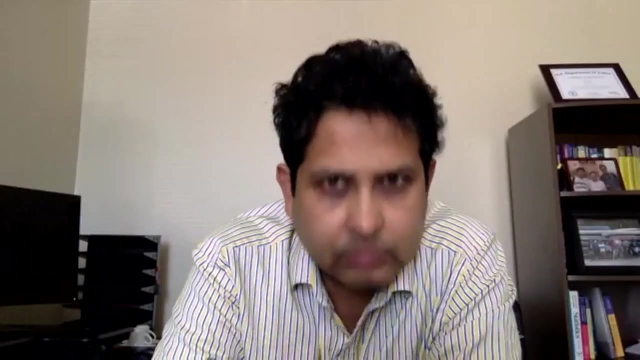 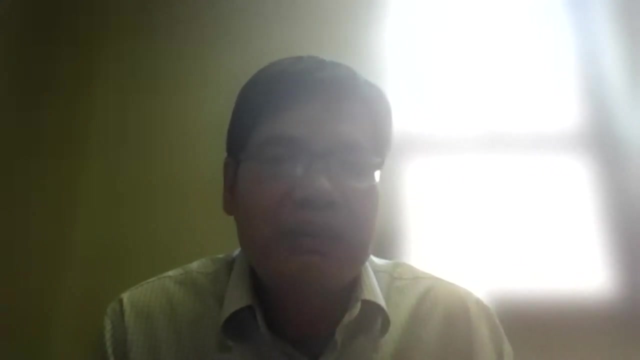 to the protein level And also there are a lot of the shelling And for metabolomics also has, you know, isomer. They share the same mass but different structure of the compound, which is still mass spec, cannot resolve this isomer. If you want to resolve this isomer, 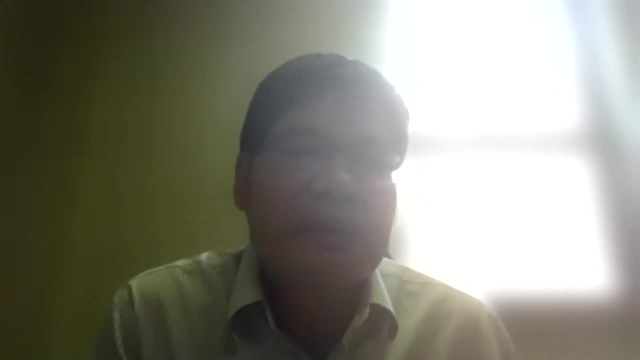 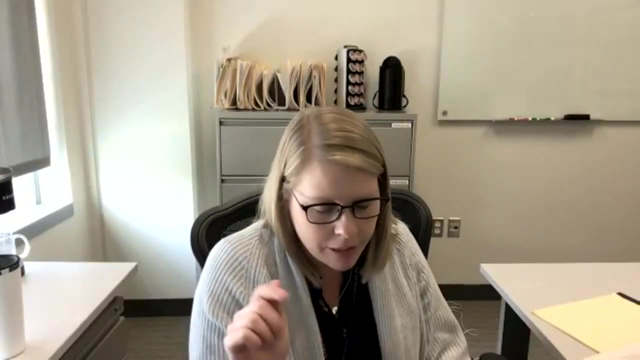 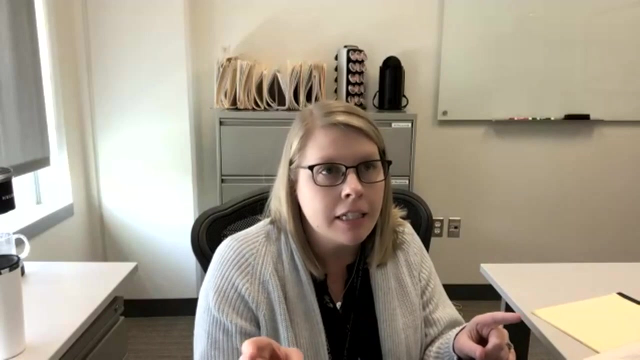 it's bad to using NMR or some other technology. So you know, piggybacking on this idea of going from peptides to proteins, how do you handle it? So you showed that those peptides that have the variant in it and you quantitate. 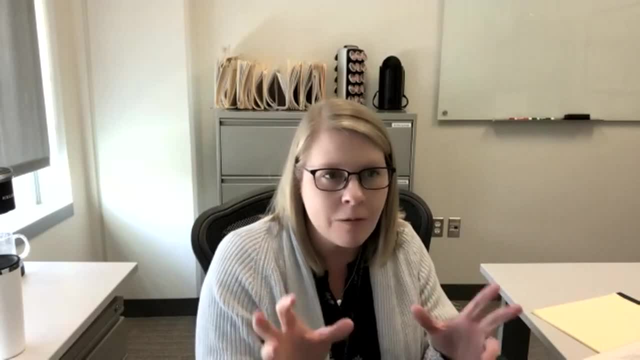 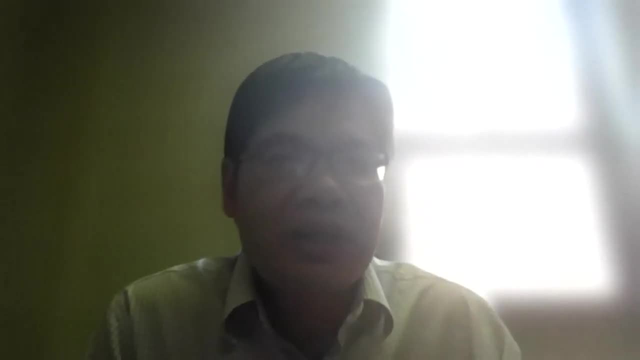 the different variant, you get different values. How do you handle that when you summarize into proteins, Right? So, as I said, we first summarize it at the peptide level, first. right, Because one peptide can be measured multiple times. And then, in order to accurately quantify this protein, we typically only select. 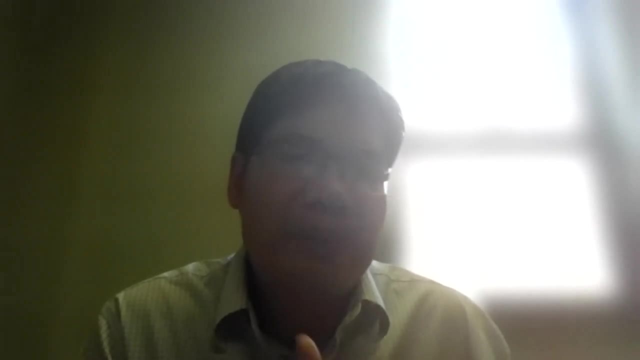 the most reliable quantification for the peptide, For example the top three measurements for each peptide, And then we summarize all this, get an average or median value for peptide. Then we get another median value or average value for the protein. But again there's some issue. 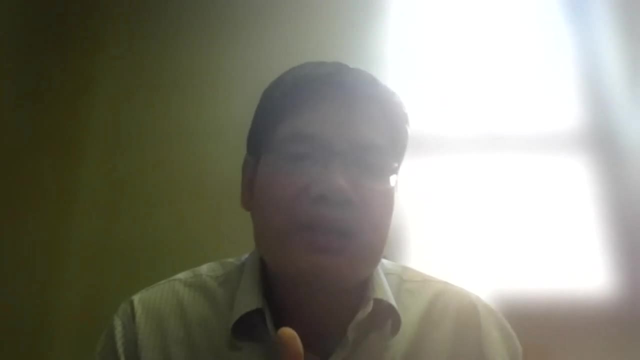 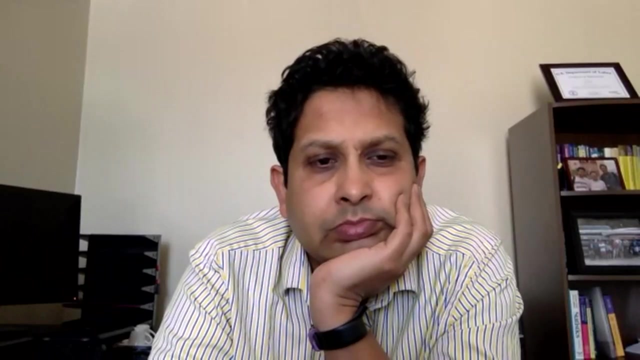 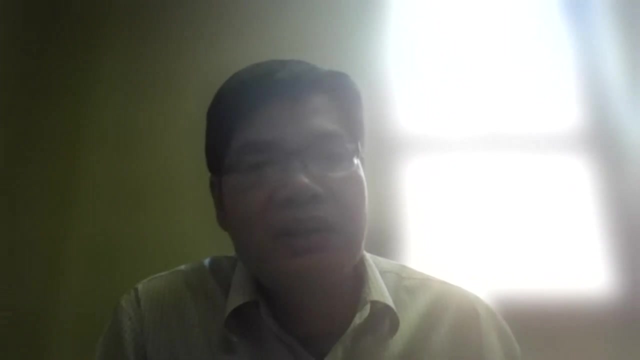 actually in the proteome. This is kind of elephant in the room. So there's a shared peptide, For example. this peptide actually contributed by gene family. It's not contributed by this isoform And so you can use the unique peptide, For example, the unique. 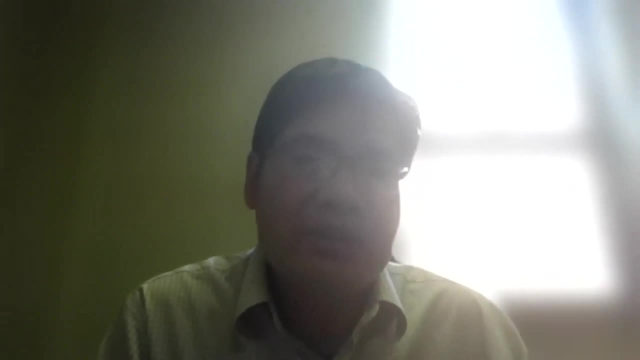 peptide from that isoform And you can say, oh, this expression is represented, this. But right now people just roughly summarize all the peptide together to represent the protein. So right now we still call the protein group, not the protein, really protein isoform. 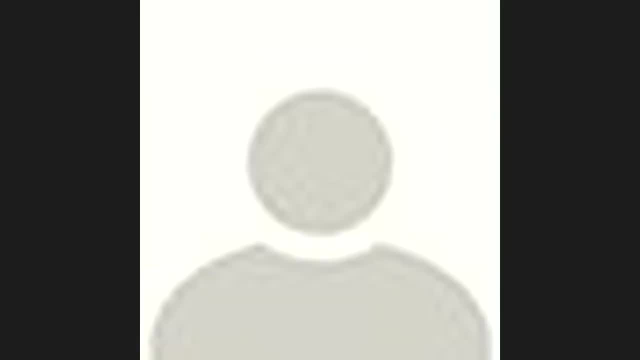 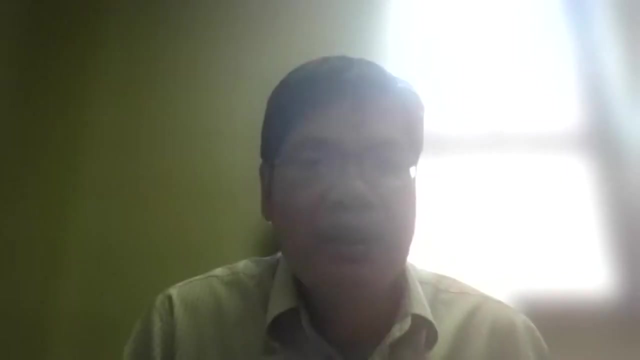 Shu-Sheng, I missed your entry point for the mislabeled. Did you have genotype data and the proteome data from these people? I missed the point about mislabeling. If you did, then I understand. Yeah, For this data set. we generated all the whole genome sequencing, RNA sequencing. 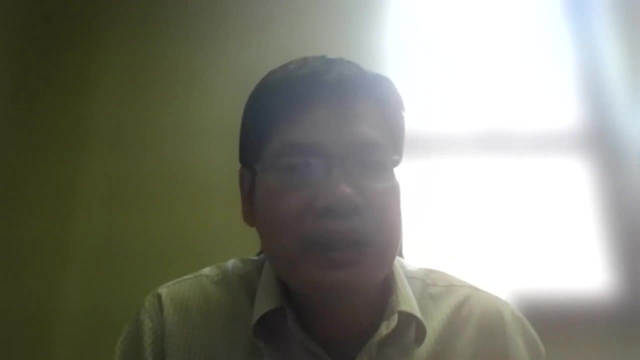 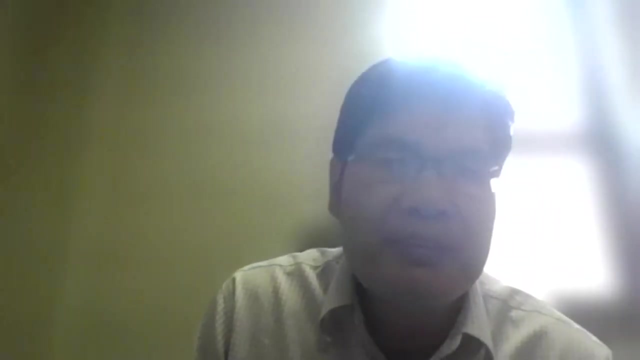 ETAF-seq, riboseq and proteome data. So we also observed mislabeling in different data set And then we do the independent correction for the ETAF-seq and riboseq And better. We also do use our approach to crack the most rapid date. 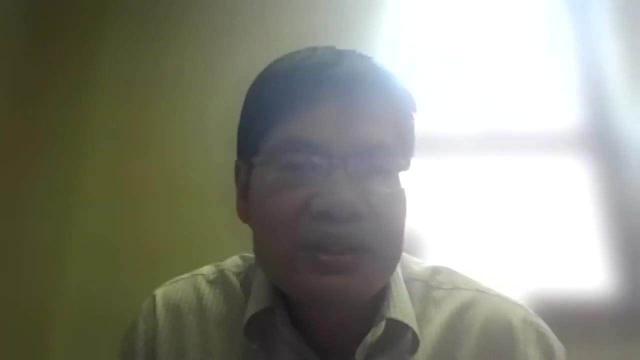 OK, got it, Thank you. So, by the way, class, we recently generated a proteome data for BRCA6 and D2 after seminar infection. I think this is a pretty good idea, But I would like to see the project data, okay. 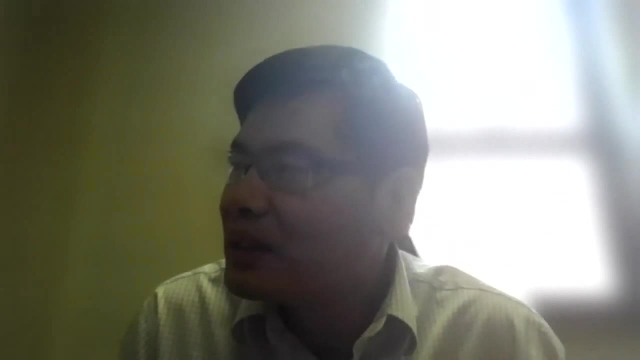 I think maybe I can share the data with you. but this is a data we generated in the UND but it's not very deep, only about 4,000 protein. But I just kind of saw that you might interesting in this data set as well. 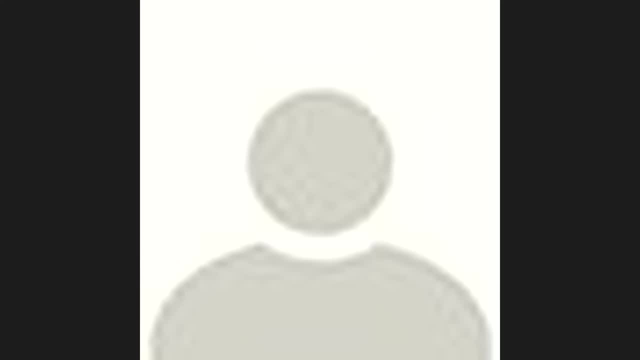 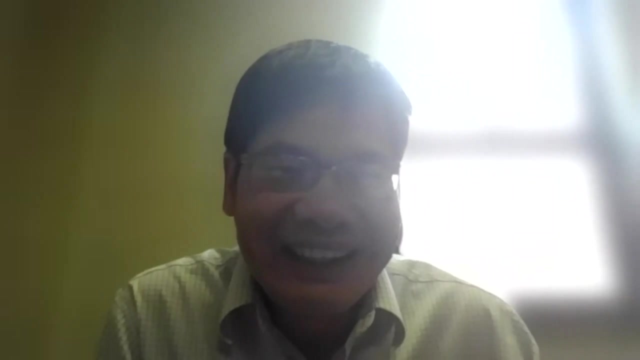 Yeah, we have some. so black six DBA2 comparisons. we have quite a bit for the lung. I guess it's the lung that you're talking about. We get it from the spring. All right, that is yeah, okay. 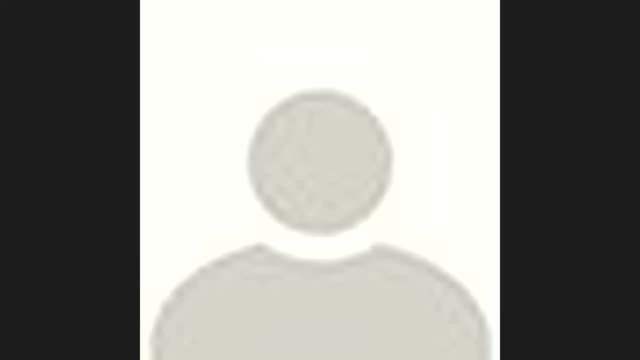 I've never done. unfortunately, I probably don't have the samples anymore. We always do the lung for okay, What kind of infection? I have to ask first. maybe It's a salmonella infection. Oh, yeah, okay, okay. 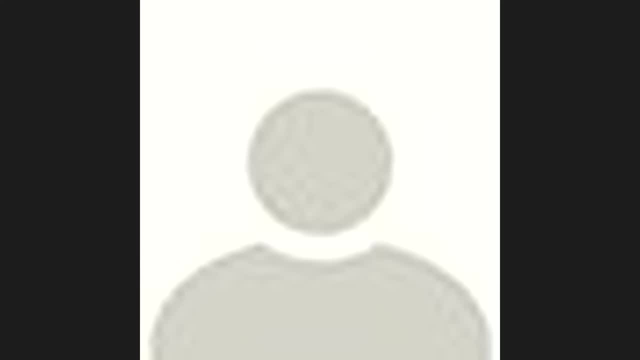 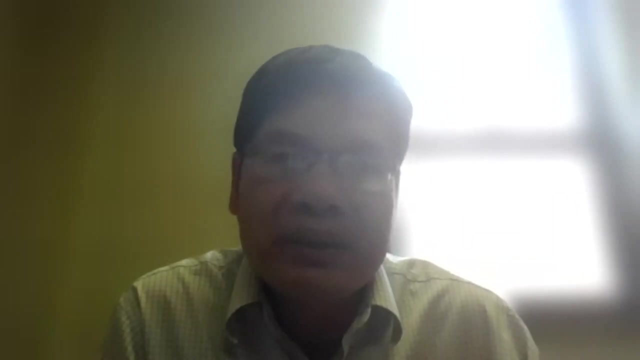 So I have flu and lung data and we do have transcriptomes of the lung and of the blood. Yeah, okay, yeah, different data. Yeah, our next experiment we'll do infection using salmonella. do the infection for AD mouse model? 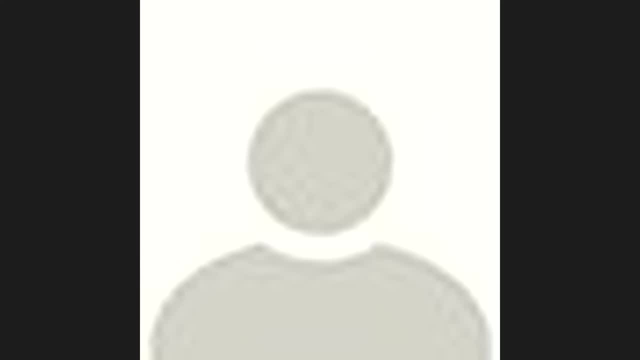 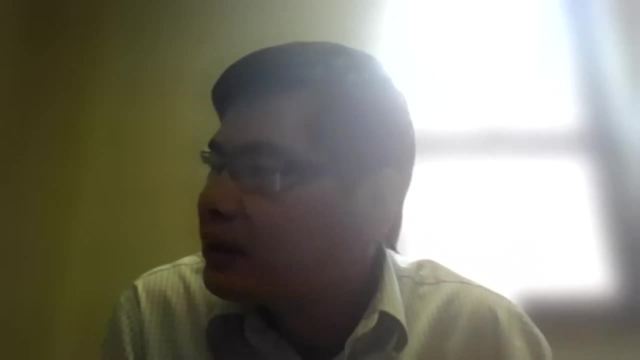 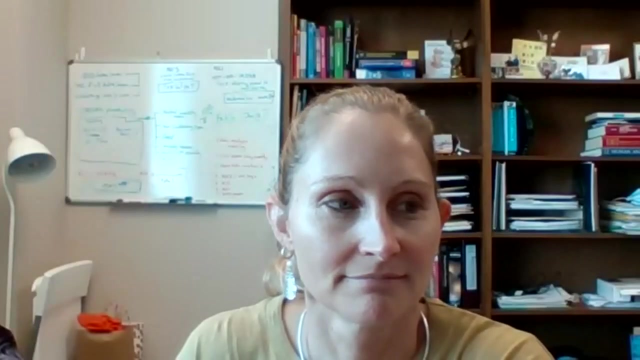 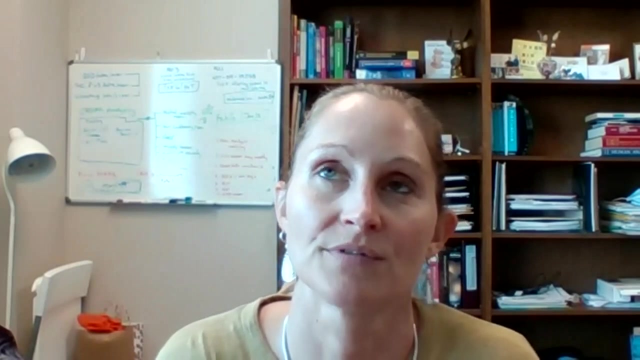 and the black six mouse model black six mice, And then we will do the proteome profiling of the infection as well. Okay, sounds interesting. Excellent, I had a quick question if there's time. I was just curious about I think you detected between like 8,000, 9,000 proteins. across your batches and you were using the whole brain? I think So. would that number change if you looked at like a region or cell type or what's determining that number of proteins? The number largely depend on how deep of your fractionation. 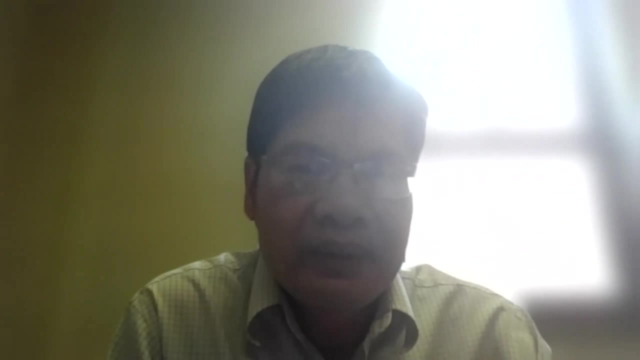 It's not depend on the brain region. Anyway, any brain region has more than 10,000 genes or proteins. So if we go to deeper enough profiling and we should be able to detect the larger amount of protein, I would say it's really depend on how deep you are going to be. 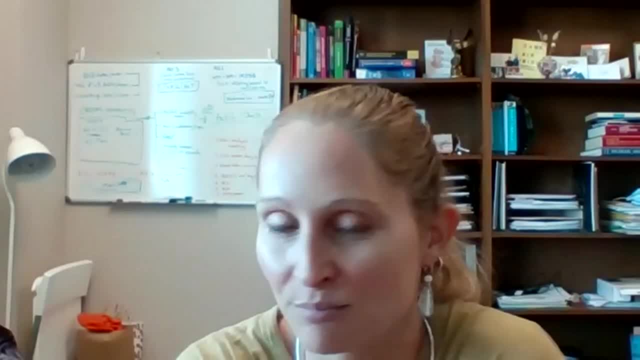 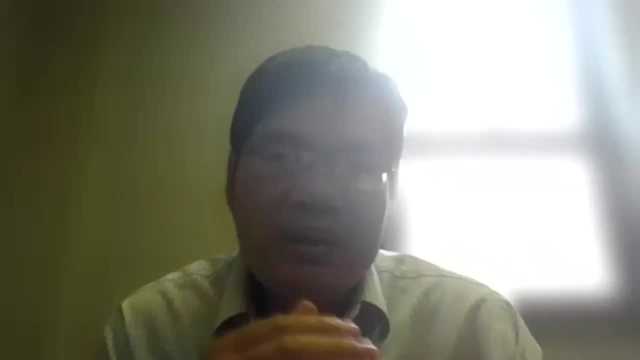 Do you have a sense for sort of the upper limit right now of protein detection? We would say for our paper: this is the deepest protein we ever getting And this is a 14,000 protein from cortex. Okay, Thank you, That's awesome. 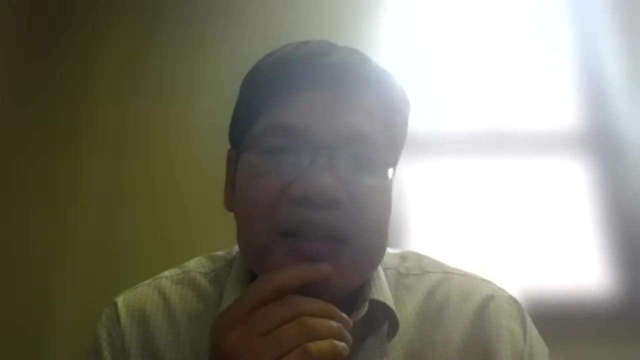 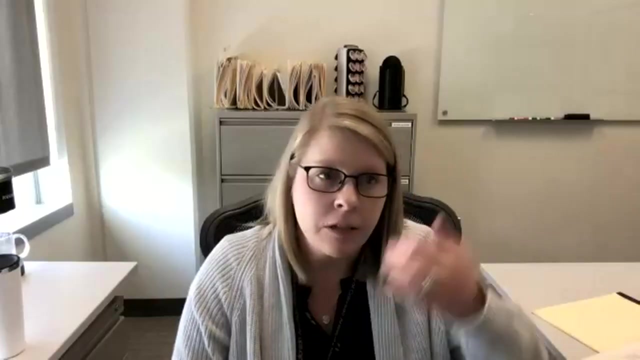 And for the phosphorylation we get the deepest data is the 100,000 phosphorylation site. One of the things I was struck by Xu-Sheng was the number of trans-EQTLs compared to the number of cis-EQTLs. 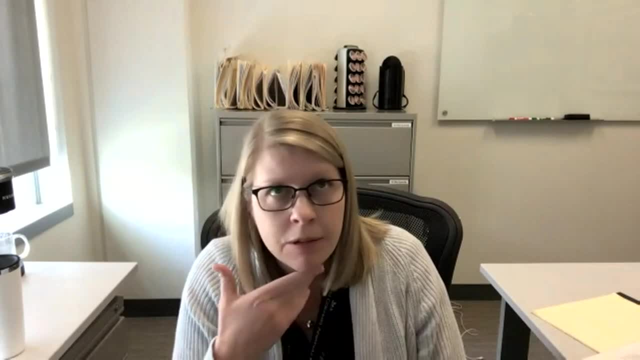 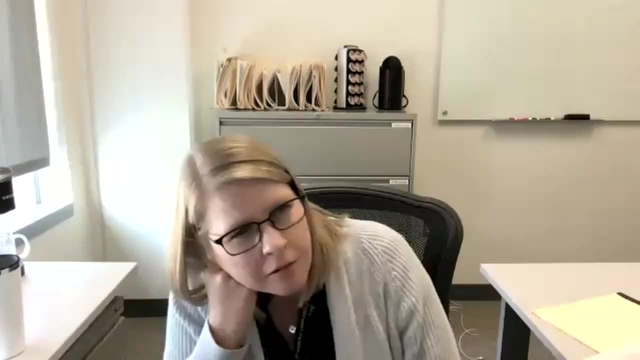 that you found in the rat. Did you do a? did you do a similar protein QTL study in the human data that you had? Yeah, we do, we do. Did you see that same ratio of trans to cis? Well, we get for the human.